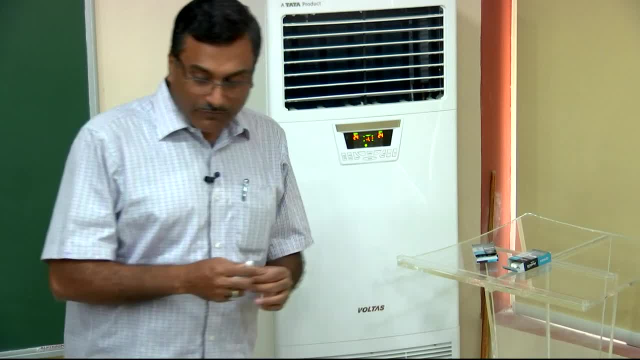 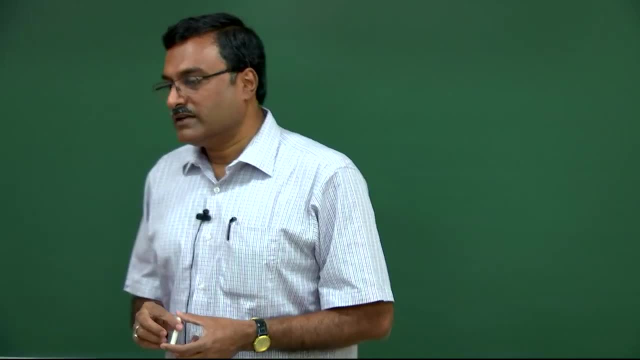 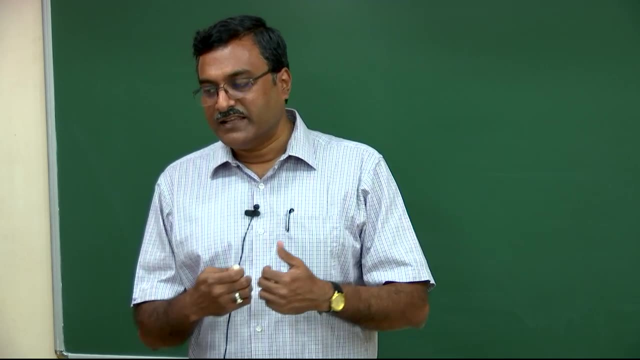 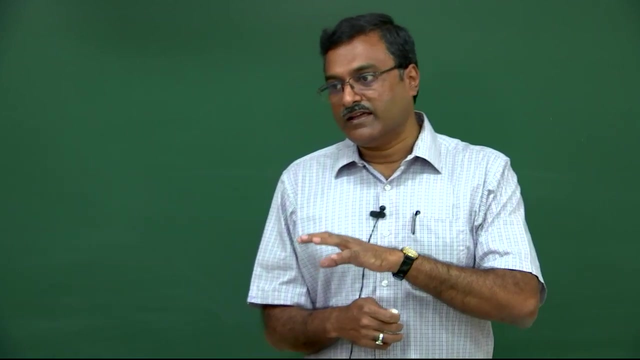 of equilibrium point. Now, of course, first of all I need to define what is an equilibrium point, and then I will be explaining you that, how a given non-linear system can be linearized around a equilibrium point, and study their stability behavior, And not in this lecture but afterwards, when I will be considering some practical problems. 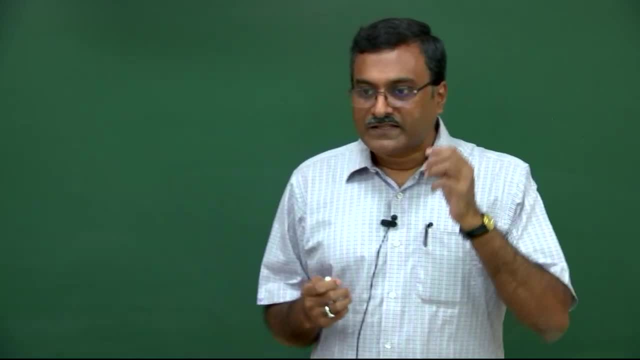 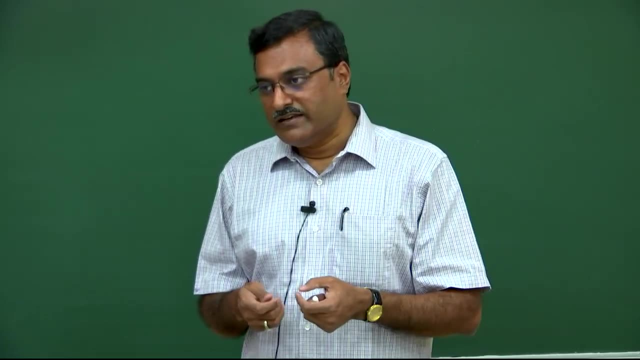 from population dynamics, then I will explain that, why this kind of linear stability is important. But briefly I can mention here that most of the non-linear system that we are having or we are dealing with those, are very complicated and most of the time you 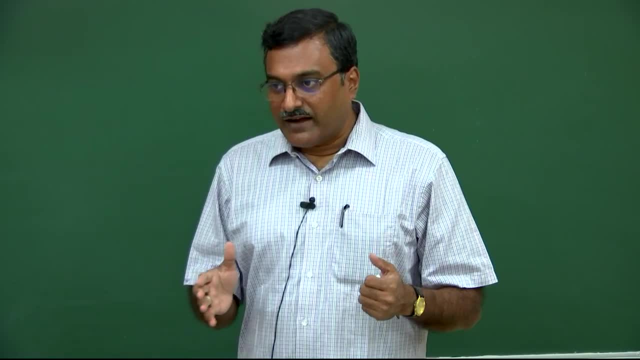 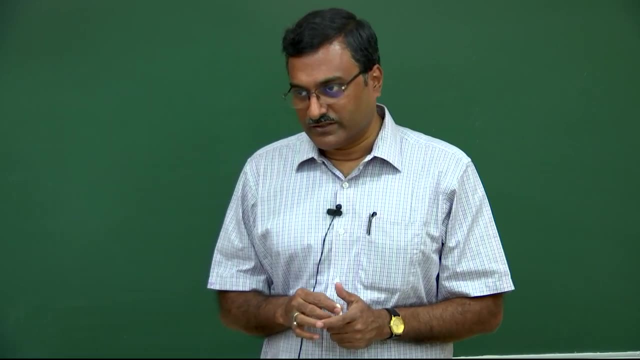 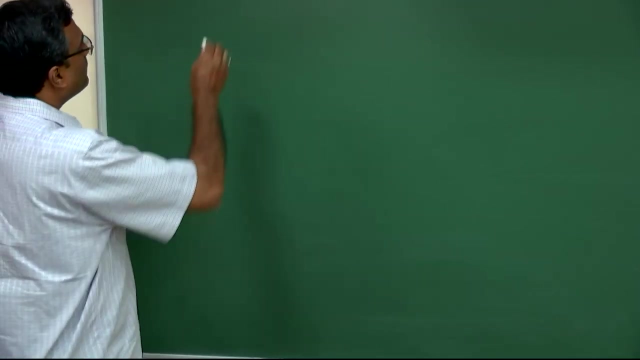 cannot find out any explicit shortcomings. 1 Solution and till today there is no way to find out a general solution for a non-linear ordinary differential equations. So first of all let us define what is a equilibrium point for a single variable system. So single variable system is defined by d, x, d, t equal. 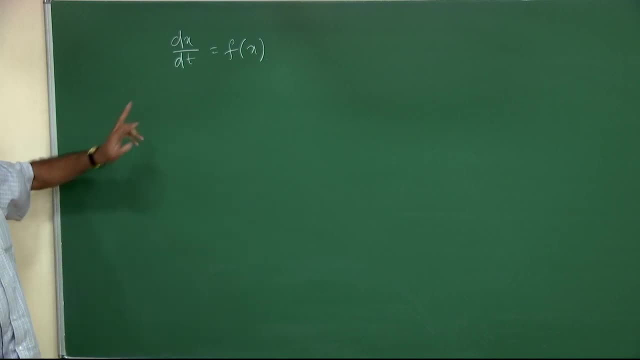 to f, x. Sometimes I will be considering this type of equation by introducing a parameter also, So that means some parameters will be involved with this system, because in case of bifurcation we are interested to study that how the system's behavior is dependent up on the particular magnitude or values of the parameters or some. 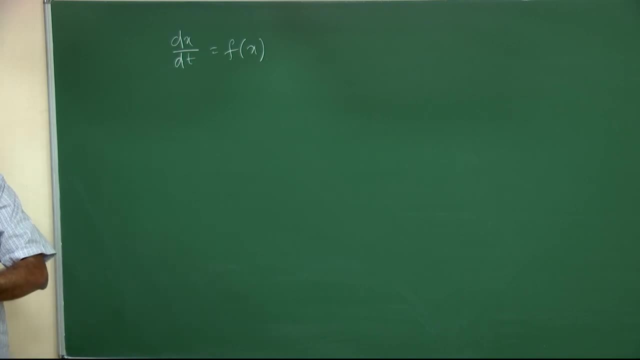 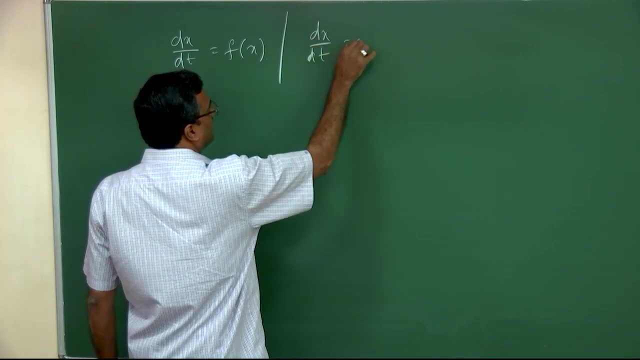 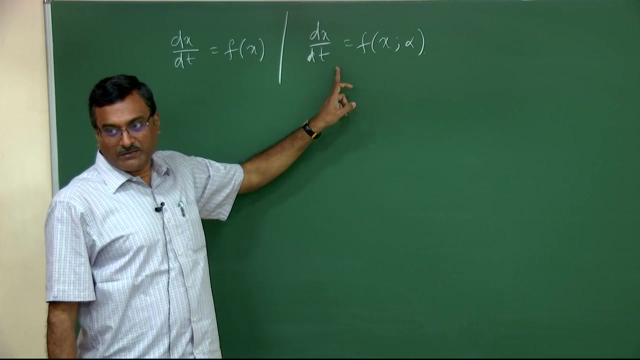 inter-relation of the parameters involved with the model system. So this is the most general form. alternatively, we can write down this system as d, x, d, t. that is equal to f of x, comma alpha. So x is the dependent variable, t is the independent variable. 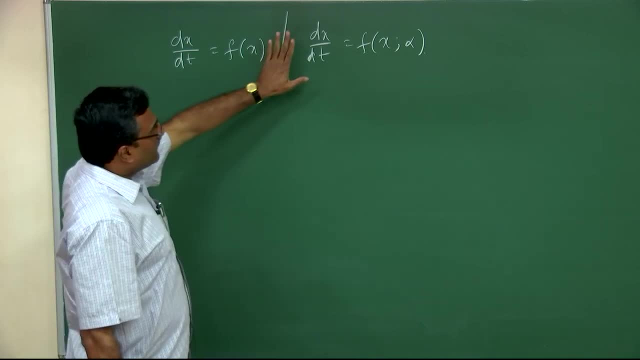 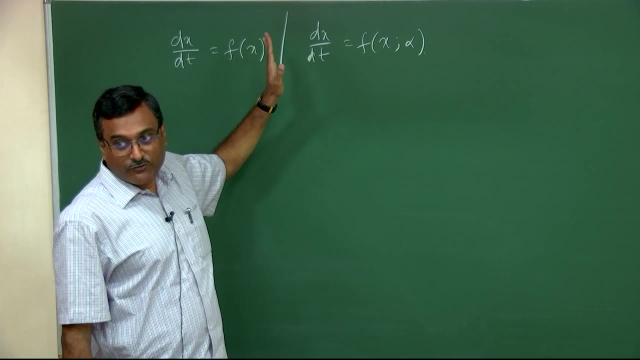 and alpha is the parameter. Now, for the time being, we are not concentrating on this equation. rather, we can concentrate on this particular equation because if I want to define the equilibrium in terms of this equation, that will be quite complicated for you at the initial stage. 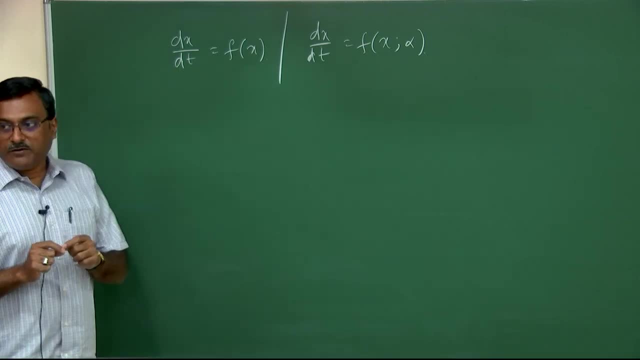 So for this system, what is an equilibrium point? Equilibrium point means it is a rest point. So if you start from here, trajectory will not move from this particular location. So that means velocity of x is 0 when x takes that particular value, which is labeled as. 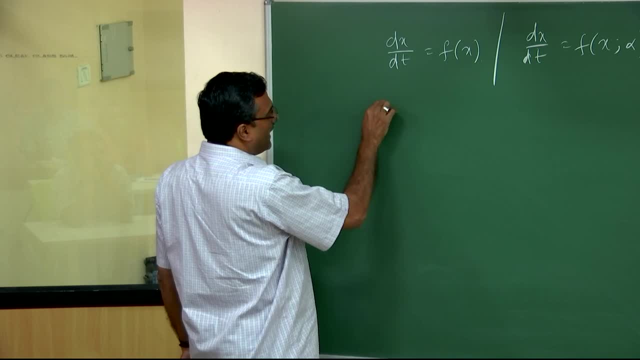 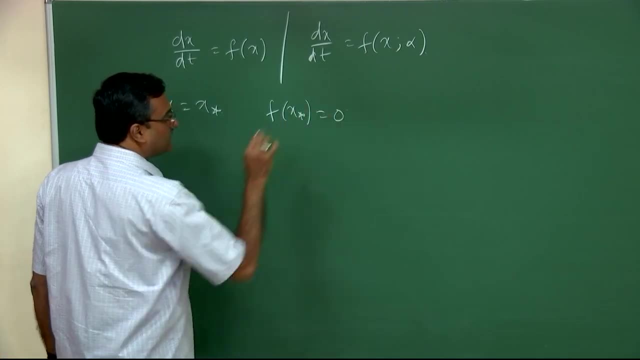 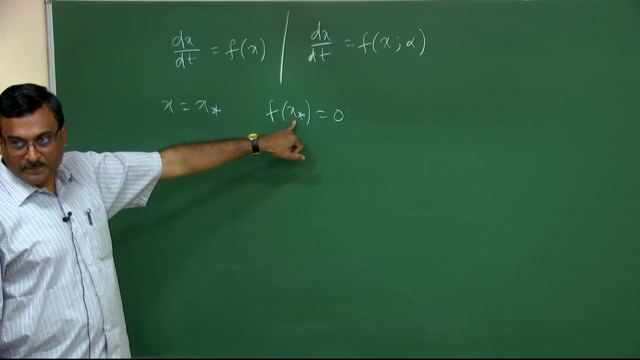 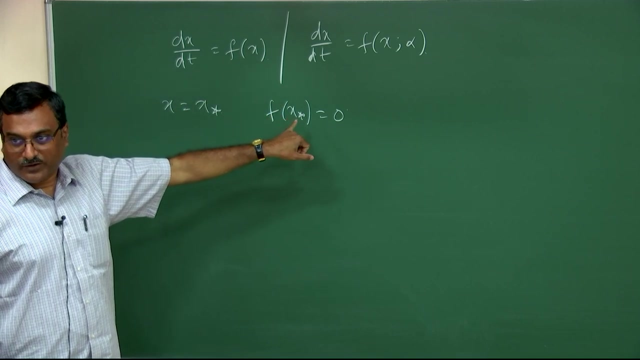 equilibrium, Then we can call x equal to x. star is an equilibrium if, and only if, f of x star. this is equal to 0. This is 0 means once your x equal to x star, then your dx dt equal to 0.. 0.. So therefore, x star is an equilibrium point or rest point. Now you need to keep. 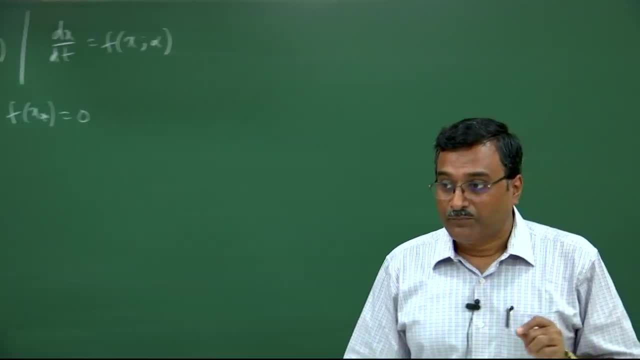 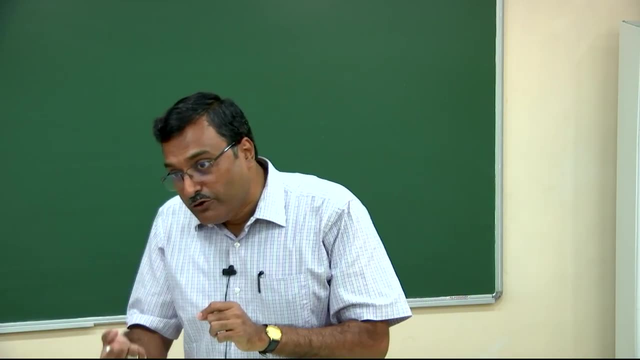 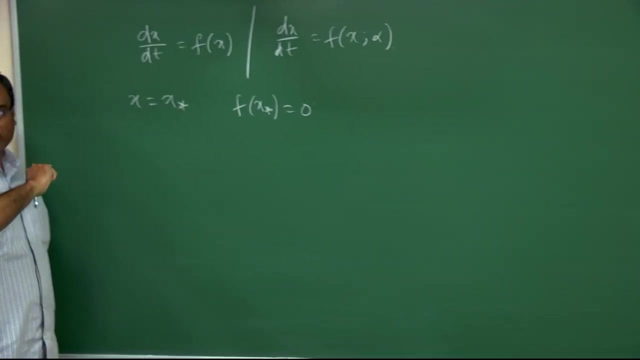 in mind that why we are interested for equilibrium point. We are interested for equilibrium point only for the reason because equilibrium point is itself a solution of the given system. Why? Because this is a non-linear equation. For most of the non-linear equation you cannot 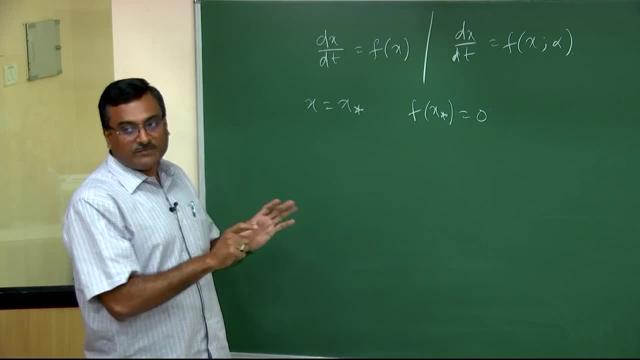 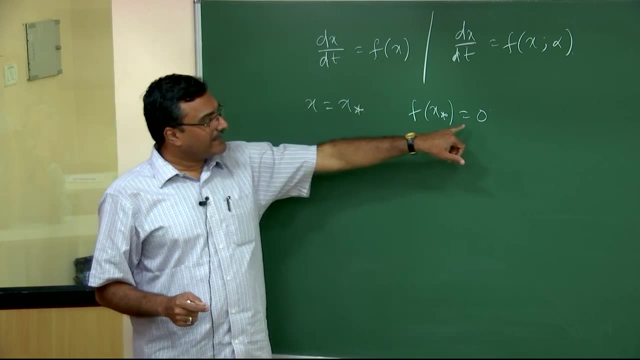 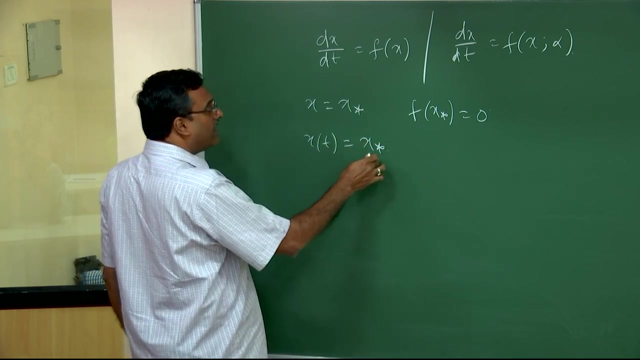 find out the general solution. For some of them we can manage a solution, but you can easily verify that if x equal to x star satisfies this condition, then x t, given by this constant value, x star, is a solution for this equation, Because f x star is, by definition, is equal. 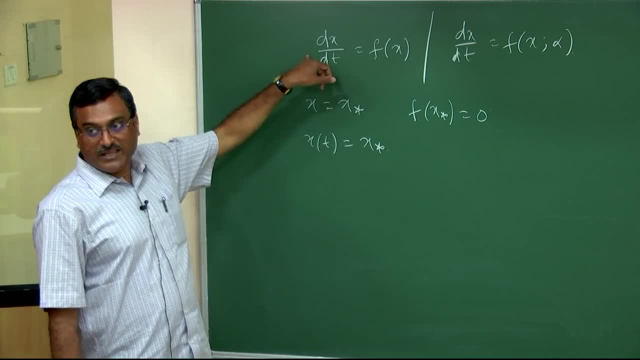 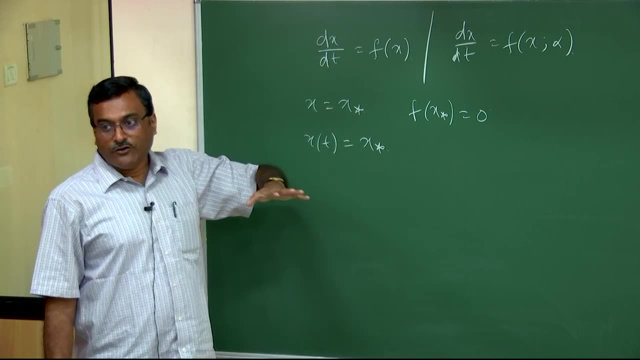 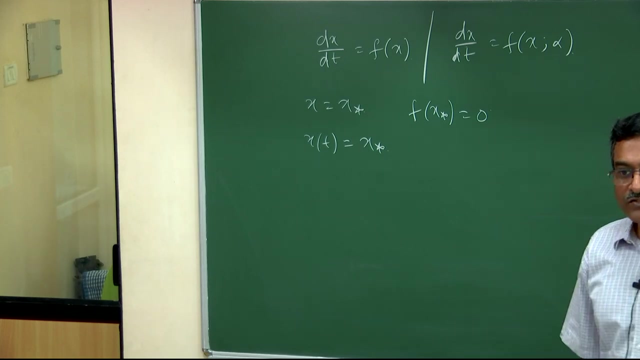 to 0 and derivative of x star with respect to t is 0, it satisfies the equation. So therefore it is an equilibrium point And sometimes it is also called an equilibrium solution for the given system. Now, before going to mathematical definition of stability of an equilibrium point and how to judge the 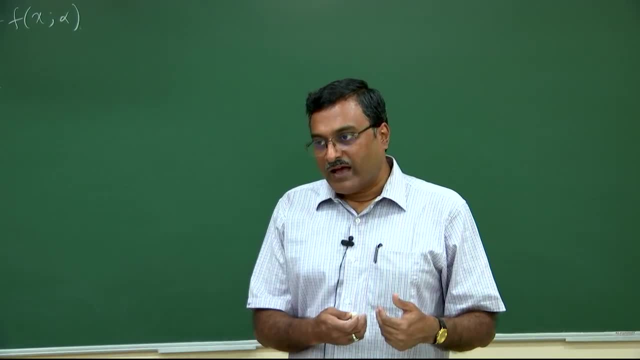 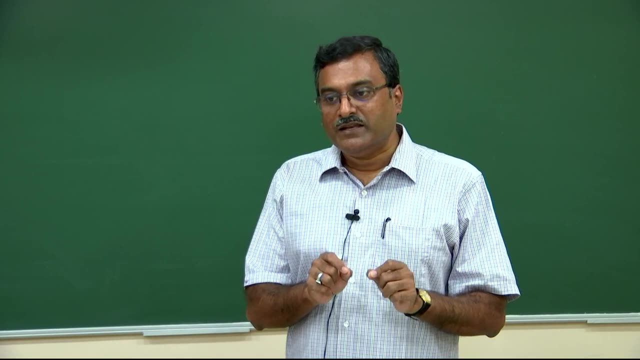 stability of a non-linear system by method of linearization. I just want to give you a very simple example- And from geometry you can understand that how we can determine the stability of the equilibrium point The given system is. for the time being, we can. 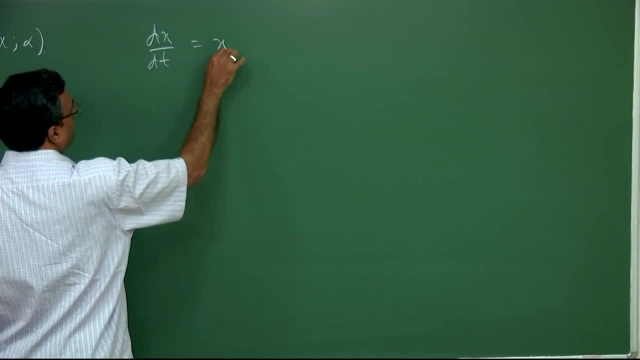 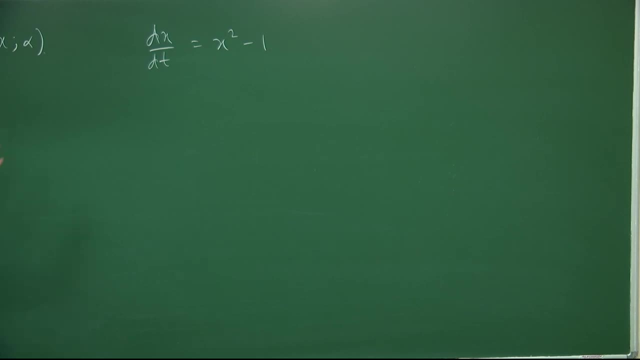 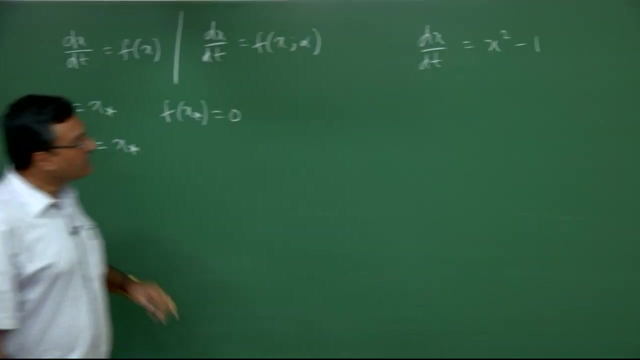 consider D x, d t, this is equal to x square minus 1.. So your f? x is given by x square minus 1.. So if you want to find out the equilibrium point, so that means some x star satisfying this condition. that means we need to solve the equation x square minus 1 equal to 0.. 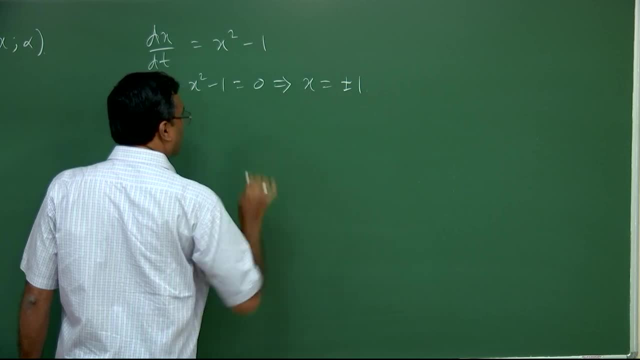 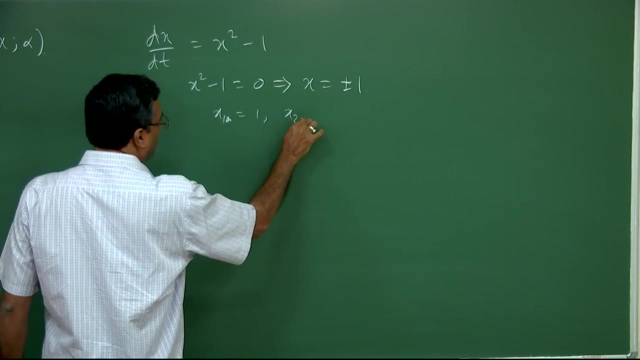 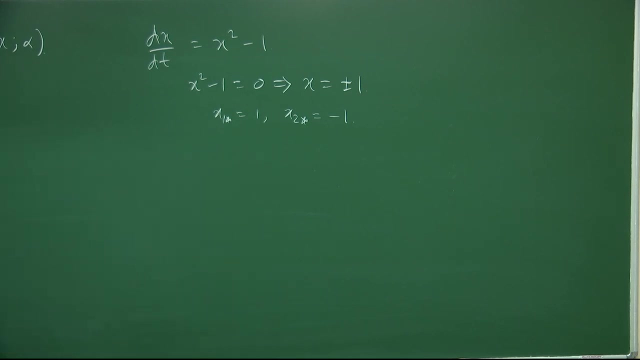 So this gives you x equal to plus minus 1.. And in terms of our notation x star, we can write x 1 star x 2 star. this is equal to minus 1.. So these two are equilibrium points. Now what are? 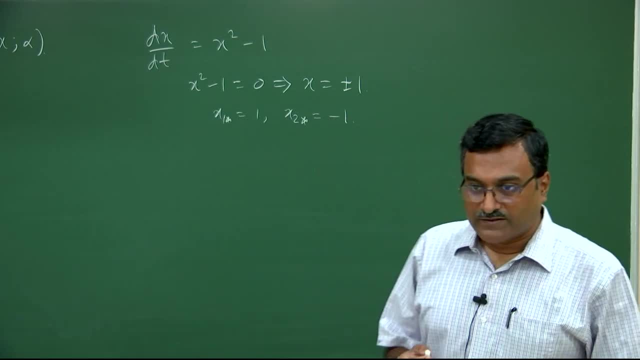 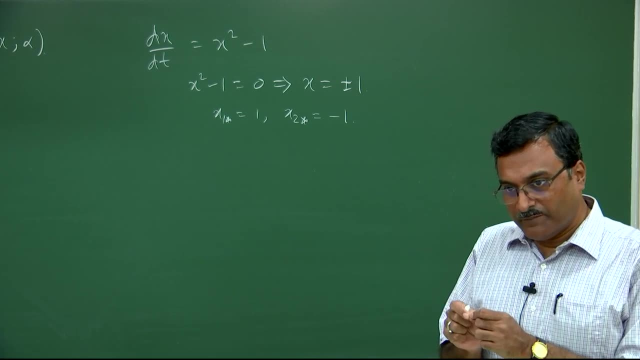 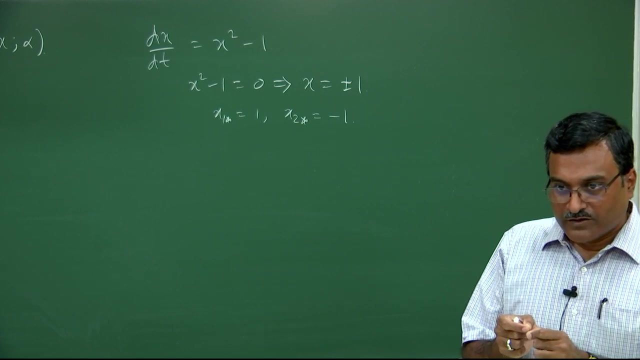 the stability concept of the equilibrium points. The answer is that if you give a small perturbation from the equilibrium point, then whether the solution trajectories has a tendency to come back to the equilibrium point or not. So in case of single variable, problem x, x square. 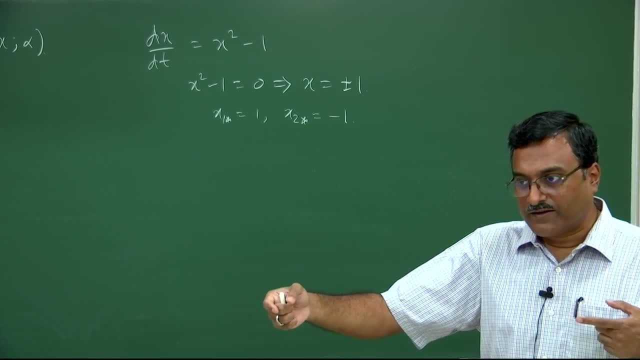 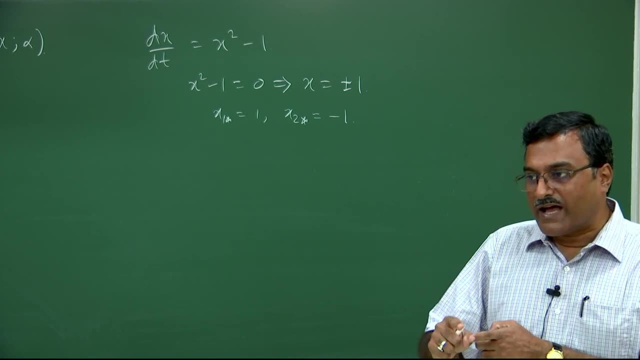 x is on x axis with the advancement of time, So you can give perturbation around the equilibrium points. that means you can give perturbation such that the point moves either on the right hand side of the equilibrium point or on left hand side of the equilibrium point. 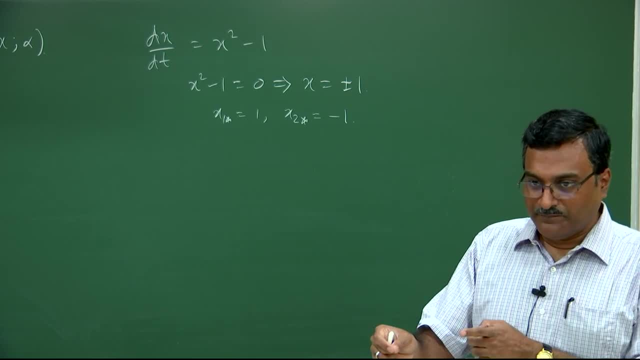 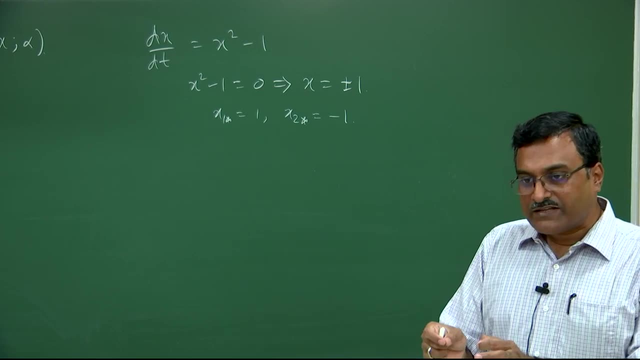 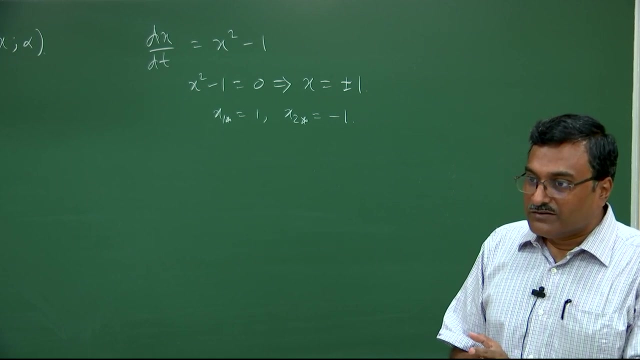 In other words, if we start from a nearby point of the equilibrium, then the solution trajectory will be approaching towards the equilibrium or not. If solution trajectory is from both side approaching towards the equilibrium point, then we can call it as a stable equilibrium. If not, then it is unstable. why I am saying if not, it may happen for certain system. it. 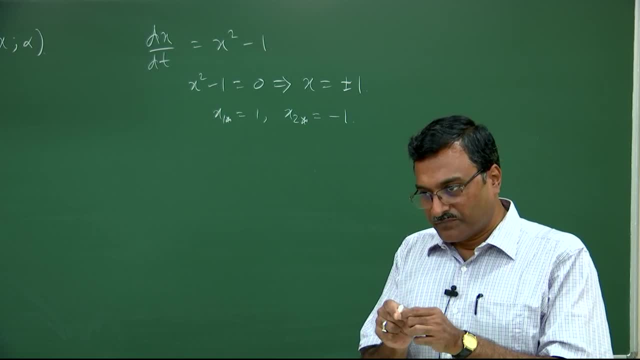 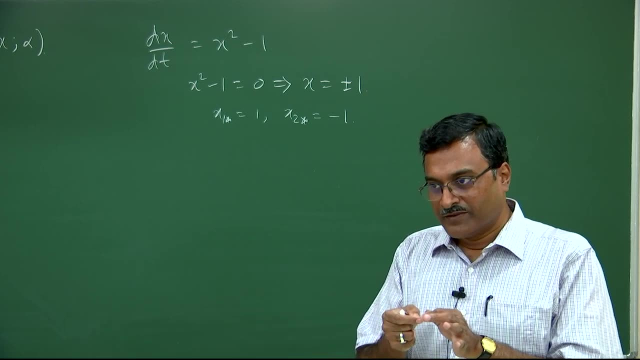 may happen that you have an equilibrium point. If you start from a point on the right hand side of the equilibrium, solution will be approaching towards the equilibrium, but if you start from a point on the left hand side of it, it may start diverging from the equilibrium. 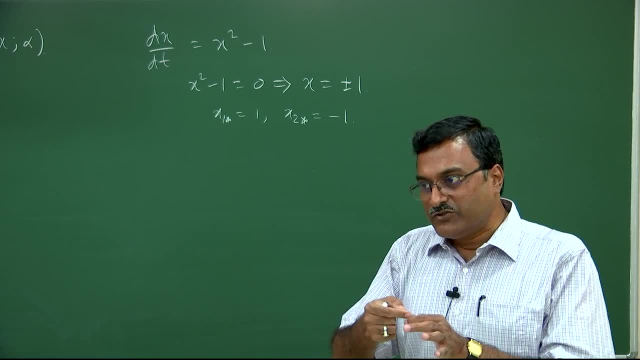 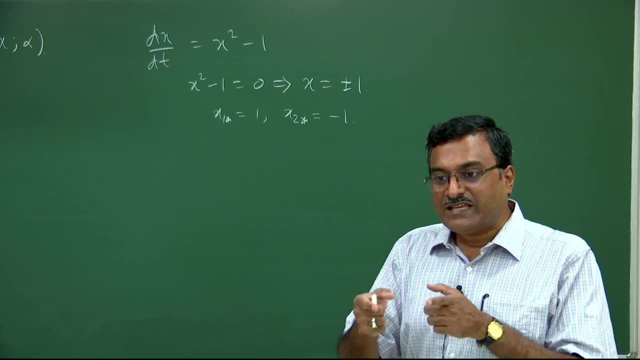 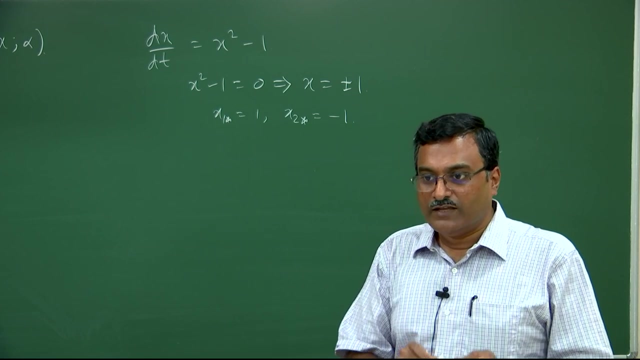 point In that case, although from one side it is approaching towards equilibrium, but from other side it is diverging from the equilibrium. So therefore, in combination we can say: this is unstable, because stable means from all the direction, solution trajectory should be approaching towards the equilibrium. point Now for this system, just looking at the property. 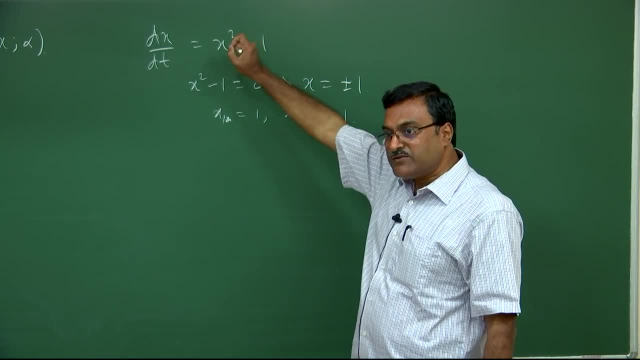 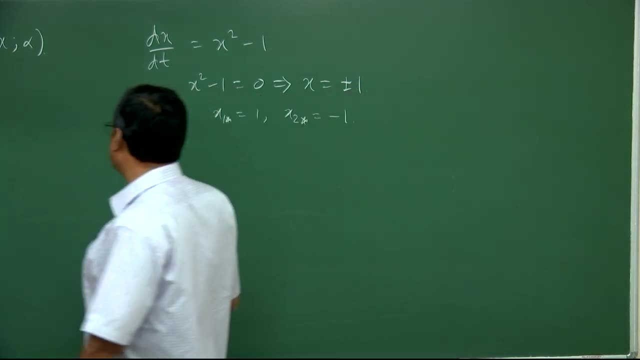 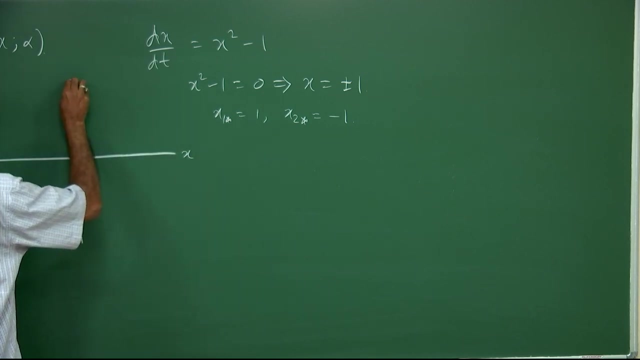 of increasing function and decreasing function in terms of derivative, we can judge the stability of these two points, These two equilibrium point. you just try to understand how it is possible. So first of all, we consider this graph. this is x direction and this is x dot direction In x x dot plane. 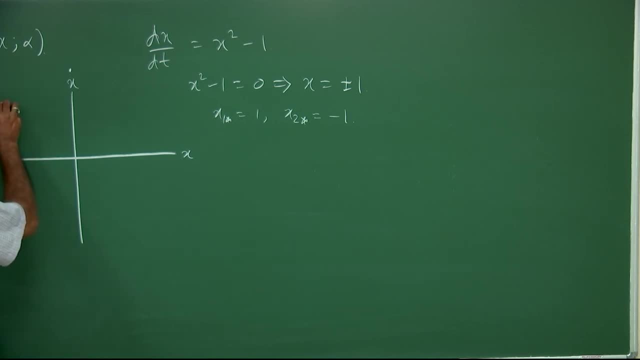 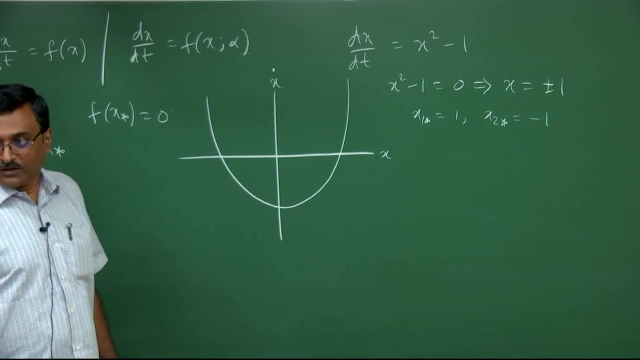 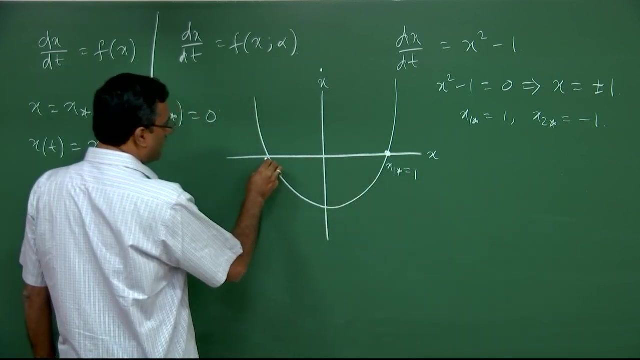 if you draw this curve x square minus 1.. So this will be a parabola like this: So this is your point. So x 1 star: this is equal to 1. this is this one, and this is your point. x 2 star: this is. 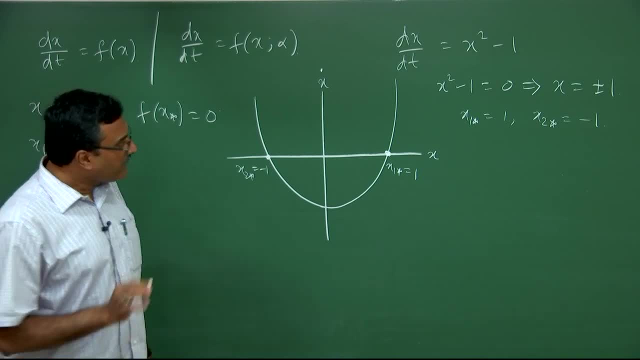 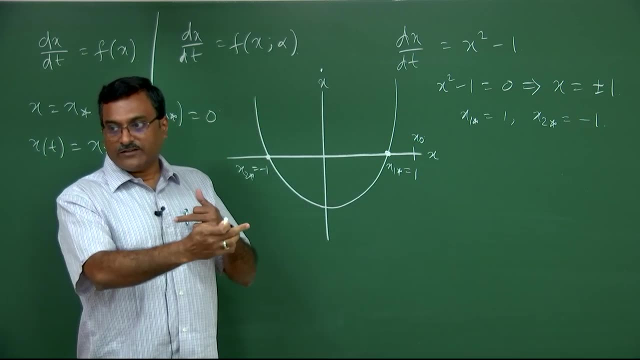 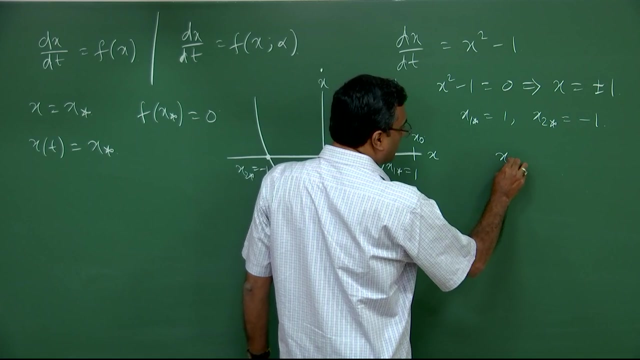 equal to minus 1.. Now you consider a point: x 0 at this position, that is, point is on the right hand side of the equilibrium, that is x 1 star equal to 1.. So this x 0 satisfies the condition that is x 0 greater than 1.. So x 1 star is equal to minus 1.. So x 0. 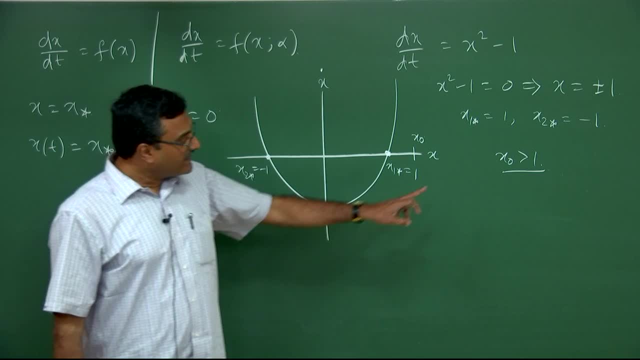 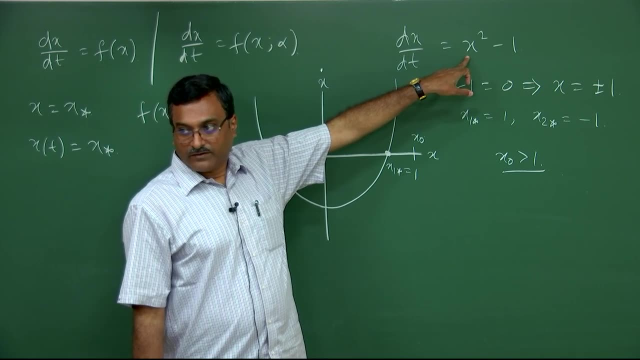 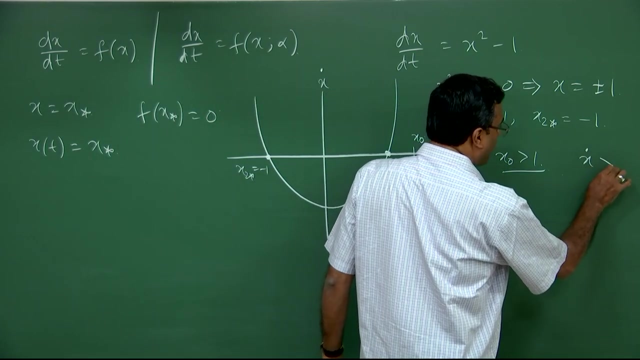 is greater than 1.. If your x 0 is greater than 1 and if you substitute this x 0 here, right? So what is the sign of the x dt? If your x 0 greater than 1, then x dot is also. greater than 1, correct? So therefore, what we can conclude? that x- t, this is an increasing function of t, right? you can consider the general format as x dot equal to f, x, y and y dot, this is equal to g x y. So these are system of two non-linear coupled OD, correct? So in this case also? 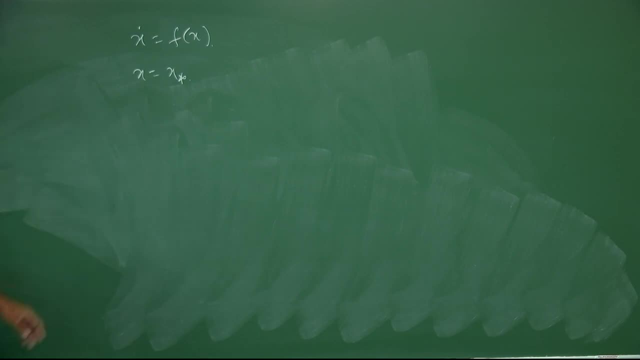 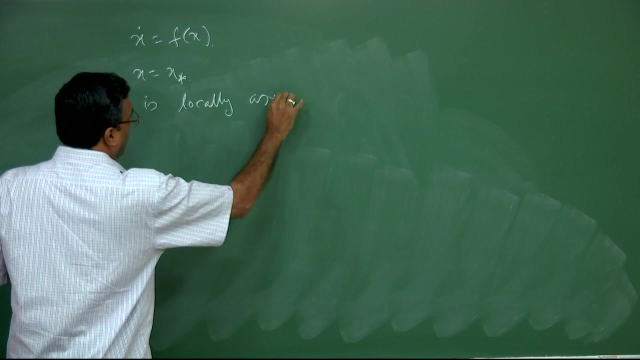 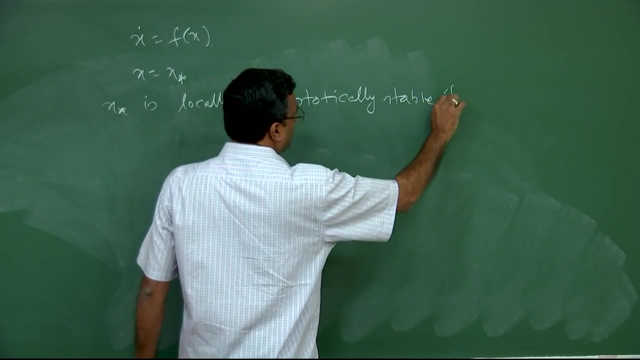 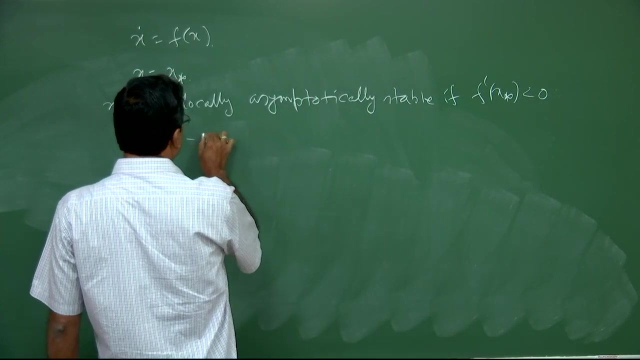 you can define that x star comma y star. this is an equilibrium point. this is an equilibrium point whenever your f of x star comma y star- this is equal to 0- is equal to g of x star comma y star. right Now we are interested to understand that, whether this equilibrium 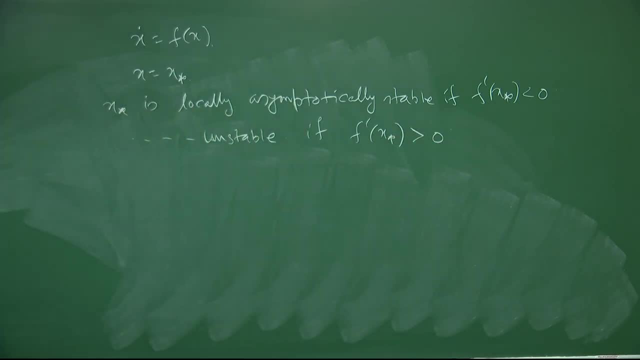 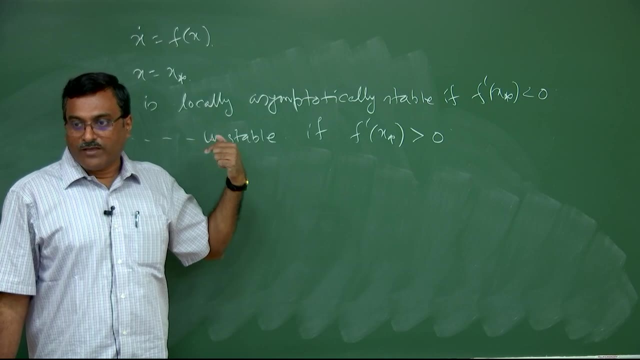 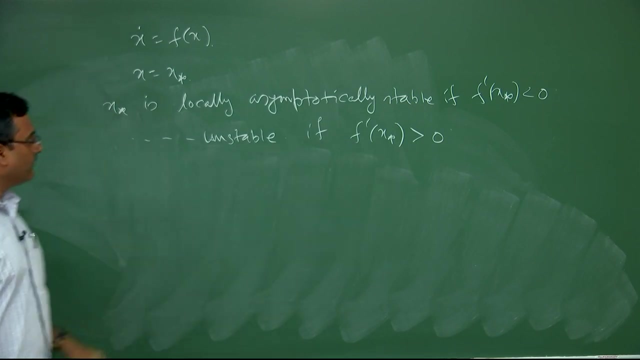 point is stable or not. So what we need to do, we need to give some perturbation around this equilibrium by x? t equal to x star plus u t, y t equal to y star plus v t, As earlier we can assume. 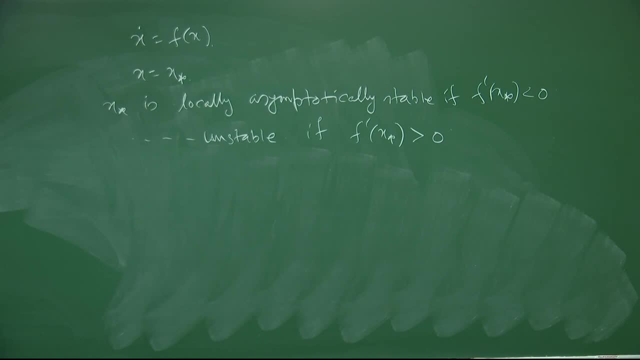 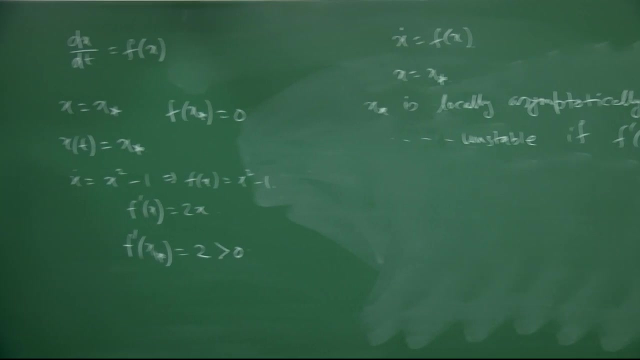 that both u and v, they are much, much less than 1, such that second and higher order can be neglected right Now. if both the Eigen values are negative or both the Eigen values have negative real part, then your u t and v? t will be approaching to 0, as t tends to. 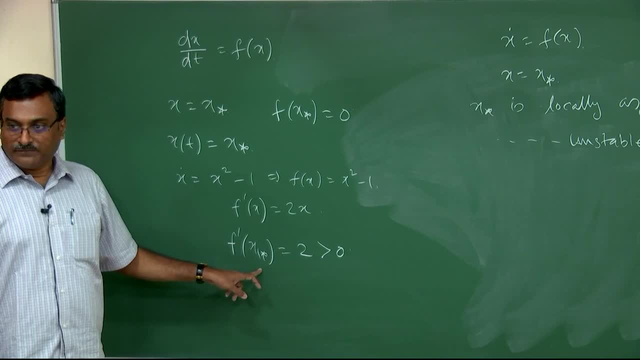 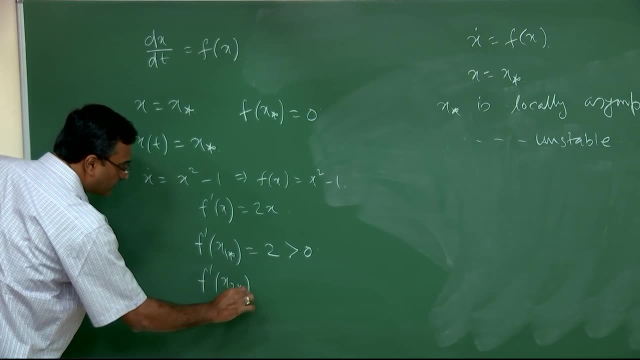 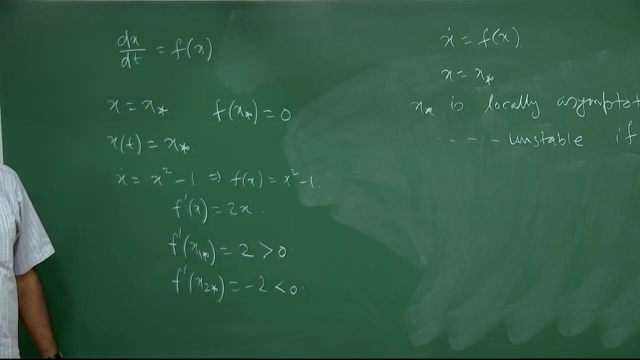 infinity. So therefore, stability condition for x star, y star of this non-linear system, that means local stability condition is given by that, both the Eigen values associated with the coefficient matrix given by a: 1, 1 a 1, 2 a 2, 1 a 2, 2.. 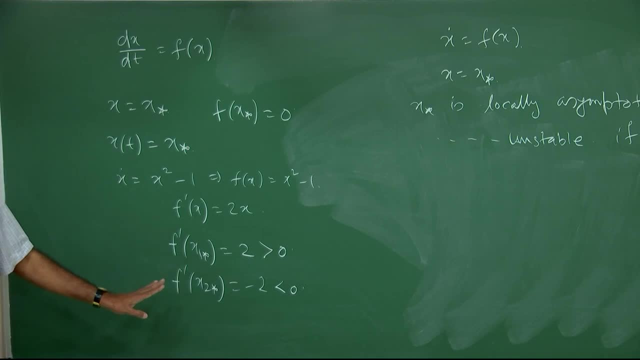 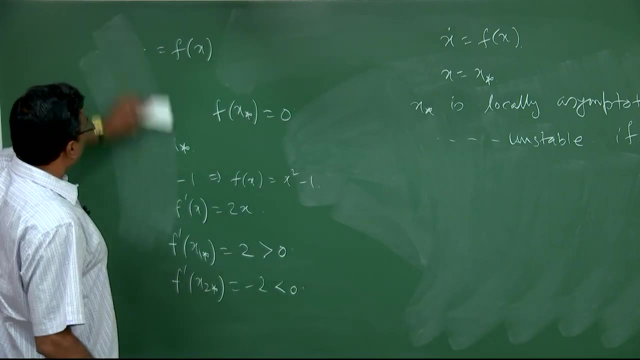 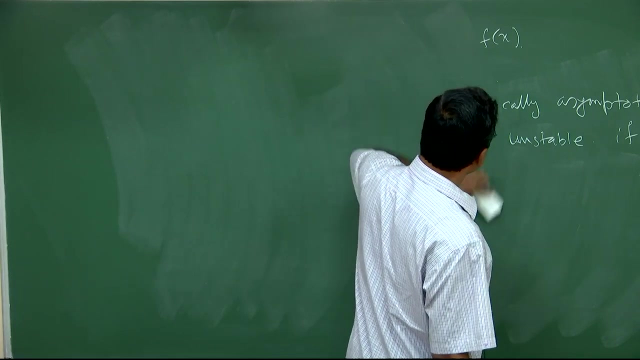 Should have either both real negative Eigen values or both the Eigen values with negative real part. Now the question is that how we can judge, or what are the conditions from which we can clearly understand that whether the solutions are stable or not. So question: 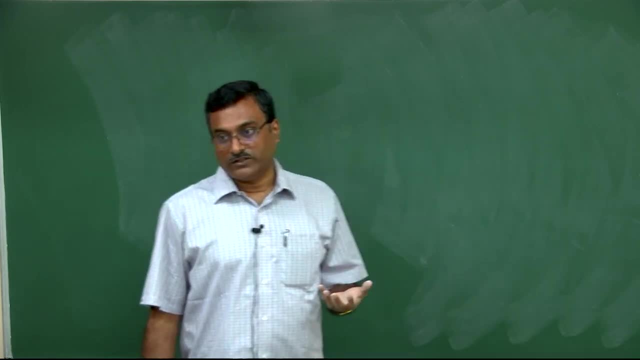 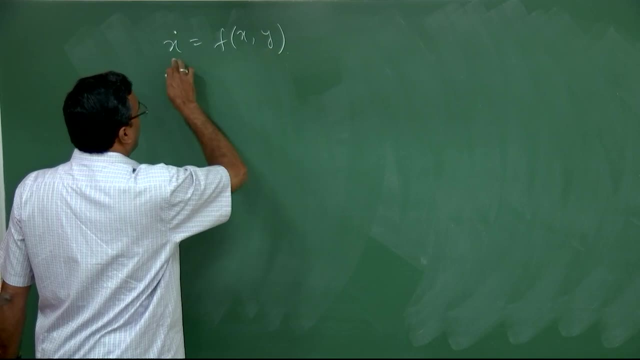 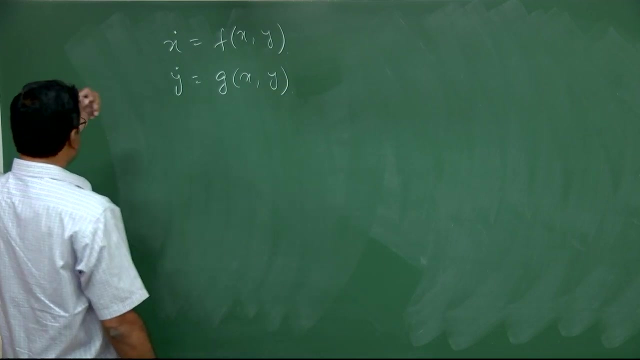 is that whether we need to find out the complete solution? answer is no. There is a very specific way or other simple logic from where you can easily check, in case of two variable system, whether the zero solution for this linear system is stable or not, and accordingly you can conclude that. 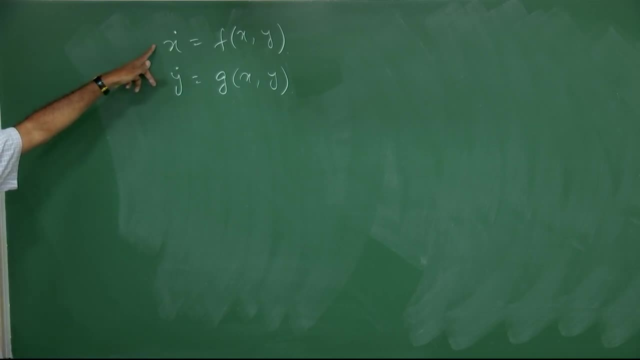 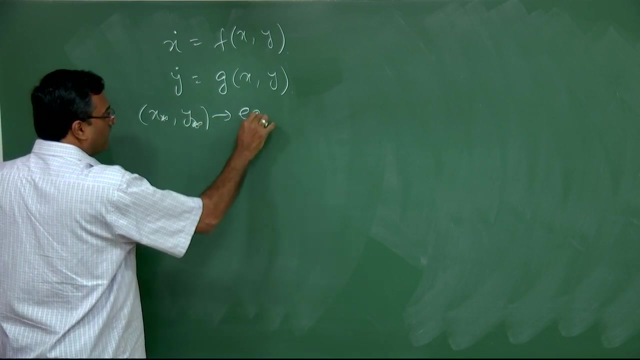 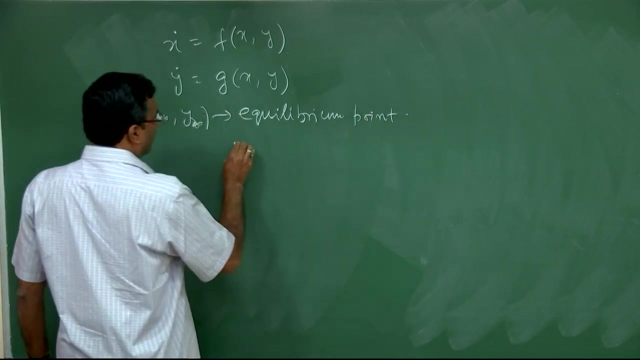 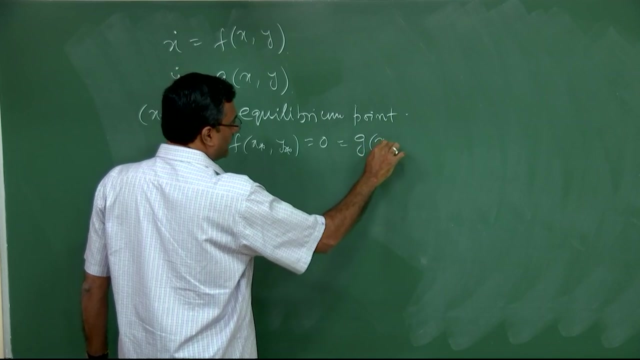 whether the equilibrium point x star, y star for the non-local system- sorry, non-linear system- is locally asymptotically stable or not. Now for this system. we can put it into the compact matrix notation that is: d d t of u v, that is equal to capital A multiplied with the column vector u v, where A is the matrix. 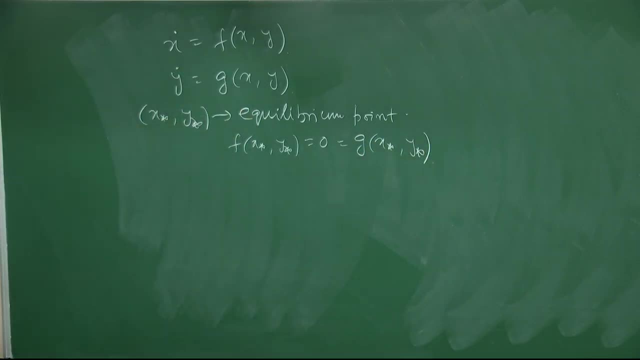 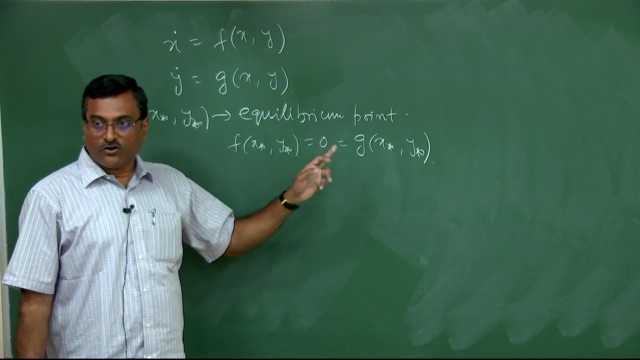 A 1: 1, A 1: 2, A 2: 1, A 2: 2.. This is also called Jacobian matrix. Jacobian matrix for the given non-linear system and evaluated at the equilibrium point x, star, y, star. 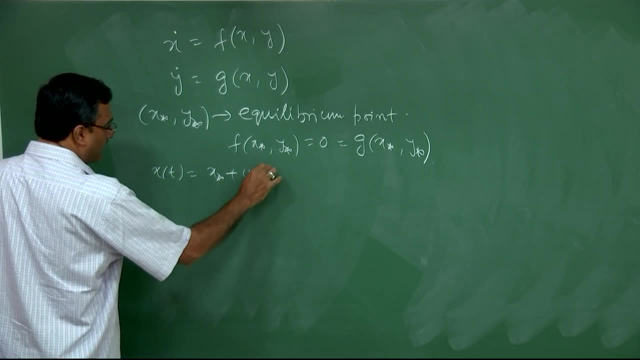 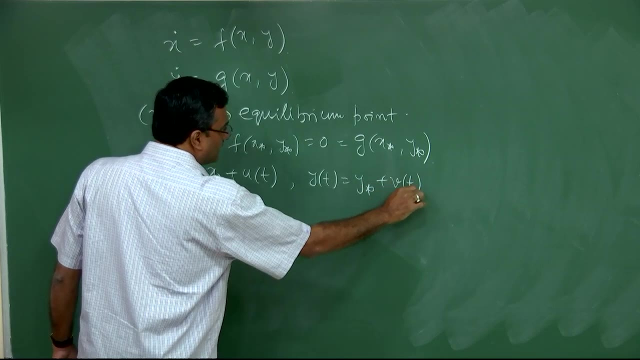 Because all the non-linear system is non-linear. the non-linear system is non-linear because all these A, i, j's, they are defined by these expressions. So therefore, this is partial derivatives with respect to x and y, of f and g and evaluated at the point x, star comma. y star. Now, Eigen values are actually roots of the characteristic equation that is, A minus lambda i, 2, this determinant, this is equal to 0.. If you expand this system then you will be having lambda square minus A 1, 1 plus A 2, 2, multiplied with lambda plus A 1, 1, A 2, 2 minus A 1, 2 A. 2: 1, this is equal to 0.. So this is your characteristic equation. Now you can just have a close look to this expression. you can write this equation as: lambda square minus trace of A, multiplied with lambda plus date of A plus date of A, this is equal to 0, correct, without a loss of generality, you can assume. this, And once this is the case, and if you denote trace of A by P and determinant of A by Q, so then this equation can be simply written as P, lambda plus Q, this is equal to 0. So once you have this quadratic equation is roots are given by lambda 1 comma 2, that is equal to P plus minus root over P square minus 4 Q divided by 2, correct P plus minus root over P square minus 4 Q by 2.. Now what we are looking for? We are looking for the stability of this literature. Linear system. so that means we need any one of two conditions should be satisfied: Number 1, either lambda 1, lambda 2, both less than 0 or real part of lambda 1 as well as of real part of lambda 2, both of them is less than 0. This is the requirement for the stability. of 0 solution of the linear system And accordingly, we are looking for the stability of the linear system And accordingly, we are looking for the stability of the linear system And, accordingly, local asymptotic stability of equilibrium for the non-linear system. right Now, if you look at this expression, so there are two possibilities. In this case that means both the roots are real and negative. This case 1 corresponds to the requirement that P square minus 4 Q is greater than 0, which ensures both the roots are real right. Now how can we ensure that both the roots are negative? We can ensure with this one, if we demand that P is also less than 0.. Now you just try to understand that P negative, P square minus 4, Q is positive. The possibilities is that either Q greater than 0 or Q less than 0. Now, in this case we can exclude the possibility q less than 0, why? Because if q less than 0, then from this equation you can observe that product of the root is negative. product of two roots is negative, so which clearly implies one root is positive. another root is negative. so that means the requirement- both of them negative- is already violated right Now. if we assume that q greater than 0 with p less than 0 and this condition is satisfied, then we can ensure that equilibrium, that is, x star comma, y star for the non-linear system. is locally asymptotically stable. similarly, 0 solution for the linear system is also locally asymptotically stable. Now, from this condition, how we can ensure both the roots are negative? also, this ensures roots are real. your p is negative, q is greater than 0, so then just try to convince yourself. 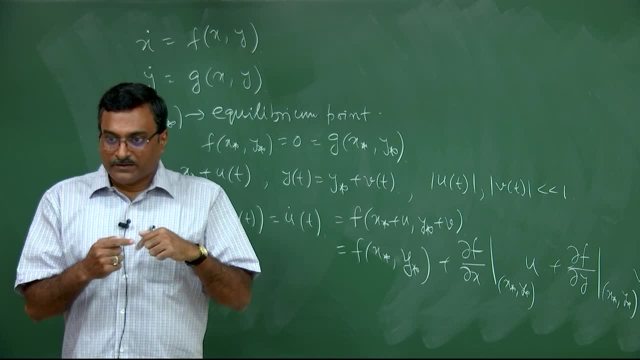 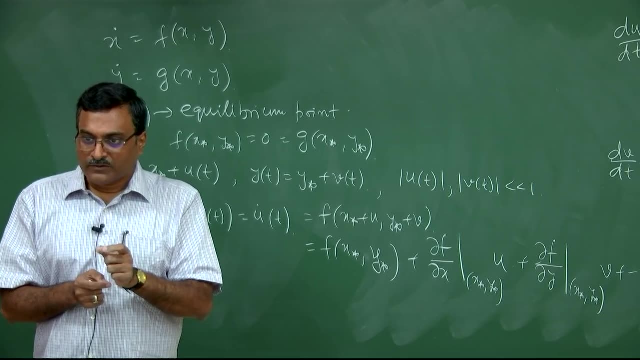 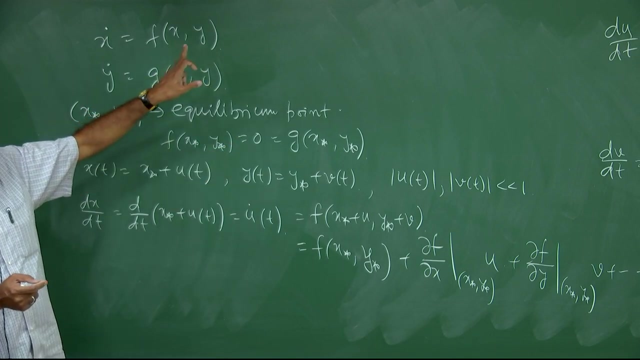 that this quantity, that is, root over p square minus 4 q, has the magnitude less than p, because this is p square minus 4 q, with q positive. So therefore, this quantity- Okay, This quantity- has the magnitude less than p. your p is already negative, so whenever. 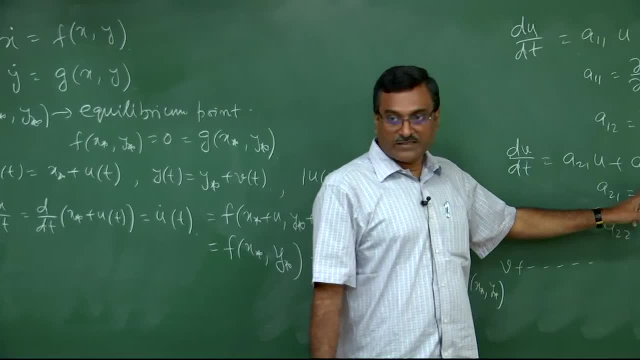 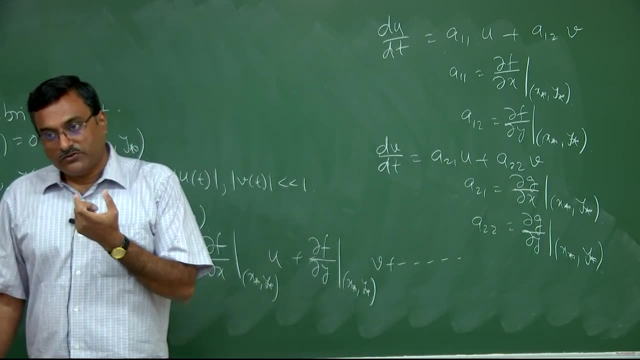 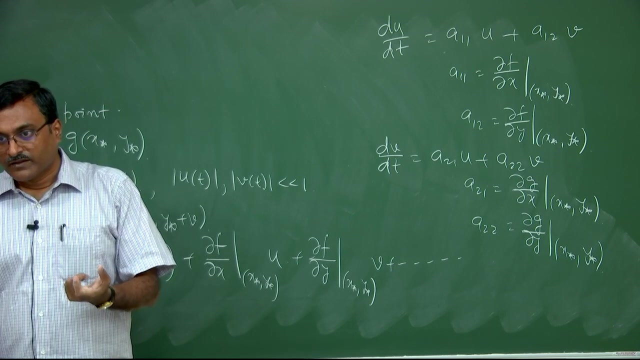 you are adding a quantity with magnitude less than p, then the resulting quantity is negative, and then p minus this quantity is clearly negative. so both the roots are negative. Similarly, you have one more possibility, that is p square minus 4 q. this is less than 0,. 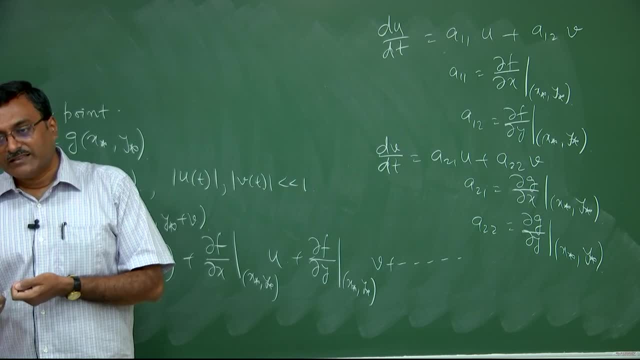 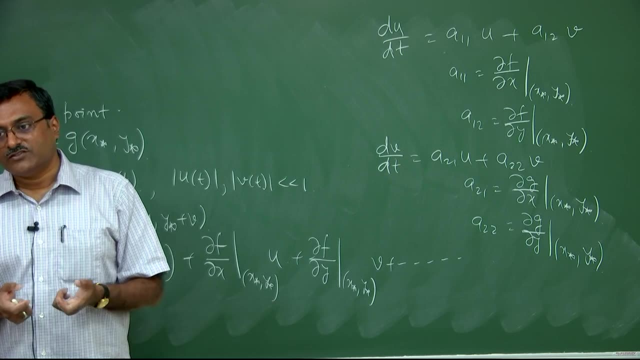 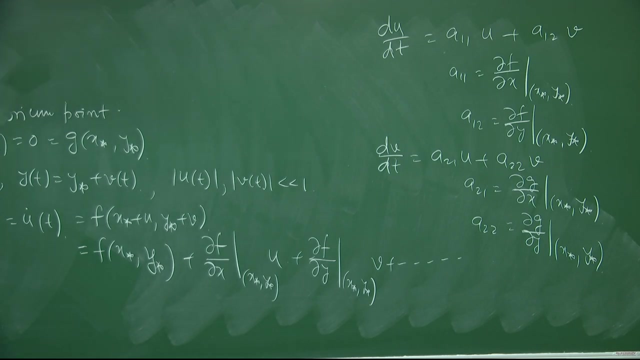 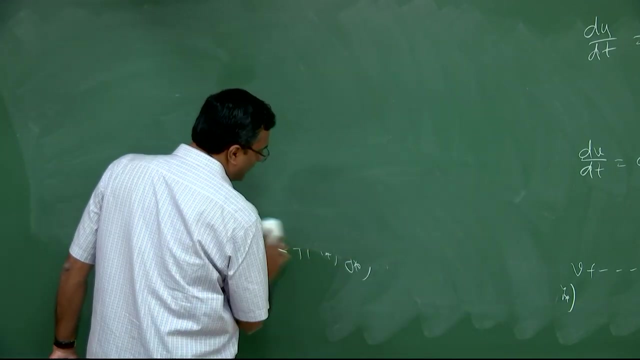 if you have this condition, that p square minus 4 q is less than 0, then automatically, if p greater, p less than 0, then it ensures that both the roots are actually complex conjugate with negative real part, because p square minus 4 q less than 0 implies that roots are complex. 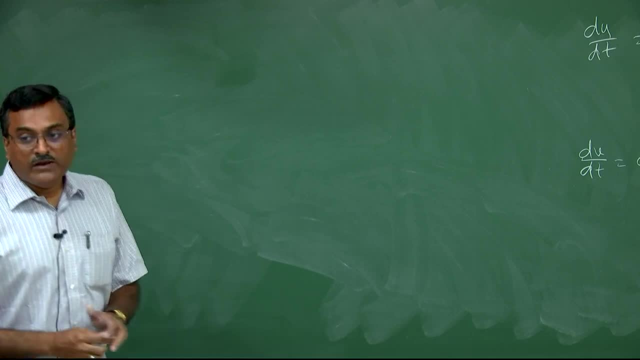 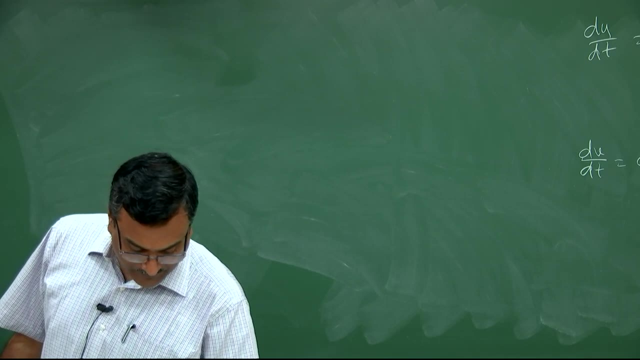 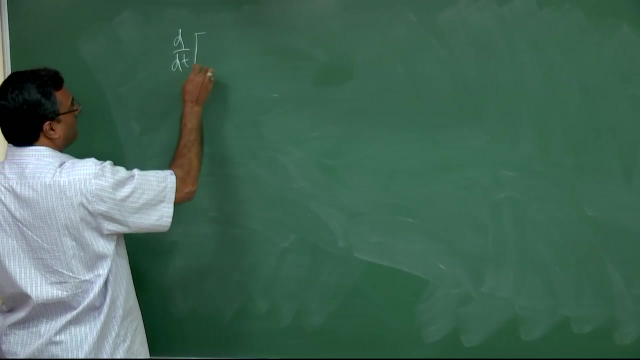 conjugate. Okay, So this will give you the imaginary part. and p less than 0 ensures that both the roots are having negative real part, correct? So therefore, if we combine these two conditions, if we combine these two conditions, then we 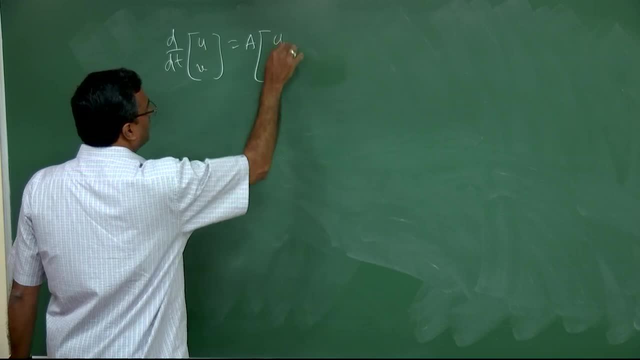 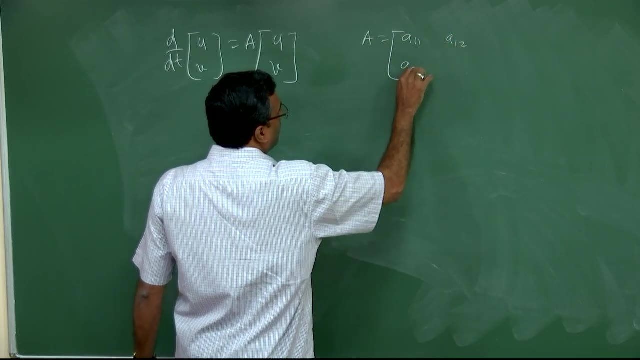 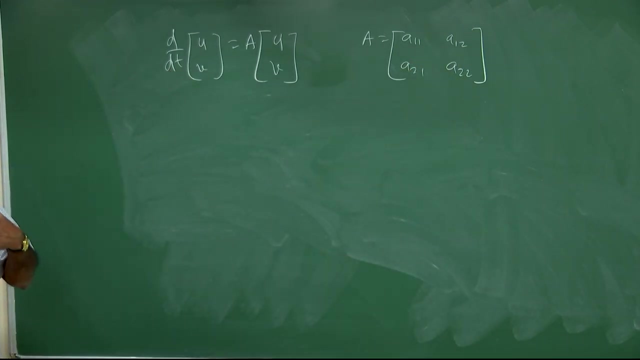 can say that u comma v equal to 0, comma 0 is stable is stable if u comma v is less than 0.. Okay, So this is the condition. Okay, Okay So this is the condition: p less than 0 and q greater than 0.. 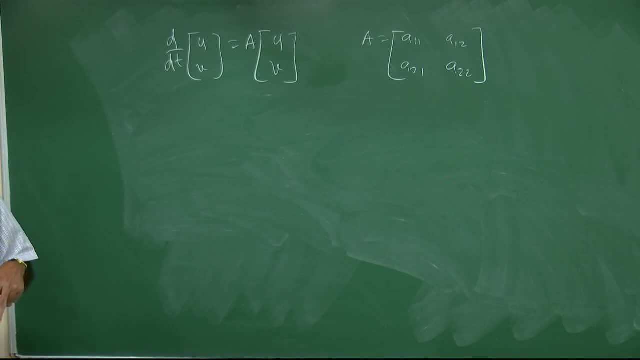 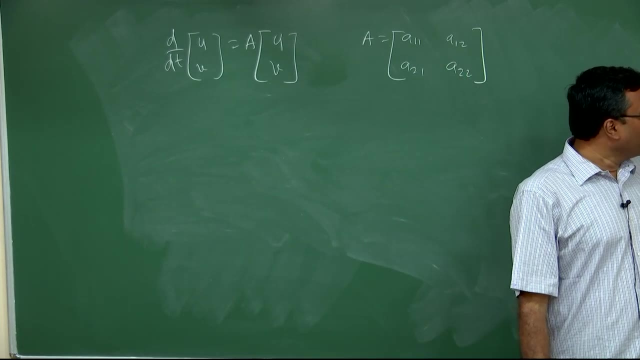 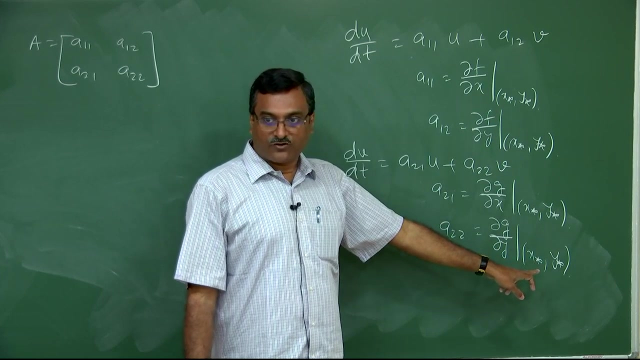 If any one of these two conditions are violated, then you will be having that equilibrium point which is unstable. Now the question is that in previous lecture I have shown some different types of phase portrait. Now the main question is: all those phase portraits can be related with these two quantities p? 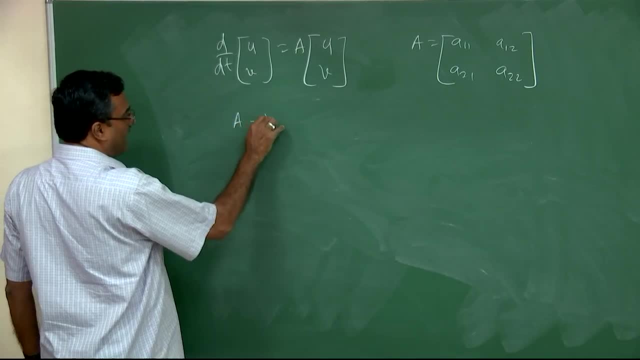 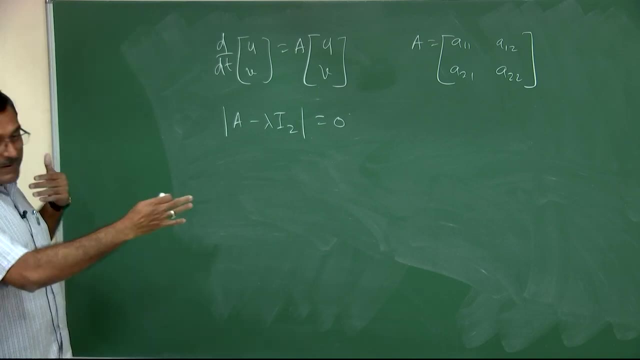 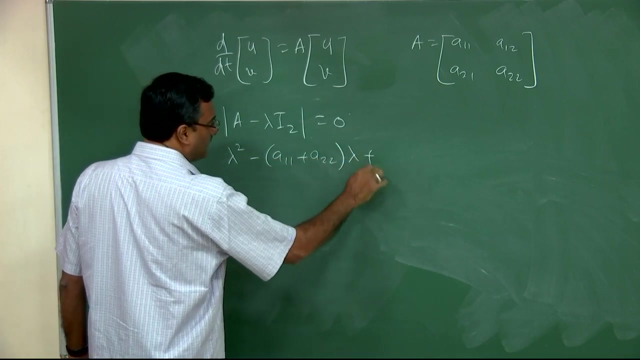 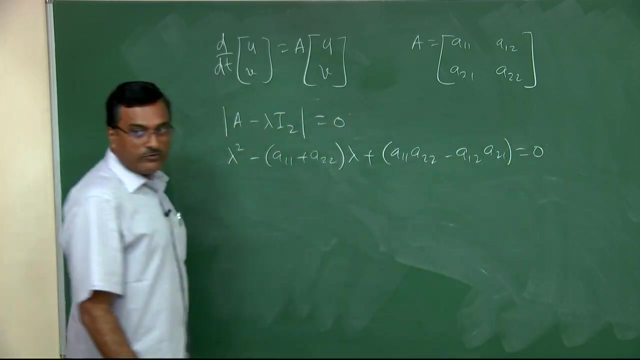 and q Answer is yes. Now I will explain how that can be done in p? q plane. So first of all, you just try to convince yourself. this is your p axis, this is your q axis. with some particular intention, I am not extending the lower part. 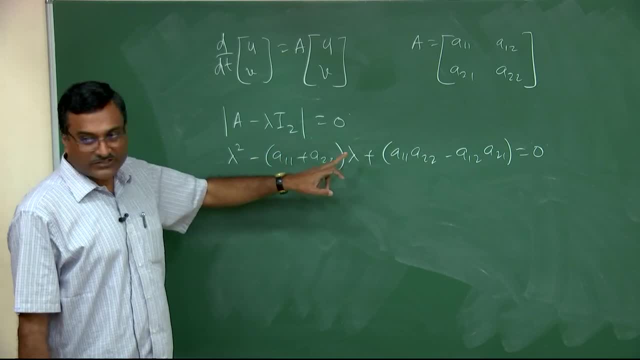 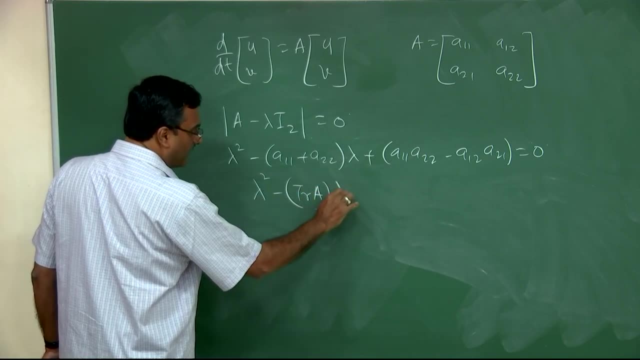 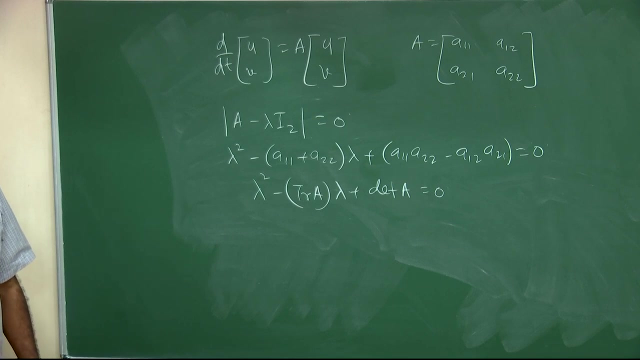 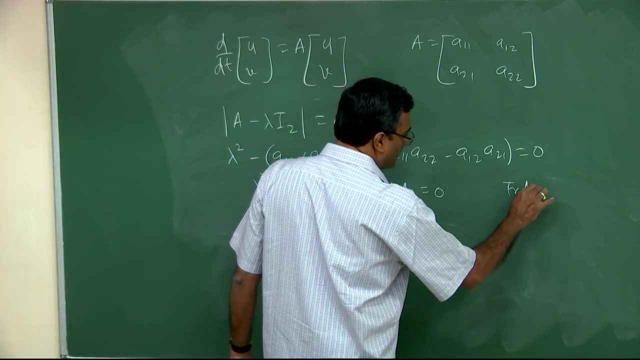 Why? Because from previous discussion you can recall that whenever q less than 0, then product lambda 1, lambda 2. this is negative, correct. So therefore, what you are having, that means what kind of conclusion you are having about the equilibrium, that both the Eigen values are of opposite sign, real and with opposite 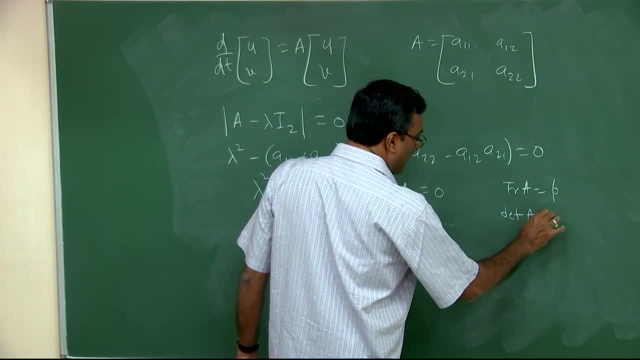 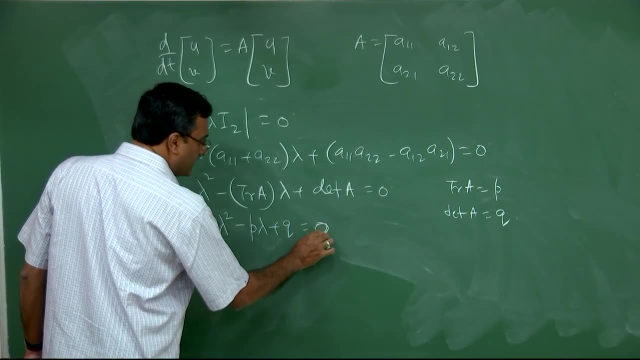 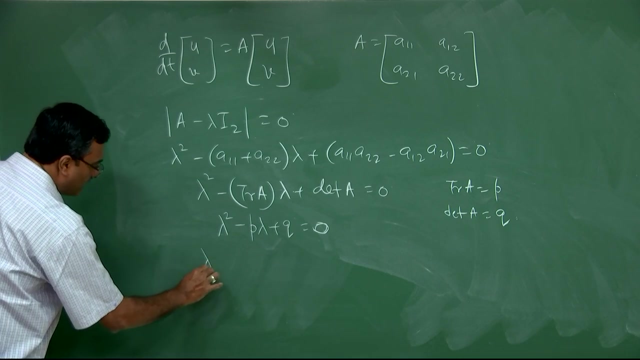 sign. So therefore, equilibrium point is a saddle point. Yes, Yes, Yes, So that is for q less than 0. you will be having this one, Suppose this is approaching to this direction. this is approaching to this direction. So therefore, your phase portrait in this domain will looks like this one or some format. 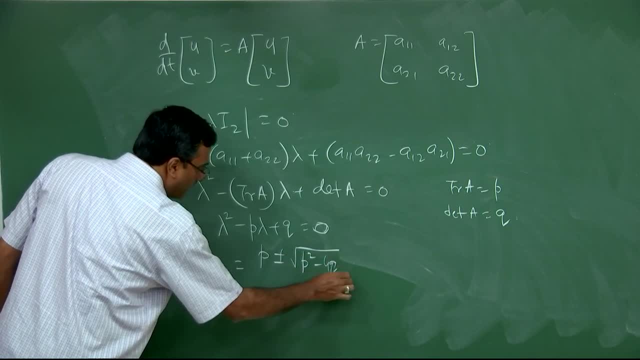 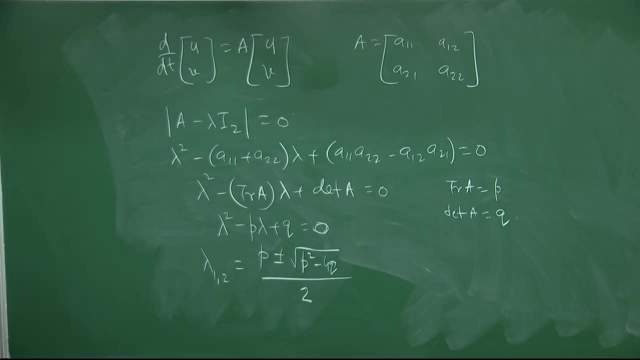 which is topologically equivalent to this one. So that means either any one of these two axis will be rotated or stretched, depending upon the given coefficients you are having for the system under consideration. Yes, Yes. Now the rest of the part we are left with that is p square minus 4q, less than 0 or p. 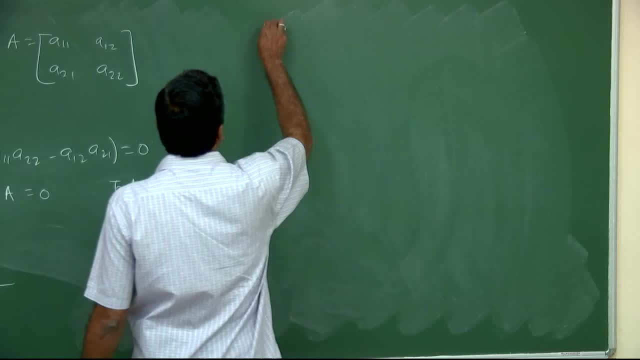 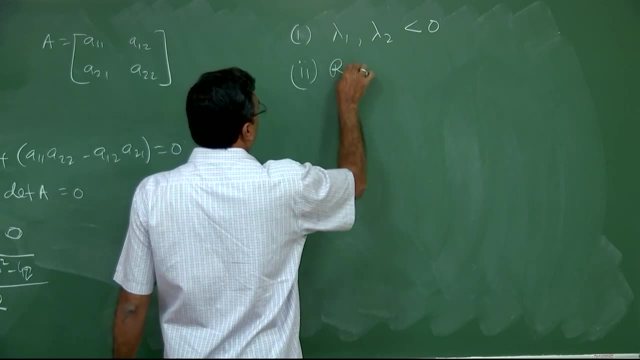 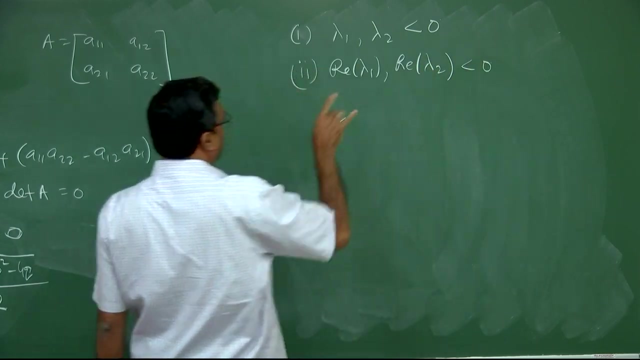 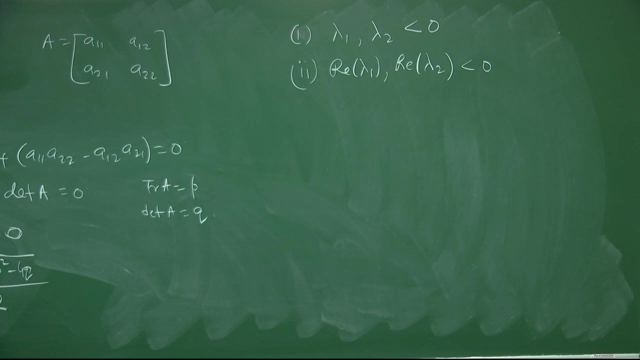 square minus 4q greater than 0.. So, of course, p square minus 4q equal to 0. this is given by this parabola, correct? So once you have this parabolic structure, then you should keep in mind that your equilibrium point, that is, 0 comma 0, is stable whenever p less than 0.. 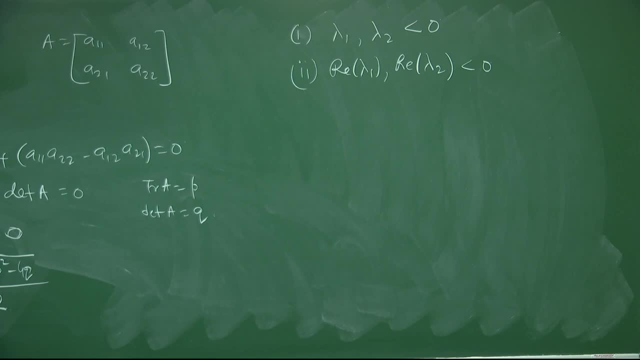 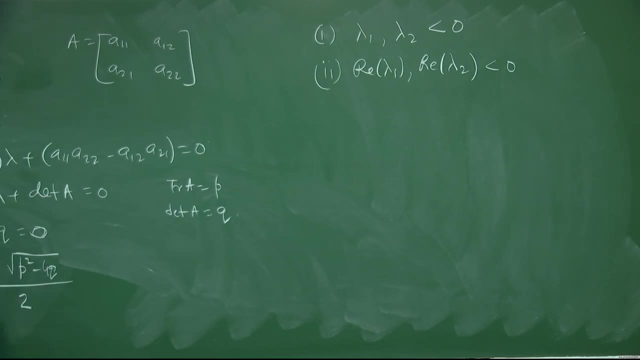 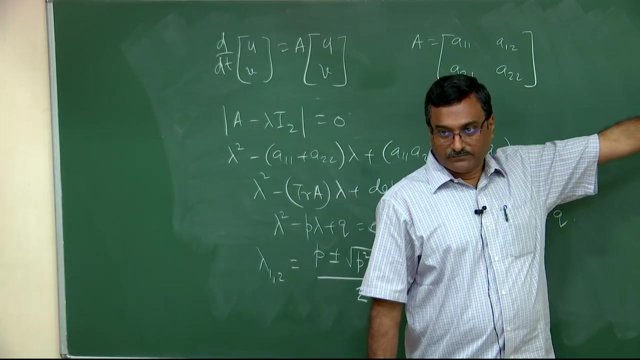 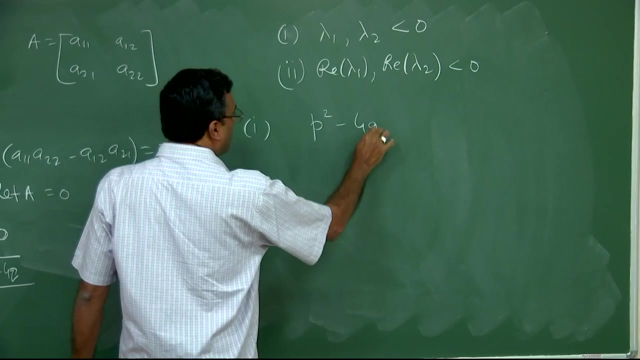 So on this side it is stable, on that side it is unstable, correct? Now, first of all, you can convince yourself: within this domain, that is, inside the parabola, your p square minus 4q is negative And outside the parabola, p square minus 4q is positive. 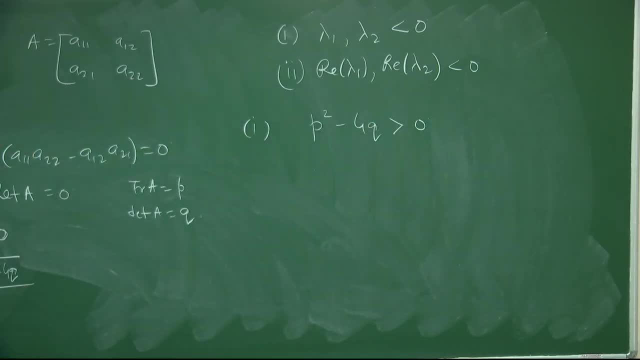 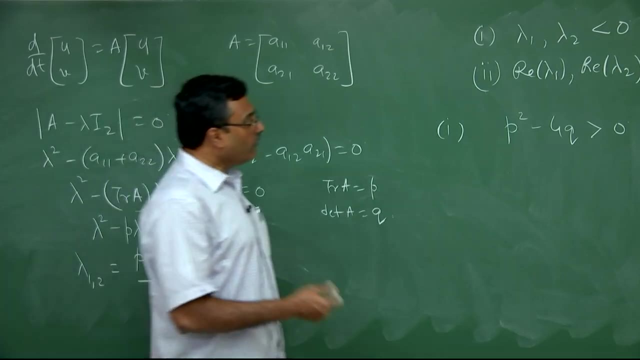 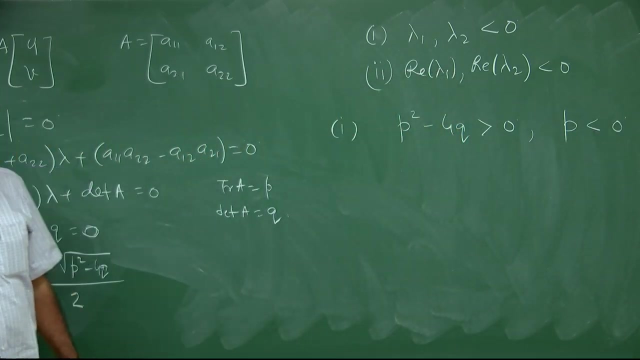 Yes, Right. how can you convince yourself? because if you take one point here on the p axis, that is 1 comma 0.. So what is p square minus 4q at 1 comma 0, that is 1, which is greater than 0, right. 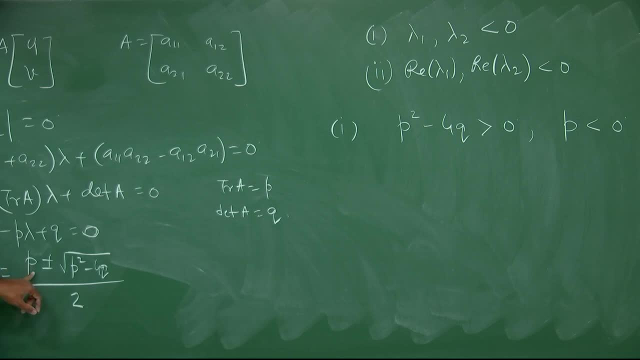 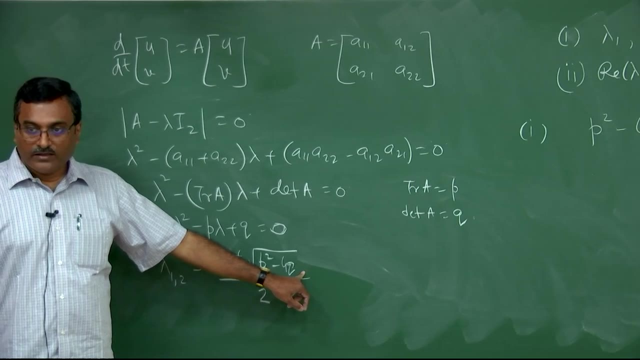 Similarly, if you choose a point inside this domain, that is say 0 comma 1 on q axis, then p square minus 4q is minus 4.. Yes, Therefore less than 0. therefore, within, that is, in the inside of this parabola, your p square. 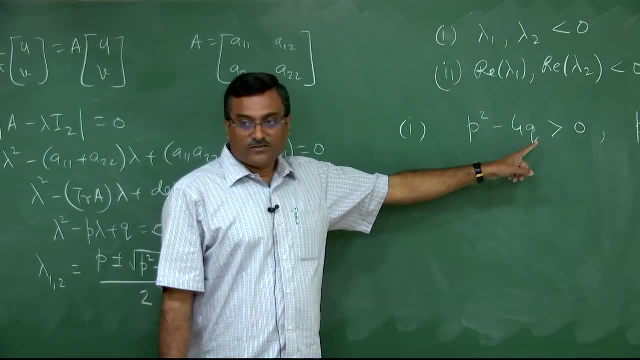 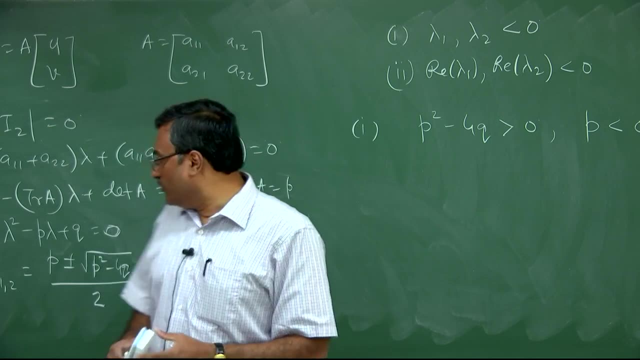 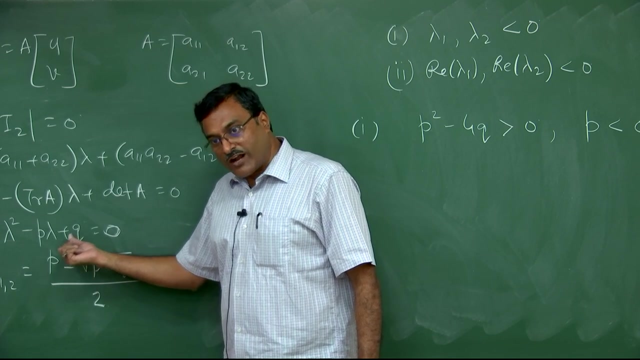 minus 4q less than 0. outside it is greater than 0. So here what you are having: that both the roots are complex conjugate with negative real part right. So it will be spiraling inwards. So if your p and q lying in this particular domain, you will be having this kind of situation. 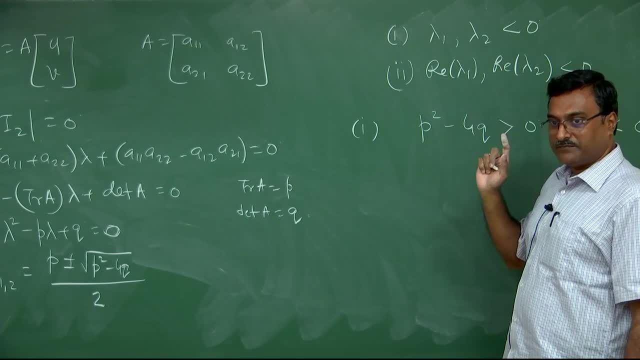 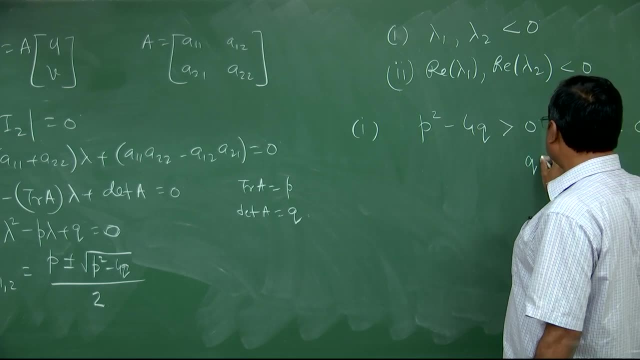 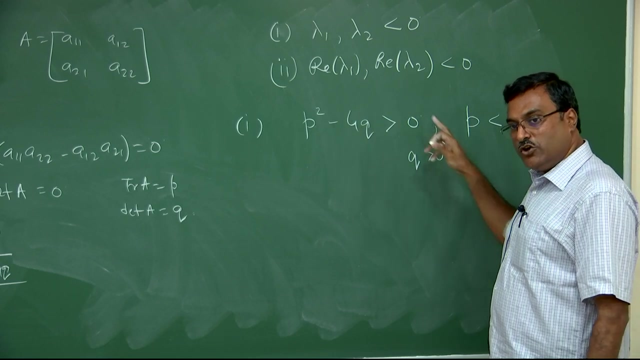 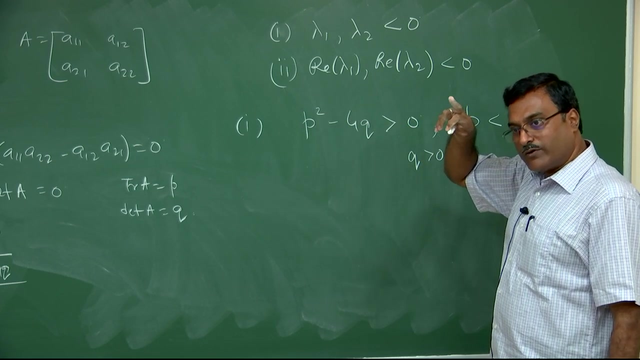 This kind of structure, face portrait here, right? Similarly, if you have your p q within this domain, then it will be: look like this one, but it is unstable, right, If you come out from the parabola. so, within this domain, what are the roots? both the eigen. 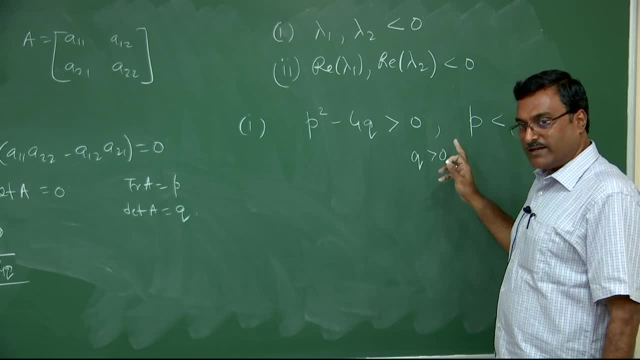 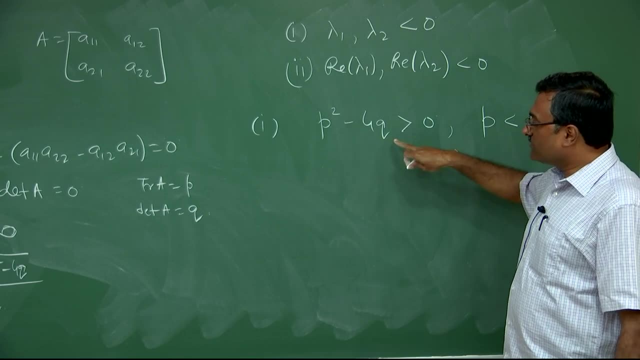 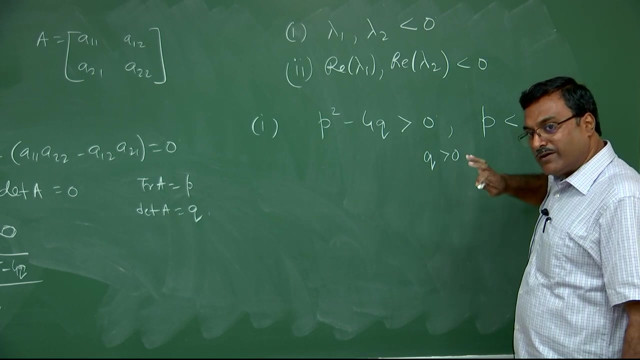 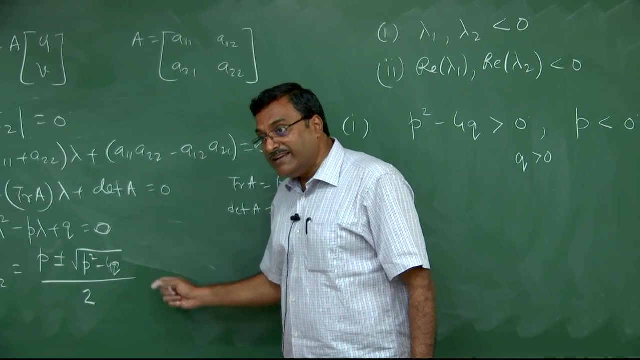 values are negative real numbers, So therefore, a typical format of the face portrait will looks like this one. So these are approaching towards this 0, 0, and here you will be having this kind of structure. this one, this one, this is away from the equilibrium. 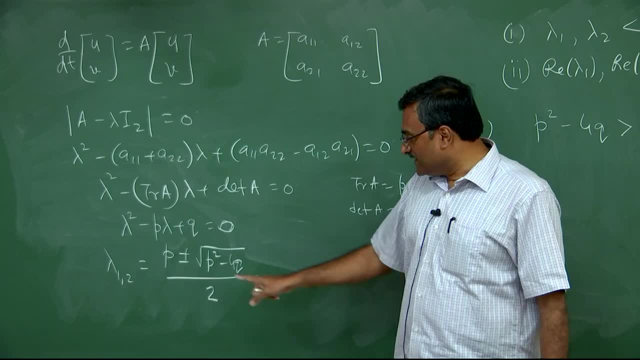 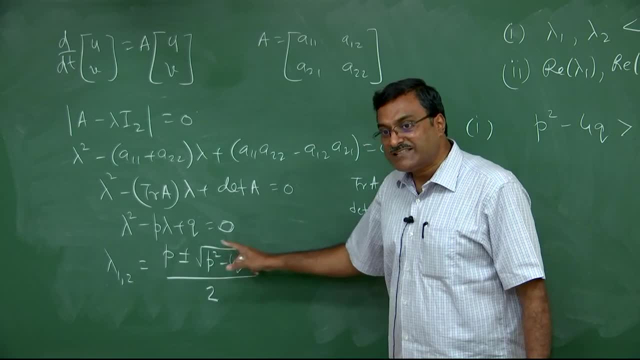 Now come out from the p and q etc in some particular domain, you will be having this shape portrait, cool right. And if you come from the parabola, which is some quarantine deine, for example, There will be changes in some content area, but you like the structure surface it will. 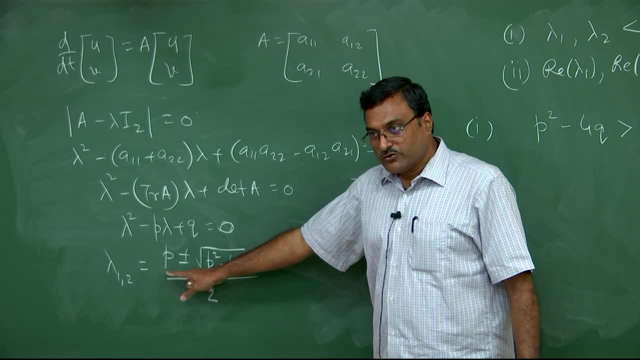 be defined as that. And the next point is that both these suits will have someinch opening surface. so you will see that there is some tension, some free spices To this. we will have a small p and q, so the force inside the space perde all those. 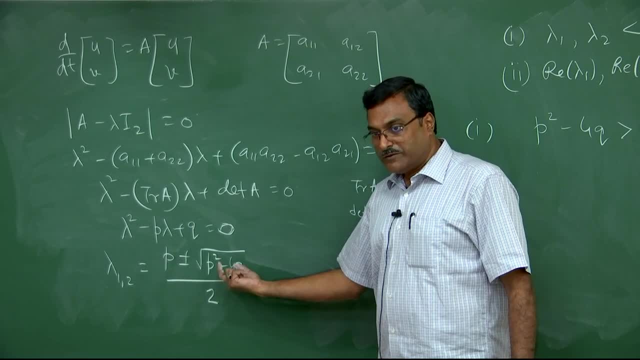 parts and do not bind it to the surface and vice versa. So all these, all other surface we take isn't strange. So you have some tension. This one say it is 90 degreeaton work, Then it is 90 degreeומiggerientos for this section, then after that would be creepy. 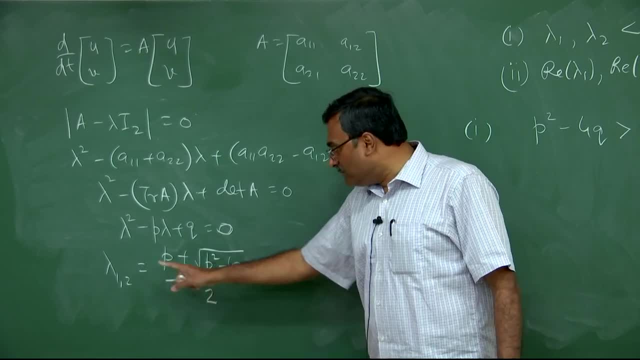 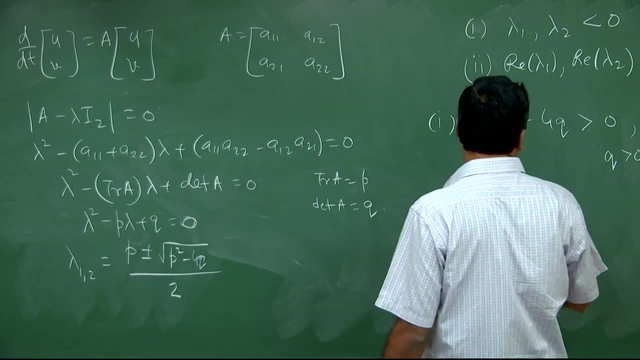 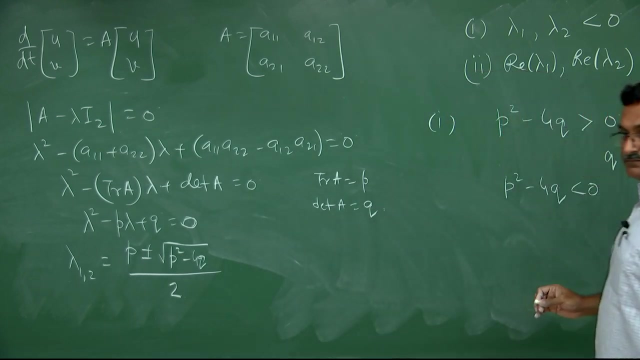 upon the fact whether magnitude of lambda 1 is greater than lambda 2 or magnitude of lambda 2 is greater than lambda 1.. So either this one or some topological equivalent form like this and also similarly here Now, what will be the last case? last case is that we have considered one more thing. 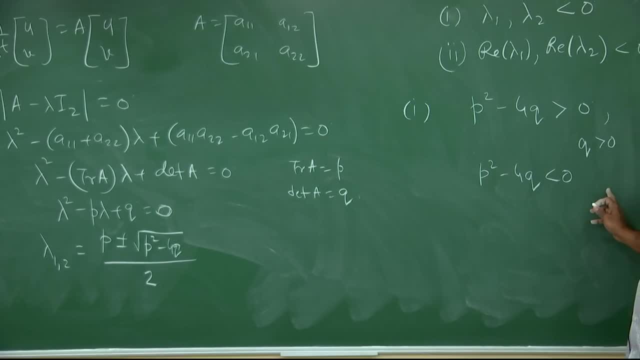 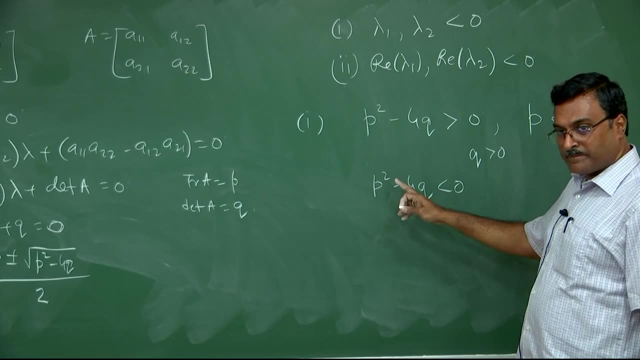 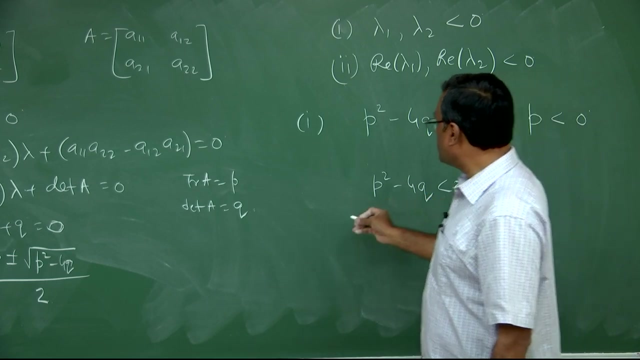 that you will be having concentric circles. where we will be having those kind of concentric circles? we will be having concentric circles on this vertical line. So if you take any p, q on this line, so that means your p equal to 0 and q is non-zero Once p equal to 0. 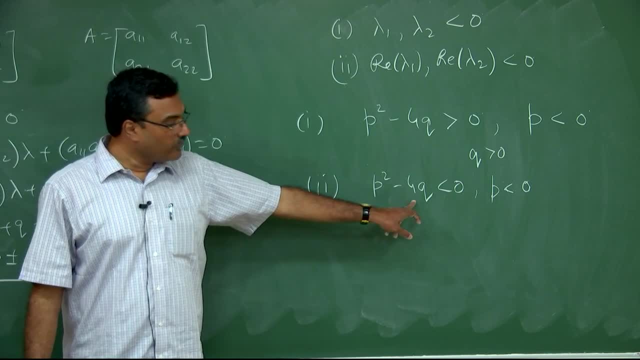 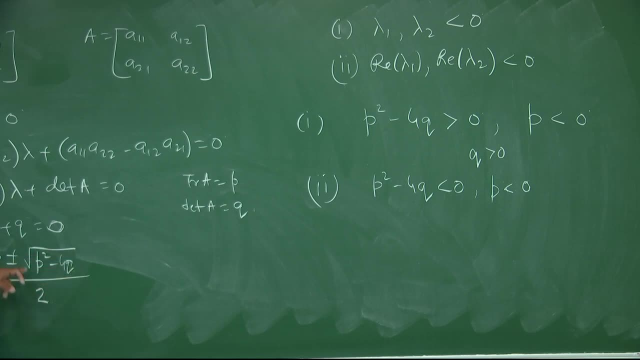 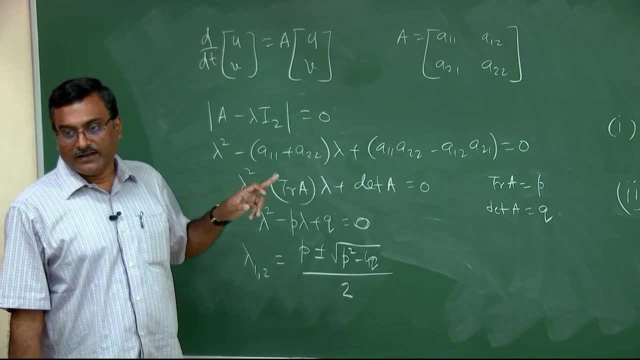 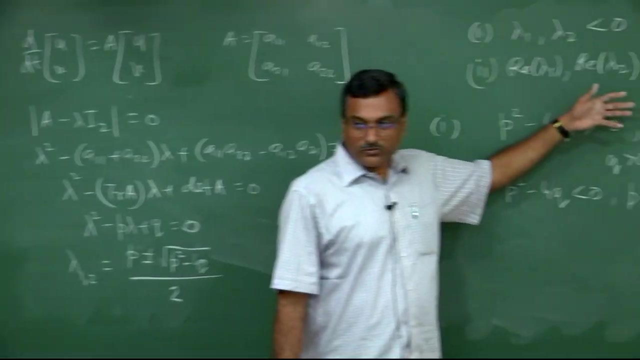 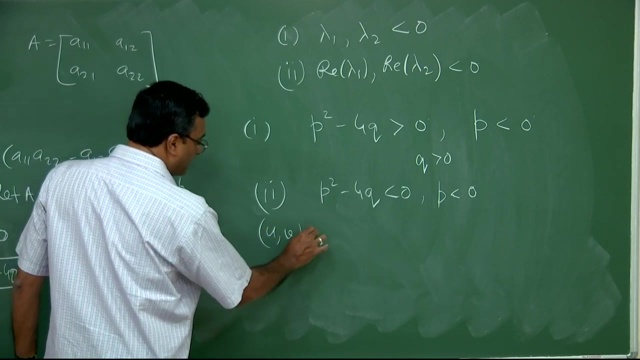 and q is non-zero, and also q is positive here above the line, above the line q equal to 0, so therefore you have purely imaginary, complex conjugate Eigen values. So on this axis you will be having phase portrait like this. So for a given two variable system you can linearize around the equilibrium point. then 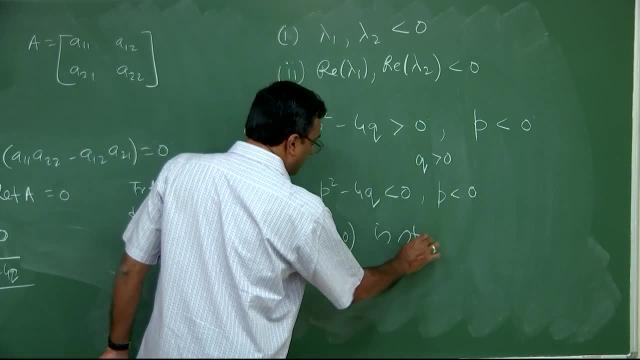 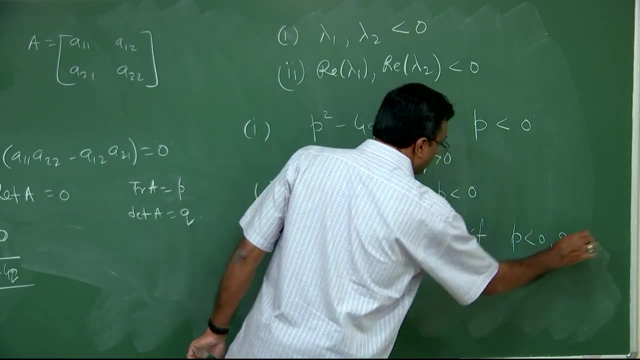 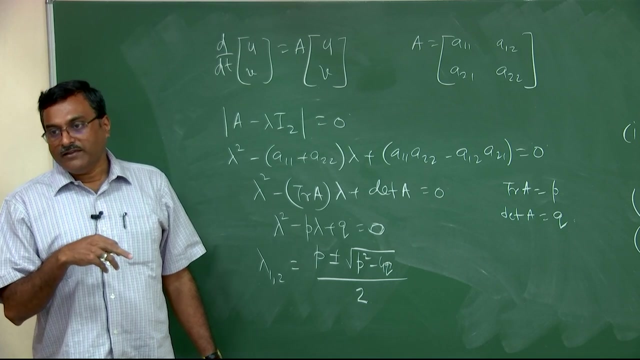 you will be having a system of linear equation. then you can immediately calculate what is p and what is q and depending upon the magnitude of p and q, you can try to judge where you are for the chosen values of p and q And accordingly you can understand how to calculate the p and q values. So this is the 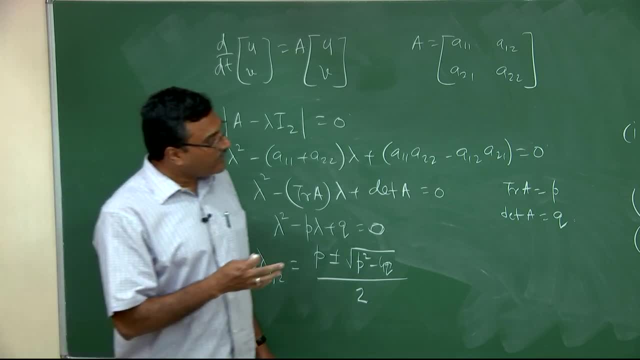 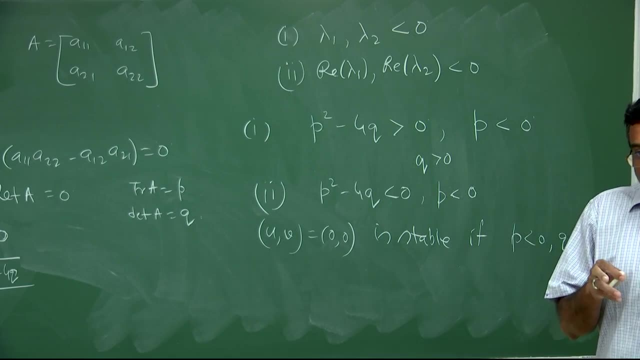 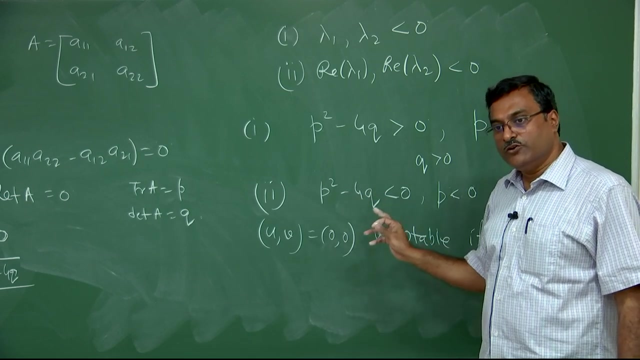 way how the phase portraits will looks like. Now the last point in this kind of relation between solutions for linear system and non-linear system. I will give you a particular example from where you can see that the behavior of the solution for the linear system will be matching with the behavior of the system for 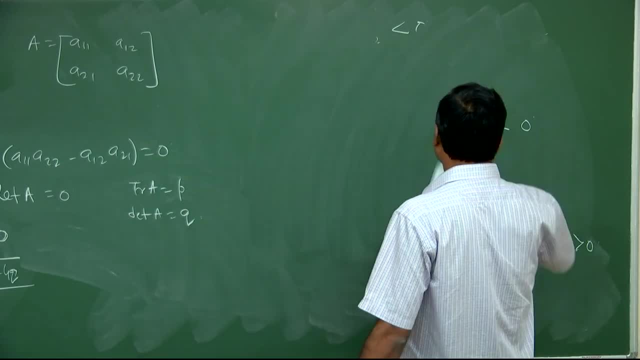 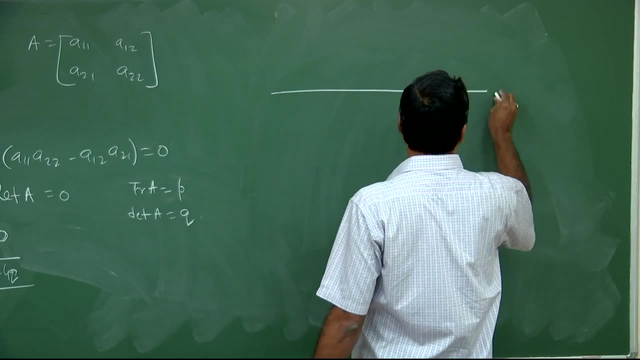 the non-linear system, Because we are judging the stability of the equilibrium point by using linear equation. we are using linear equation. we are using linear equation to create the situation. There is an important theory that is called Hardman-Grobman theorem. It says that you 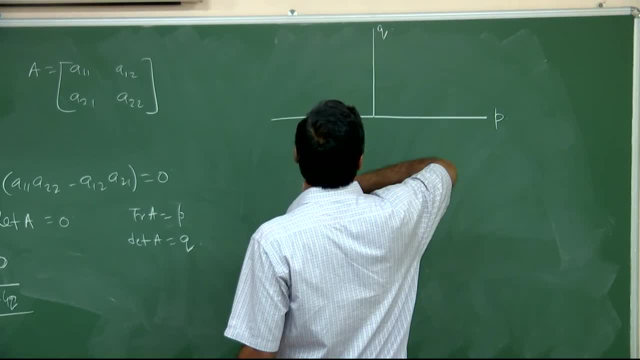 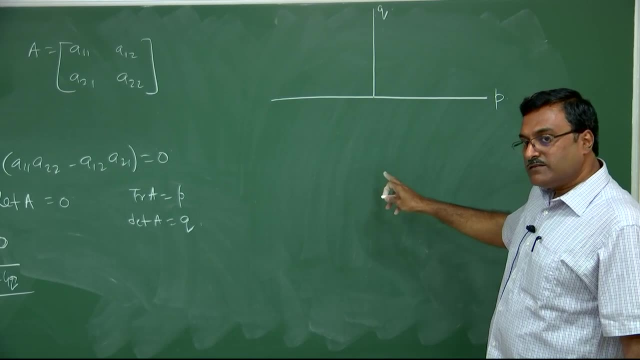 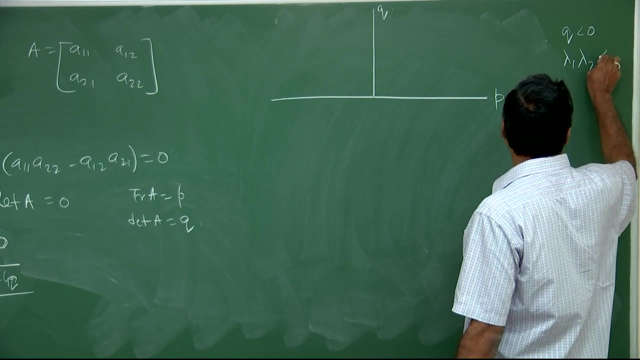 have an equilibrium for a given non-linear system, such that all the Eigen values of the linearize matrix having non-zero real part. If this condition is satisfied, that all the Eigen values have non-zero real part, so then solution trajectory of the non-linear. 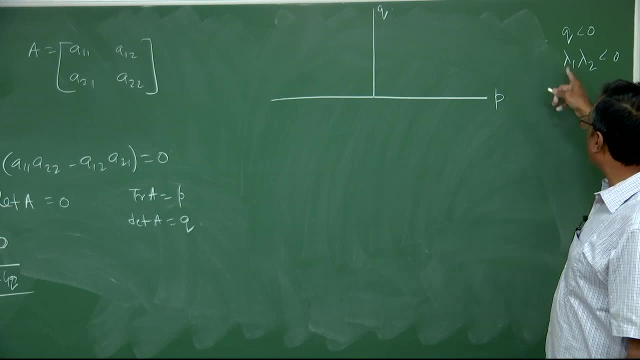 system near the equilibrium point by this matrix will be similar to the non-linear system. Okay, So all these equations are working. So what is the solution trajectory? Now I will. equilibrium point will be topologically equivalent to the structure of the solution trajectory near the trivial equilibrium point for the corresponding linear system. 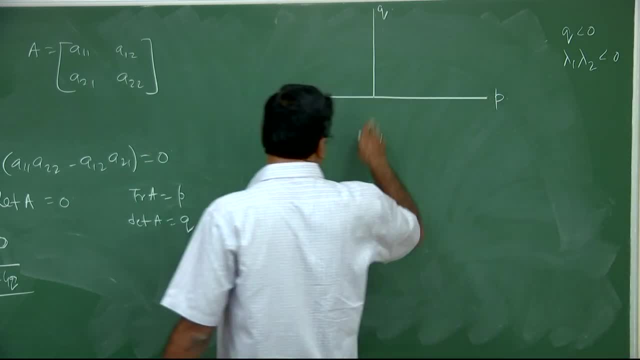 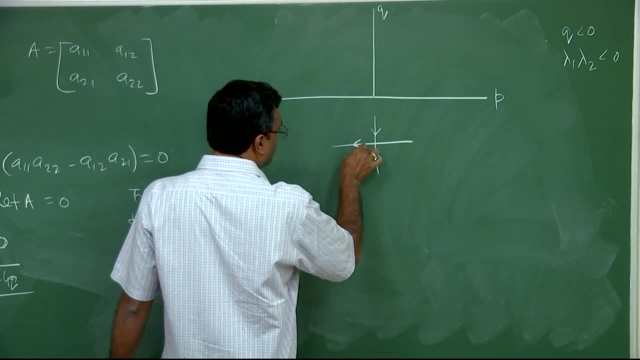 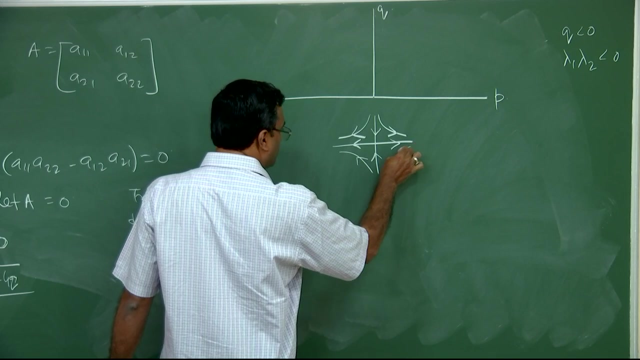 And there are very few examples which are available for which you can convince yourself that this behavior of the solution trajectories for the linear system and non-linear system. they are more or less identical. Now I will give you one specific example from where you can clearly visualize how these 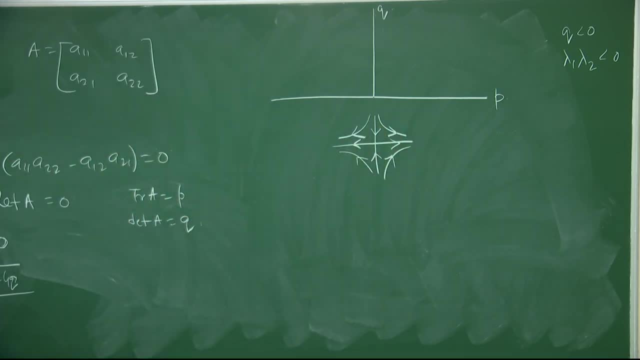 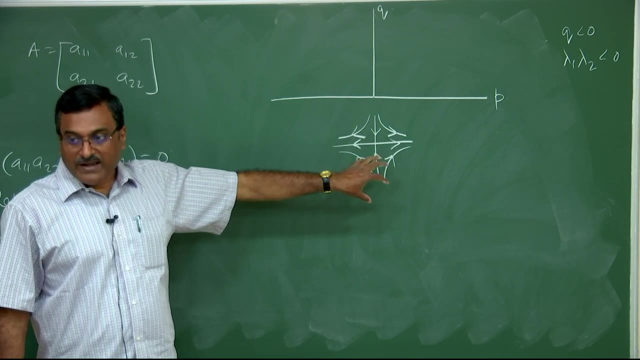 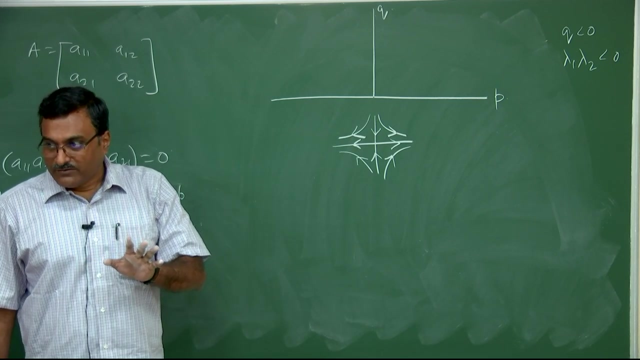 two linear and non-linear systems are seems to be equivalent near the equilibrium point and that actually justifies that this kind of theory can be applied for other higher variable system. But of course it is quite difficult to visualize that this kind of one-one correspondence between 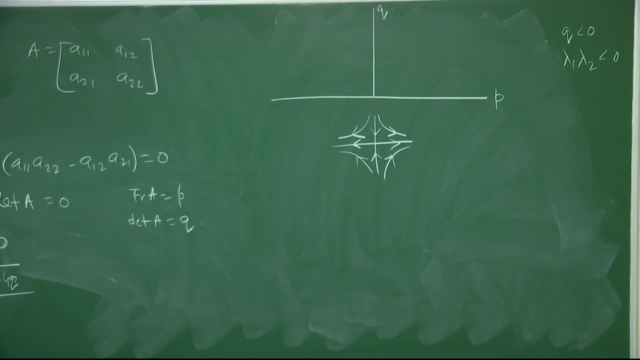 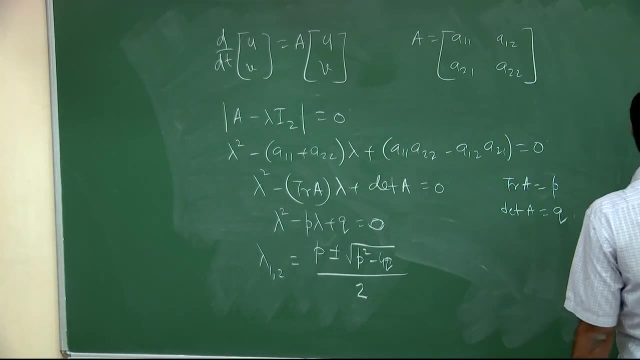 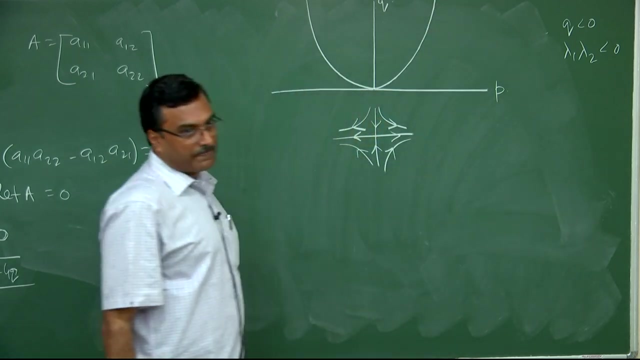 two system. rather, we need to depend upon the available theories to understand that Or mean, in order to convince our self. there are some possibility to make a one-one correspondence between the nature of the solutions near equilibrium point for a non-linear system, as well as corresponding 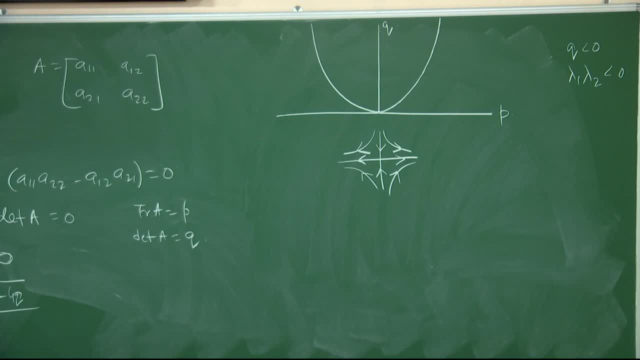 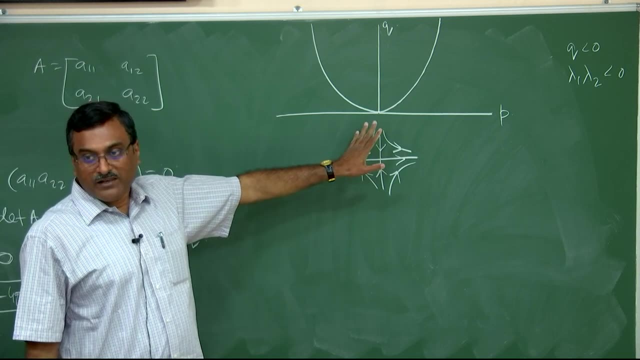 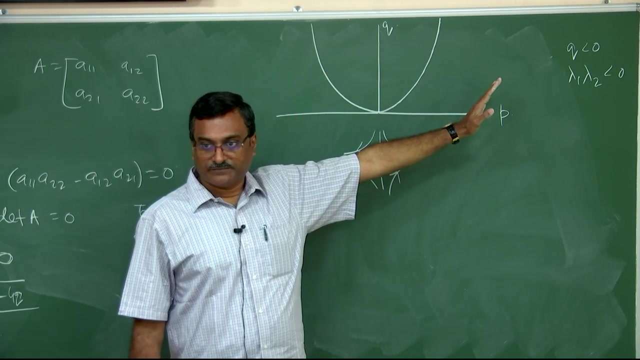 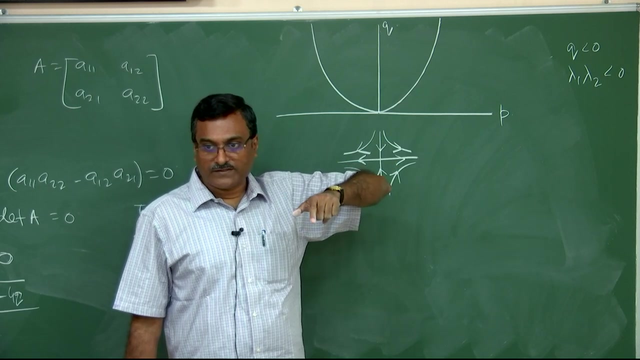 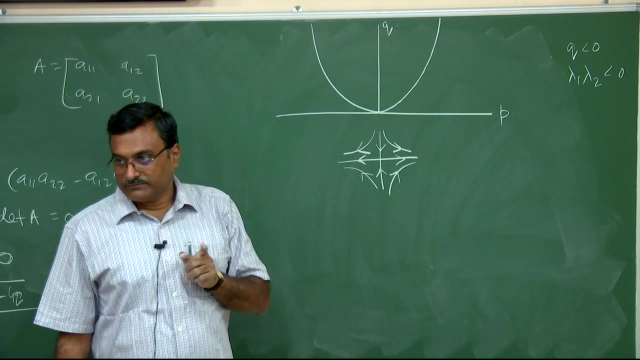 linearized version. So for that purpose we consider this simple system. So here we consider this system: X dot equal to X plus y square and y dot equal to minus. 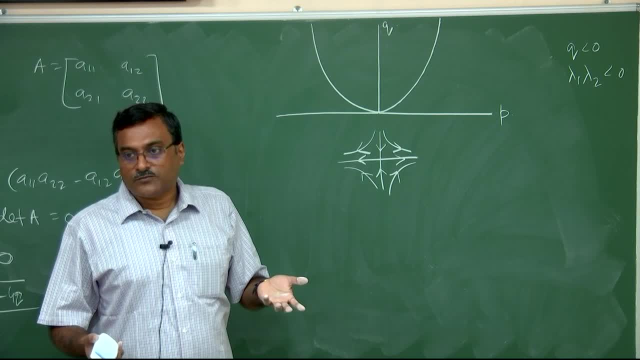 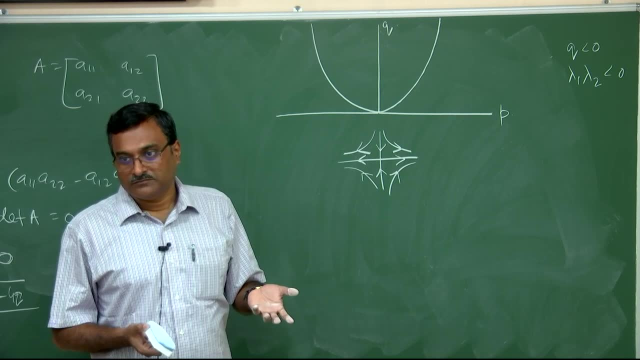 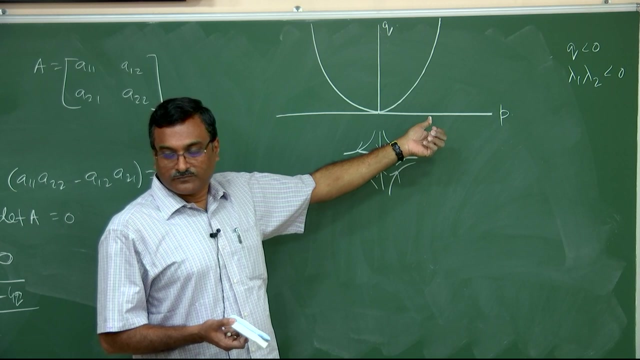 y. So I am considering this system only for the reason because I can show you that, although this is a coupled of a two coupled non-linear equation, still you can find out their solution explicitly. So, first of case, your x star, y star is 0 comma 0, this is the equilibrium point If we want to match. 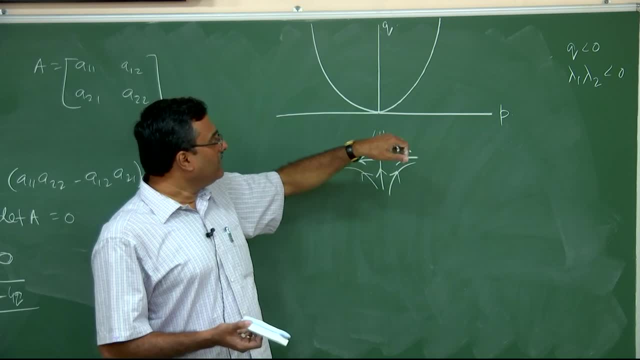 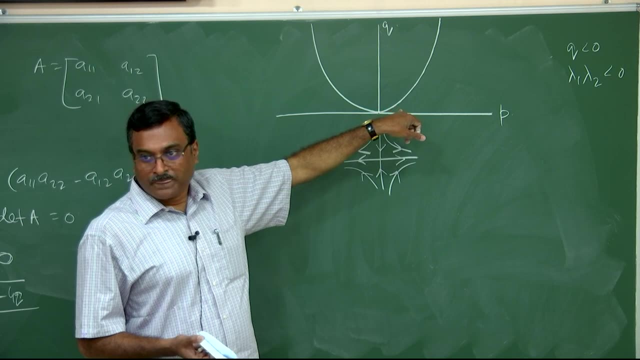 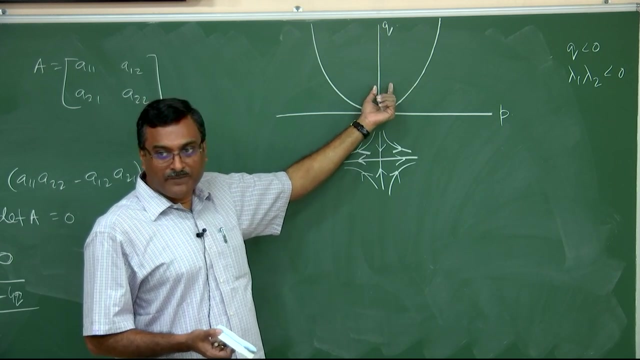 with the previous example, then you can understand that your f of x comma y, this is x plus y square, and g of x comma y, this is actually minus y. So therefore, if you calculate the matrix capital A, so therefore del f del x at 0, 0, this is 1. del f del y, that is 2y. 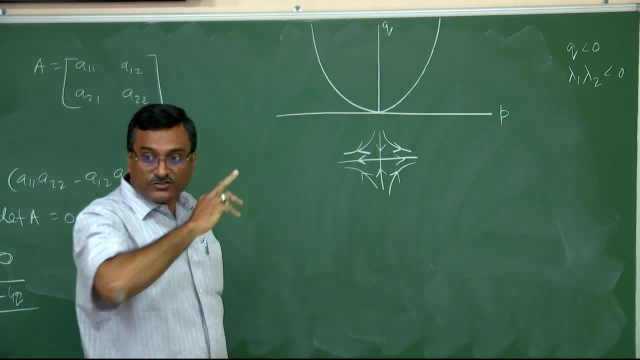 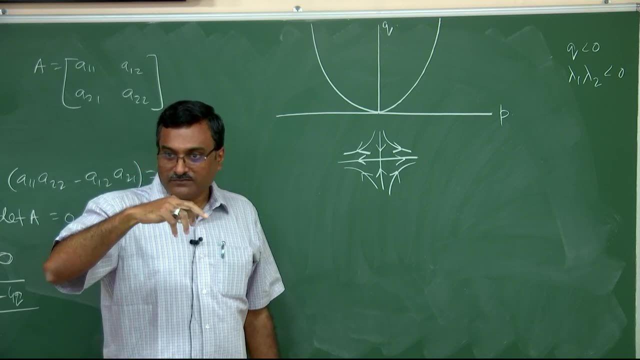 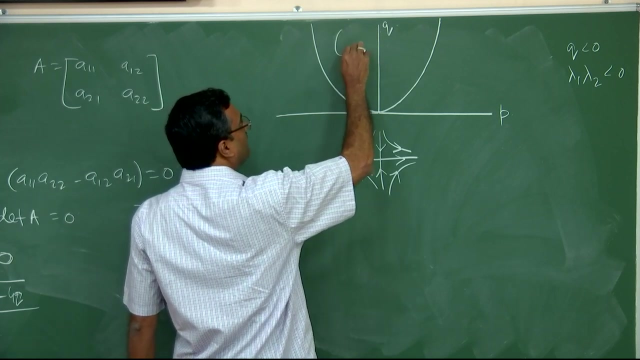 at 0: 0, this is 0, then del g del x, this is 0, and del g del y, this is minus 1.. Already, I have considered this type of problem earlier, correct? So what will be the phase portrait for the linear system? that is, u dot equal to u and. 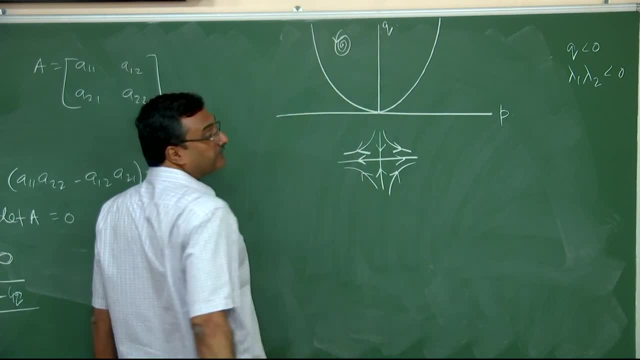 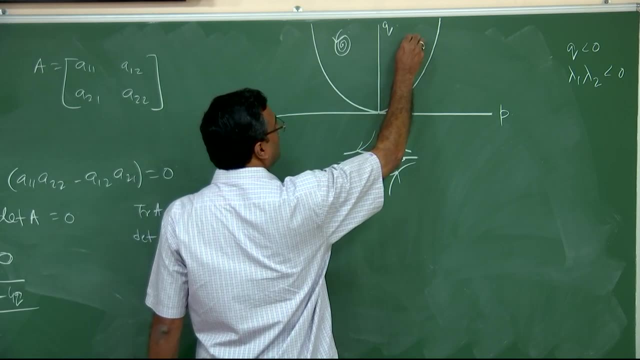 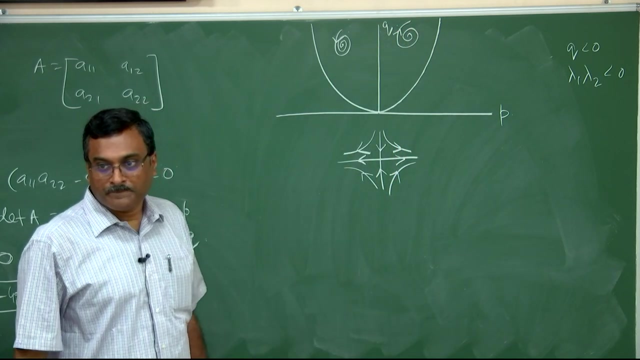 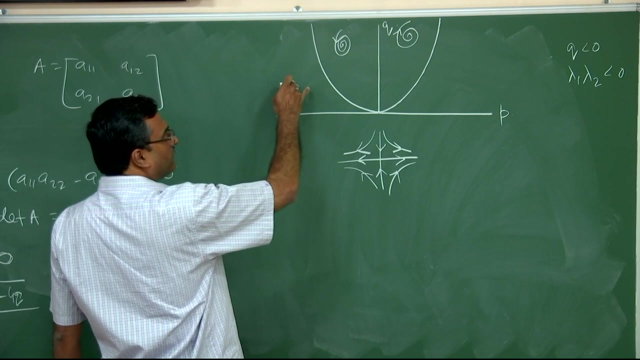 v dot that is equal to minus v V. In this case, face portrait will looks like: this is away from the origin. this is towards origin and therefore face portrait will looks like this one right Now. how to obtain the solution for the non-linear system: y dot equal to minus y. this gives: 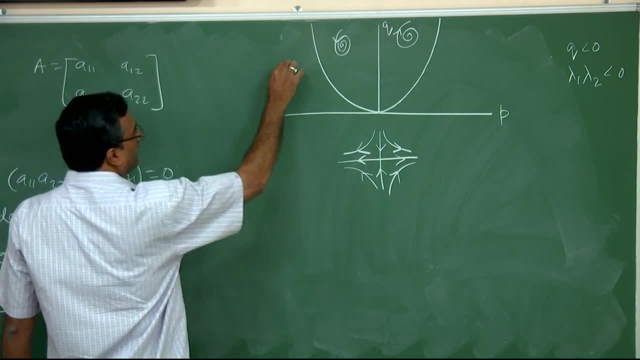 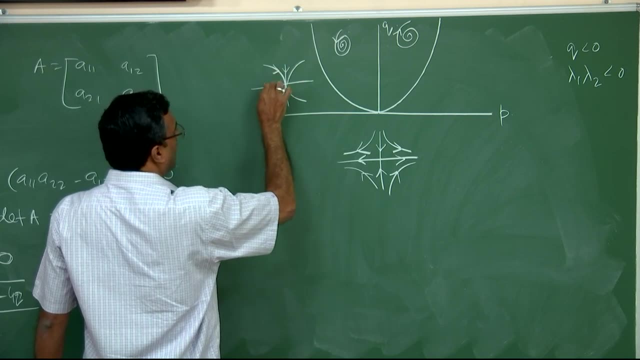 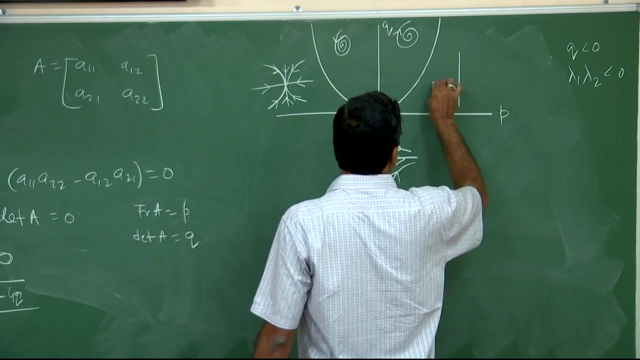 you the solution: y t equal to y 0, e to the power minus t. Then if you solve the second equation, first equation, that is x dot equal to x plus y 0 square e to the power minus 2 t. So this will imply that d d t of x e to the power minus t that is equal to y 0. 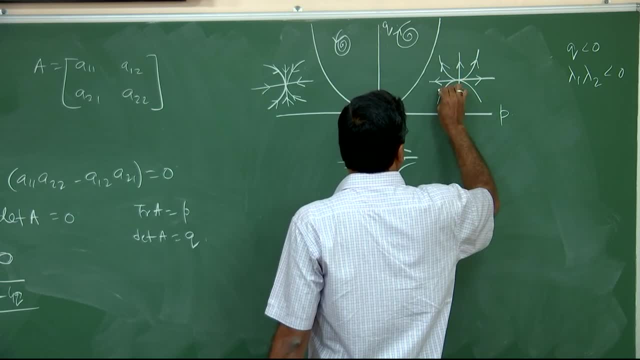 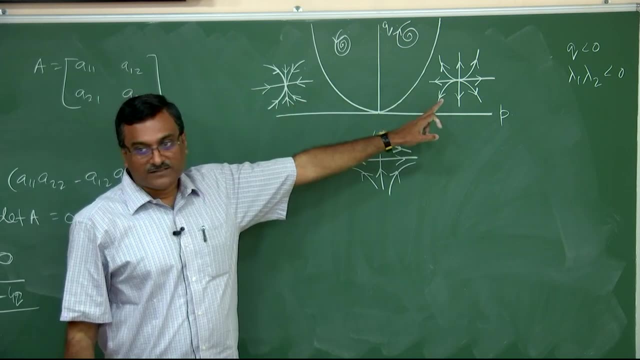 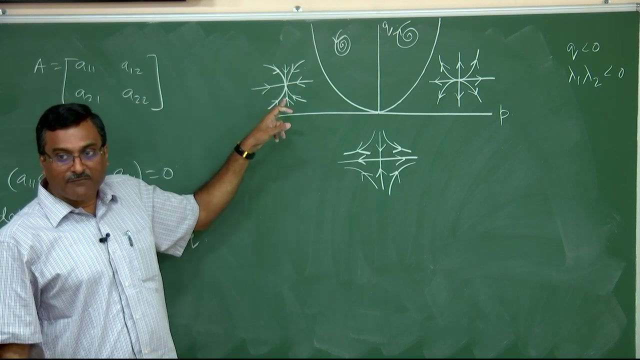 square e to the power minus 3 t, right? So therefore, by solving this equation, you can find x e to the power minus t. that is equal to some constant minus y, 0 square by 3 e to the power minus 3 t. Next, if you assume, 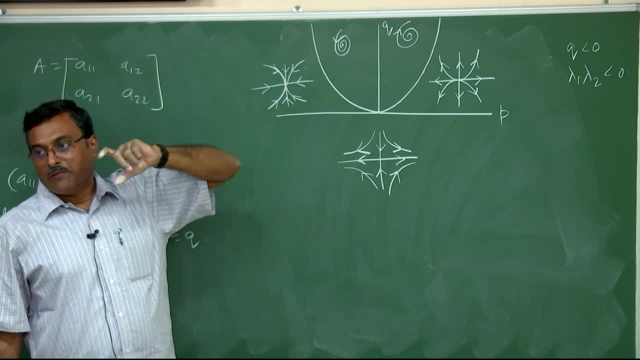 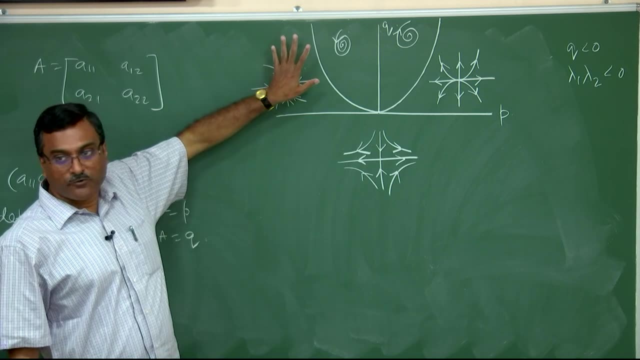 at t equal to 0, your x equal to x 0.. So therefore you can find x 0 plus y 0 square by 3, this is equal to c. Substituting back into this equation, you will be having x- t equal to. 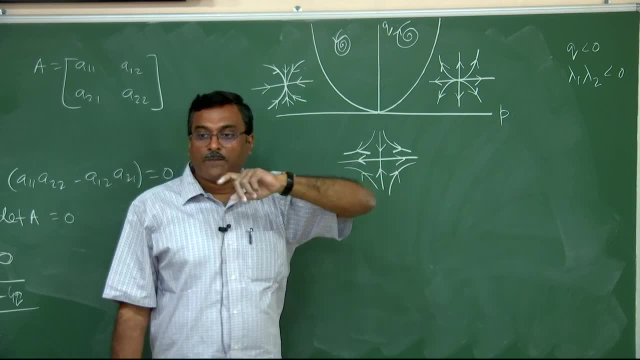 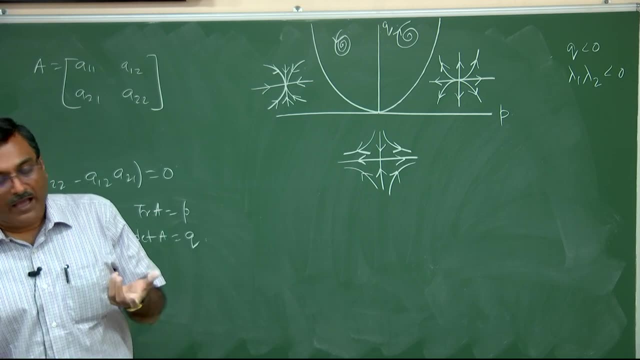 x 0.. So you can find x 0 square by 3 plus y 0 square by 3 times e to the power t minus y 0 square by 3 e to the power minus 2 t. So I am just substituting this value of c. 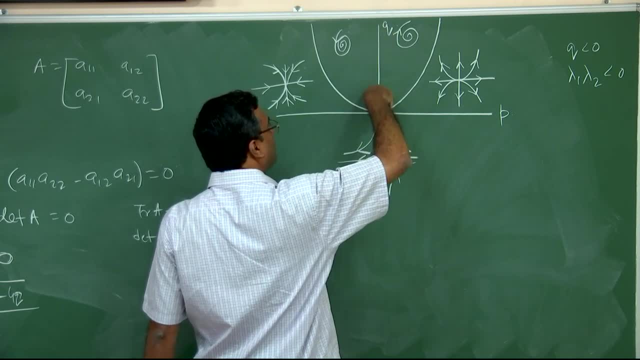 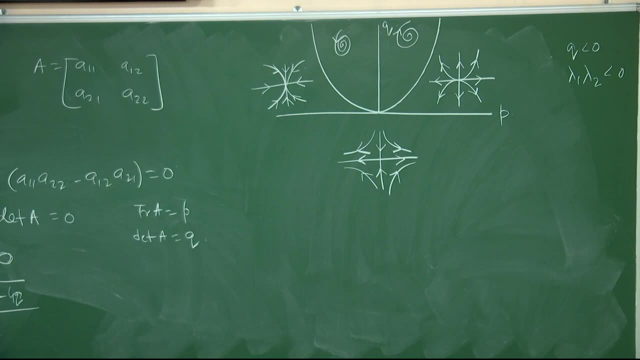 here and then multiplying both side by e to the power t. right Now, once you have this structure, then you can just write down the solutions in this format: y 0 square by 3 times e to the power t minus y 0 square by 3, e to the power minus 2 t and y t, this is equal. 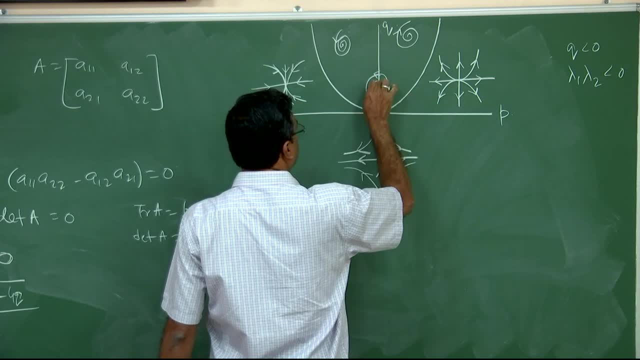 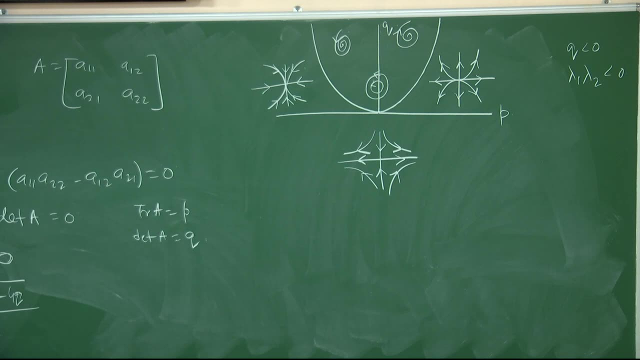 to y 0, e to the power minus t. Now, in this case, first of all, if you choose your initial condition, as y 0 is equal to 0.. If you choose y 0 equal to 0, so that means 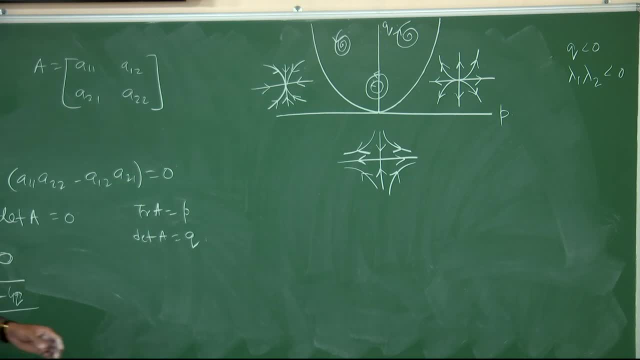 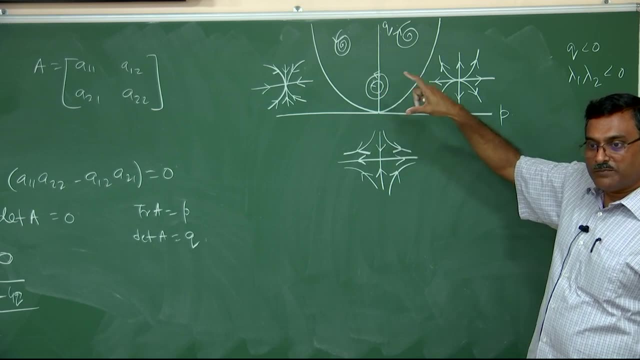 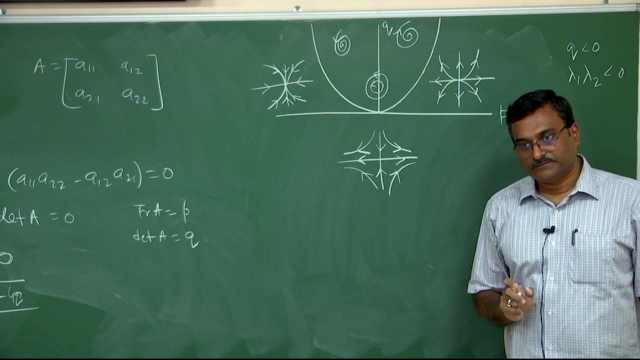 your solution is comes out to be x t equal to x, 0, e to the power t and y t. this is equal to 0. So that means you are starting from a point on x axis and it shows that solution will remain always on x axis, correct: x t equal to x 0, e to the power t. So that means 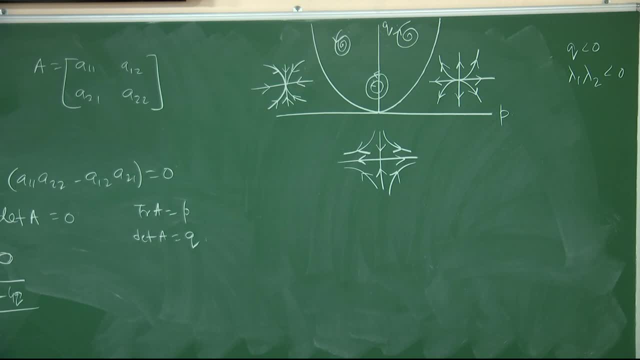 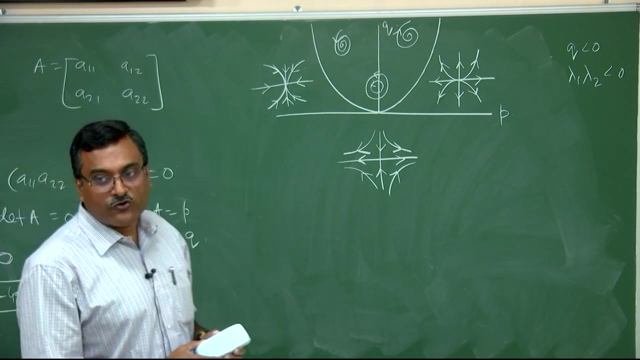 as t tends to infinity, solution trajectory will be approaching to either plus infinity or minus infinity, along x axis, depending upon whether your x 0 is positive or negative. So therefore, on x axis, you will be having this kind of behavior along this direction, if this is your origin right. So, along this line, solution will be diverging to plus infinity. 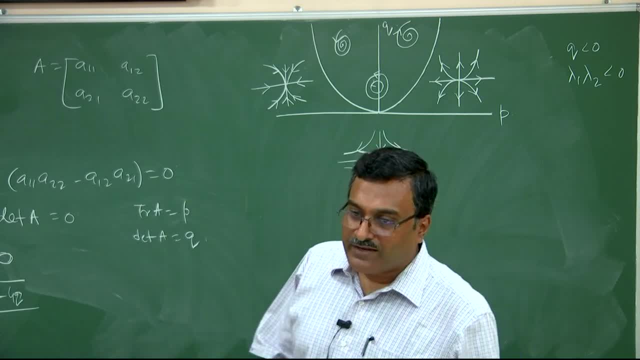 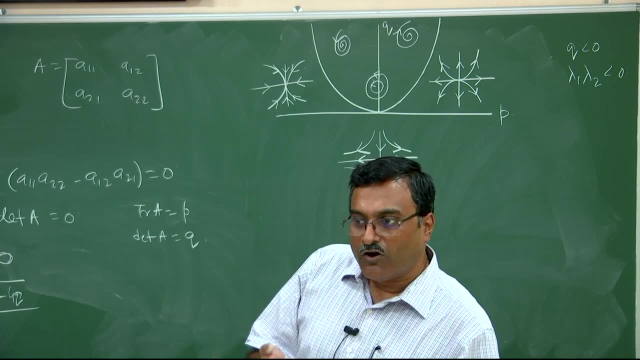 Next, if you choose the initial condition in a little bit clever way, that is, you choose your initial condition, that is x 0 plus x 0, that is plus infinity. So that means you y 0 square by 3, this is equal to 0.. Why I am considering this is equal to 0? Because 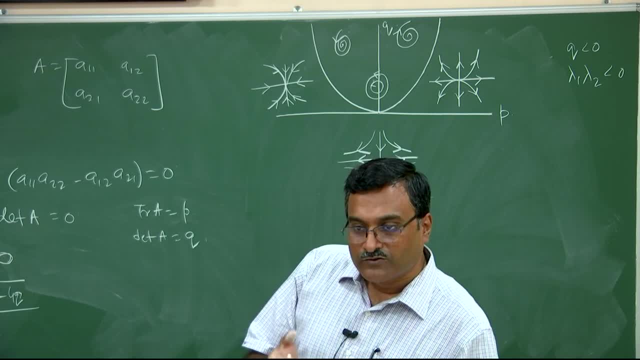 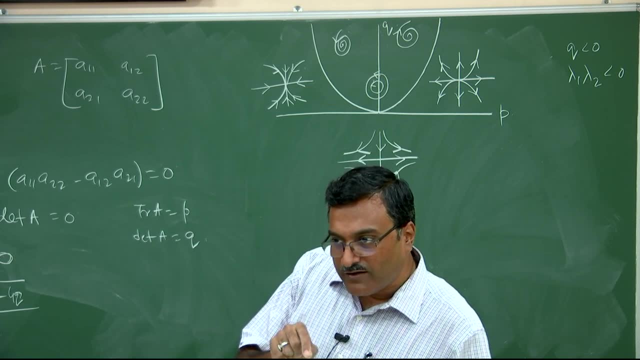 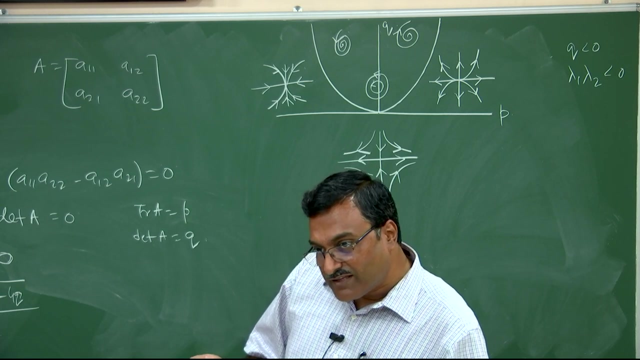 now I want to see that if is it possible to find out one curve along which solution trajectory will be approaching towards the origin. So in order to do that, I need to consider the coefficient of exponential term having positive factor of t. that coefficient should be equal. 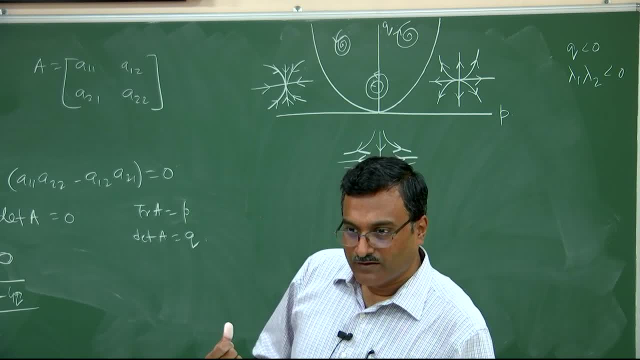 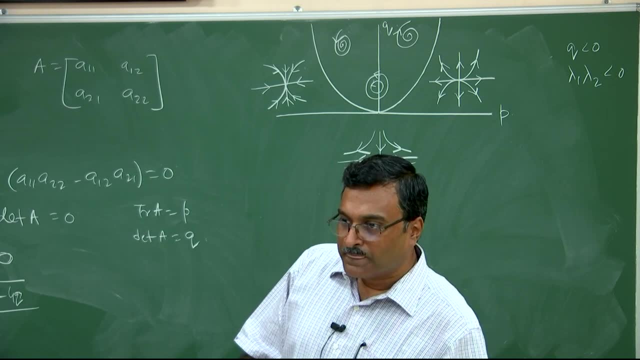 to 0.. So here you have e to the power t. so that is why I am considering x: 0 plus y 0, square by 3, equal to 0.. If you consider this one, then what is the structure of your solution? 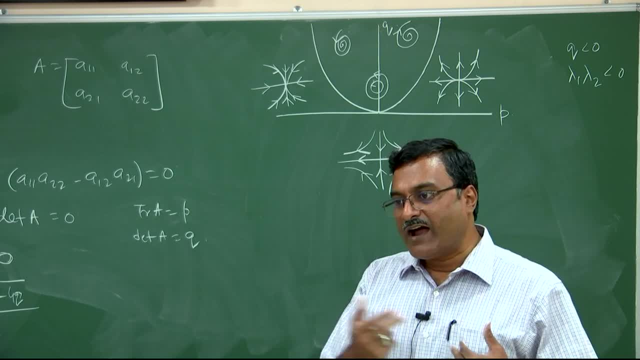 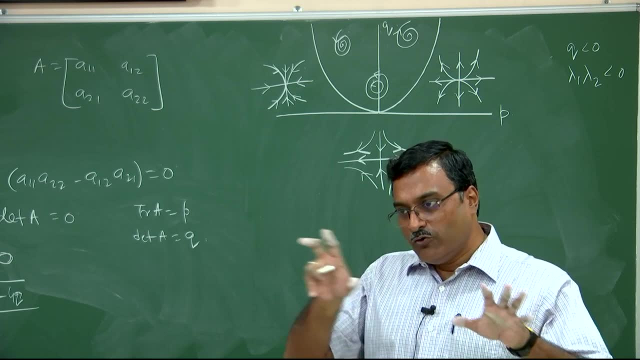 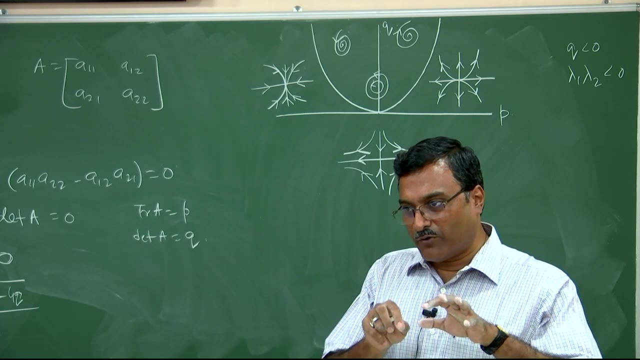 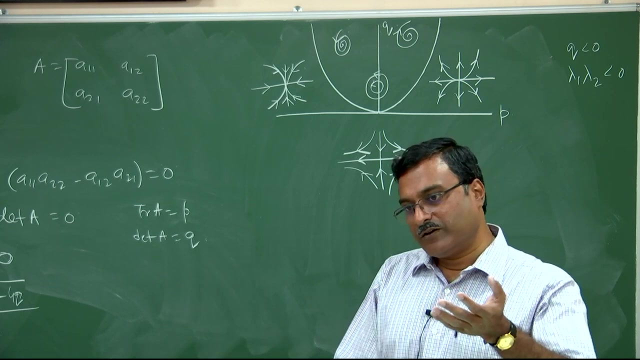 The structure of your solution comes out to be that x t- this is equal to minus y 0, square by 3- e to the power minus 2 t and y t- that is equal to y 0, e to the power minus t, correct? Now, if you eliminate y 0 and e to the power minus t from these two equations, then you: 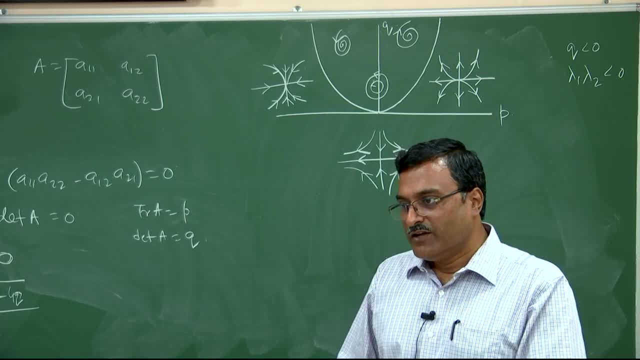 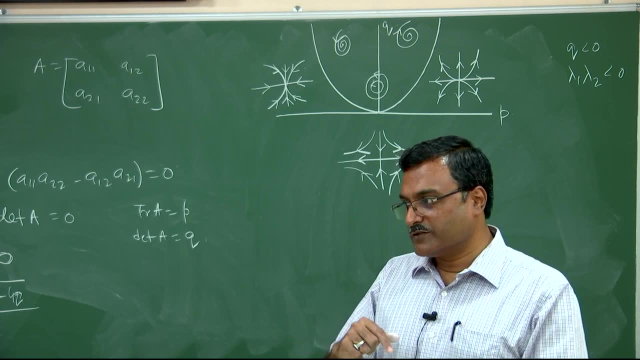 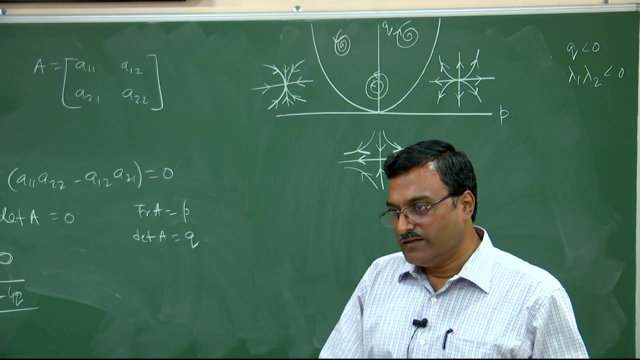 can verify that you will be having actually this particular curve: x 0 plus y 0 square by 3.. Because if you make it square, so this will be y 0 square by 3, e to the power minus 2 t. then if you add them, then you will be having this one. So now just try to understand. 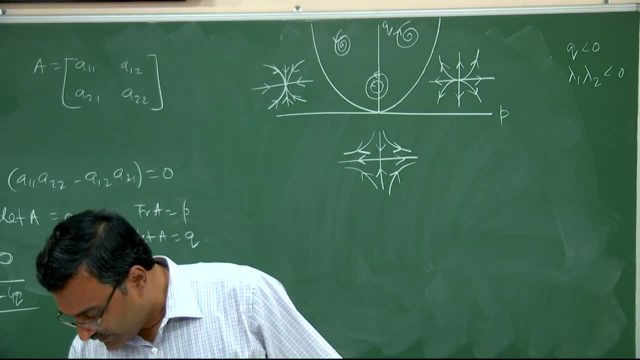 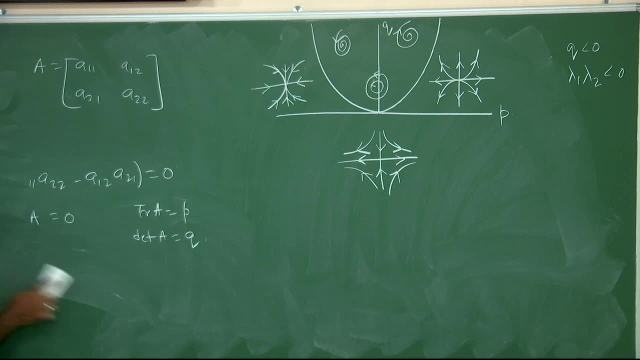 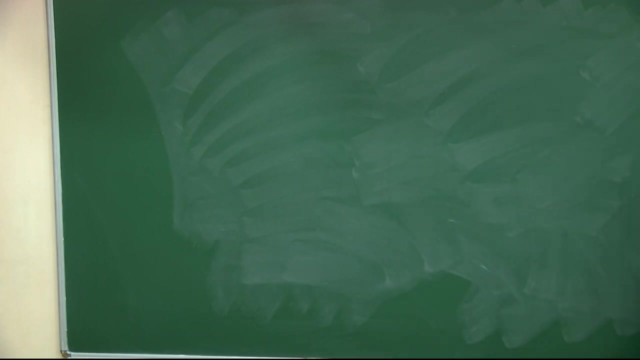 what is the beauty of this problem? You are choosing your initial condition like this. so that means your initial point x 0, y 0 lies on this particular curve, correct, and accordingly your solution trajectory is that curve itself: x plus y 0, square by 3, and this is a parabola. 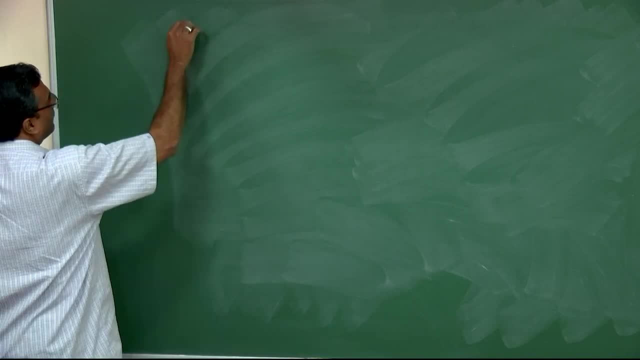 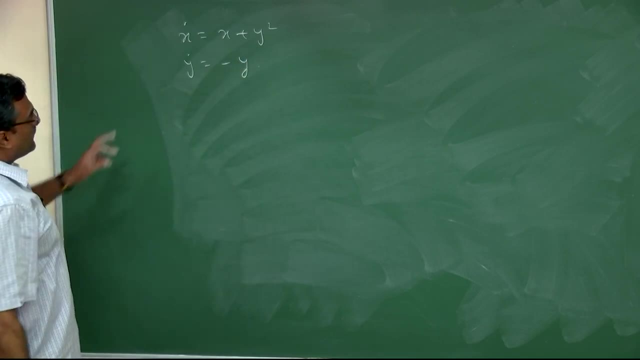 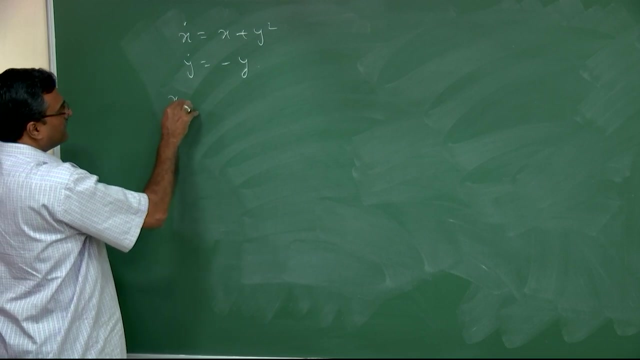 like this. So along which solution trajectory will be approaching to the origin and rest of the trajectory? they will looks like this one, this one, This one and this one correct. and now try to understand then this and that particular phase portraits. they are topologically equivalent. 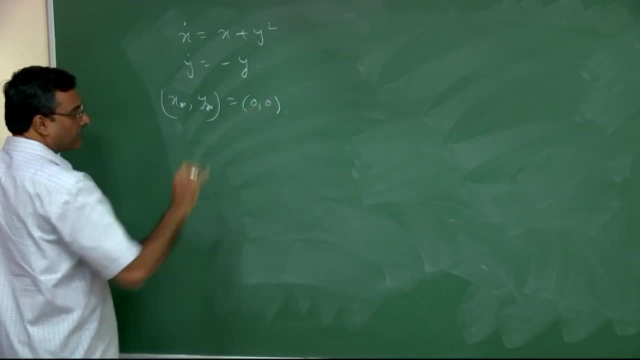 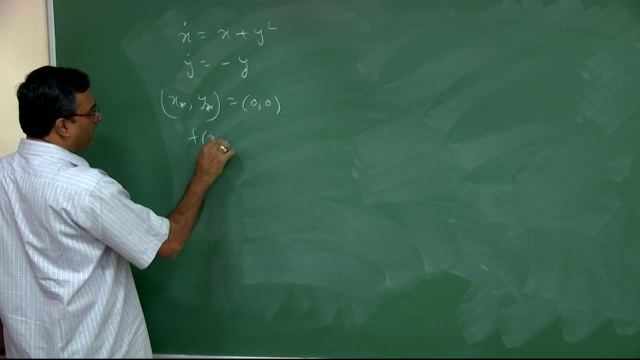 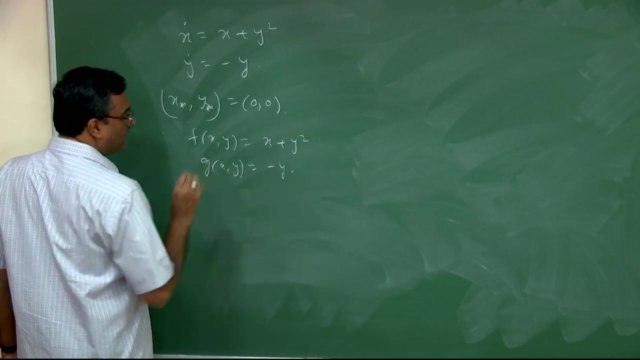 So what is happening here? that this line remains horizontal and the vertical line. this is actually stretched. in a way, it will be constructing this curve- x 0 plus y 0, square by 3, equal to 0, and rest of the trajectory will be stretched accordingly in order to have 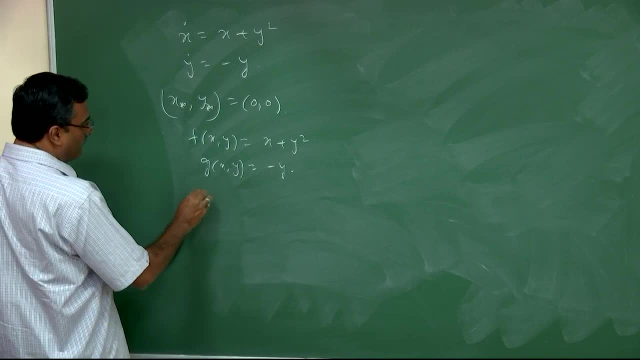 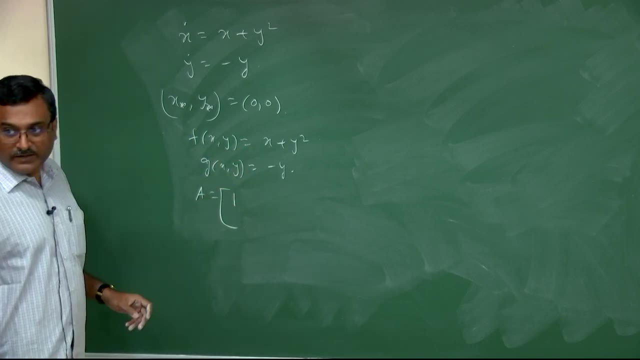 this kind of structure. So if you consider a very small vicinity of the equilibrium point for this non-linear system and this phase portrait, probably you can convince yourself that they are topologically equivalent. So in order to understand the stability behavior of this point, if both the 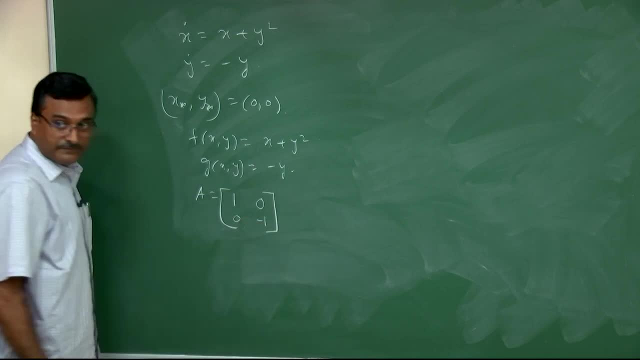 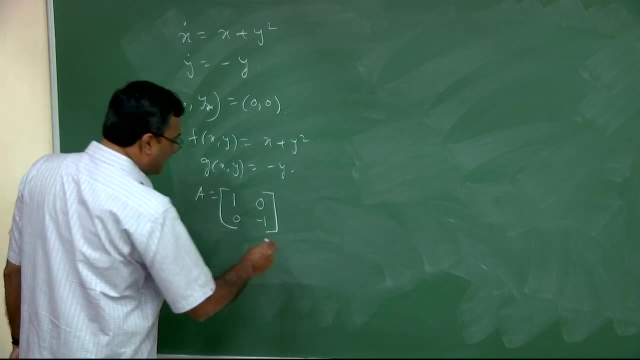 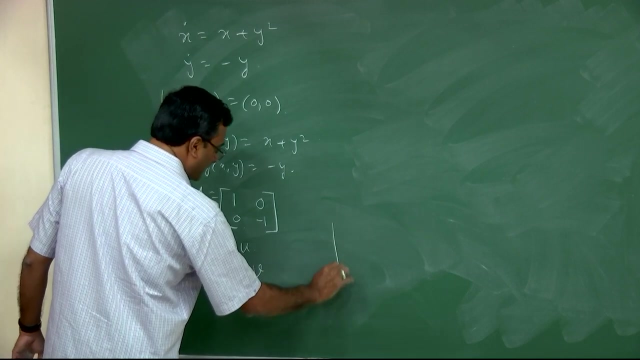 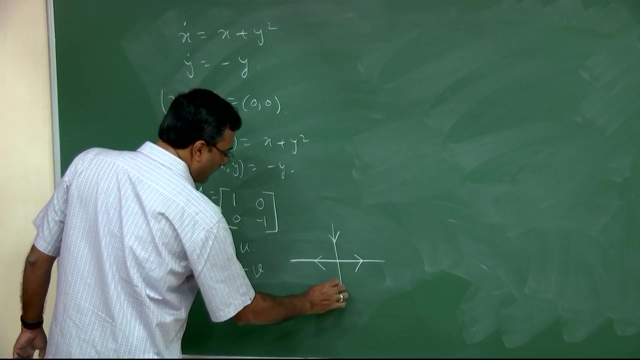 Eigen values are either non-zero or having non-zero real part, then the corresponding linear system will give you the nature of the solution trajectory nearby the equilibrium point. Last, I will just give you a simple idea of the global stability for a non-linear system with a specific example, but of course in the next lectures I will be coming back to 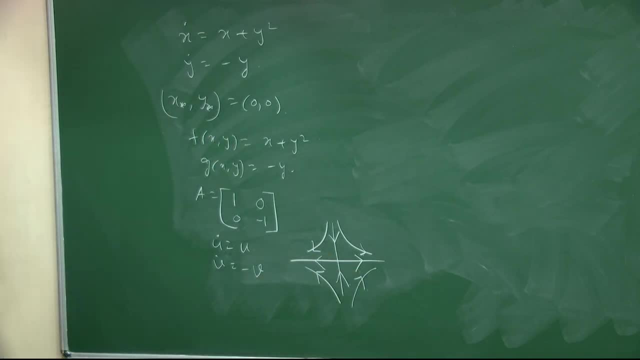 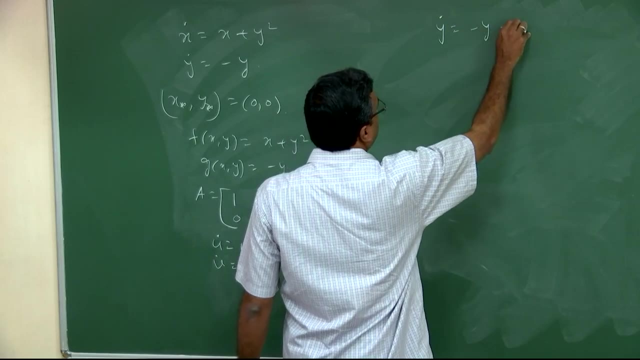 same system because this is a simplified version of an well known single species population model. So this is a non-linear system and I am considering this problem within the domain X greater than x equal to 0, because I will explain you that how this is related with some population model. 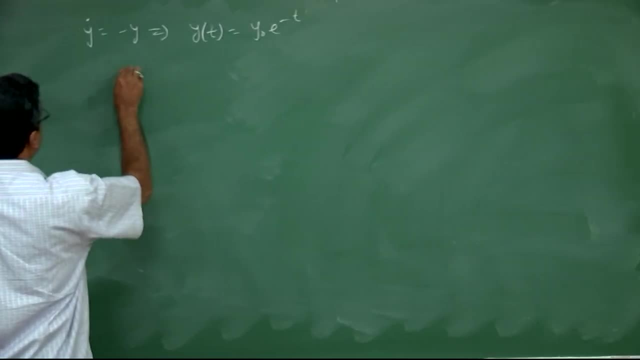 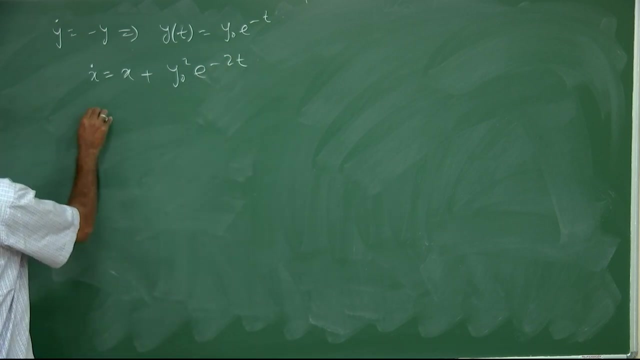 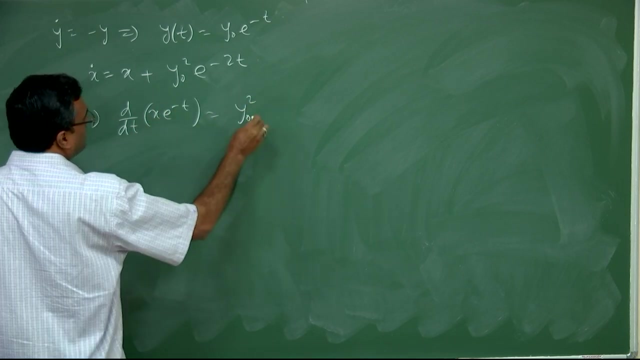 and in order to make it make a appropriate sense for this problem. so x happen to be positive. Now it has two equilibrium points, that is, x 1 star equal to 0 and x 2 star is equal to 1. correct f dot x for this problem will be equal to 1 minus 2 x. So from linear stability, 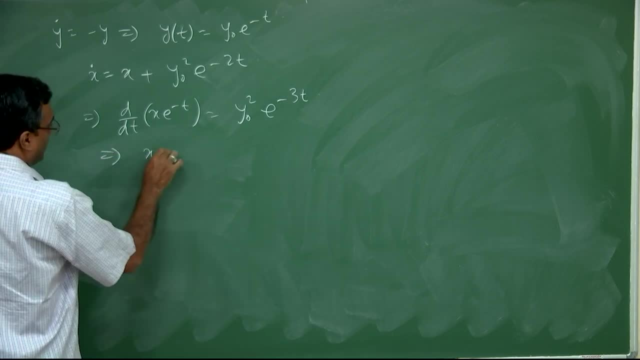 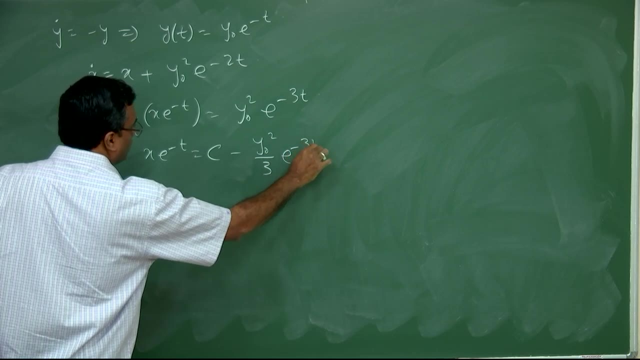 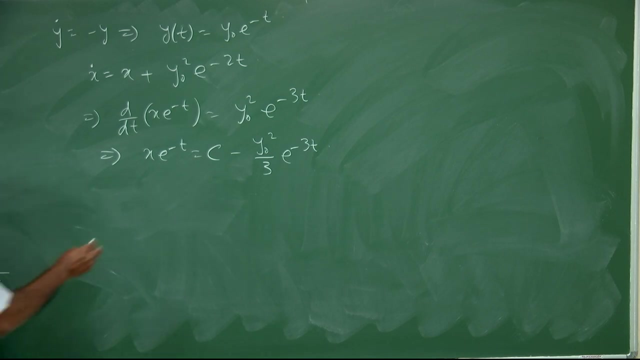 analysis: at 0, this is positive, at 1, this is negative. So therefore, x 1 star equal to 0 is locally unstable and this is locally stable. Now the point is that we can prove that if we start from any point x greater than 0, then all the solution trajectory will. 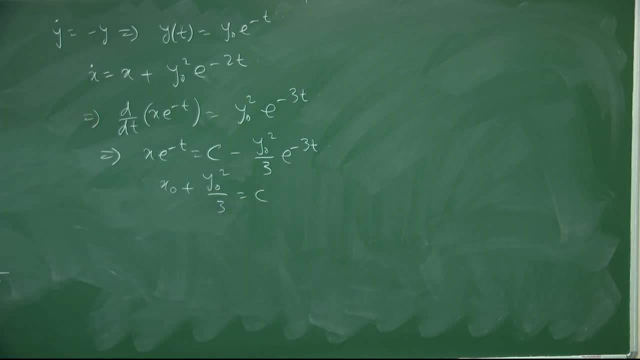 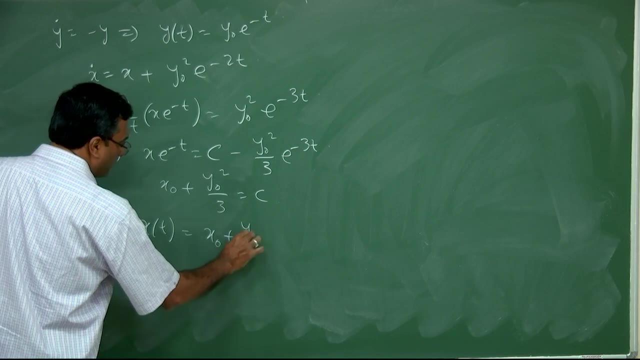 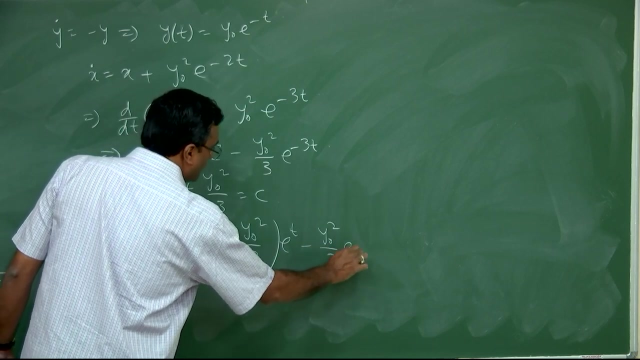 be approaching towards this equilibrium point by constructing a Lyapunov function. So Lyapunov function means you need to construct a positive definite function Which is positive, definite except at the equilibrium point. and it is time. derivative should be negative definite except the equilibrium point. If this is satisfied, these two conditions. 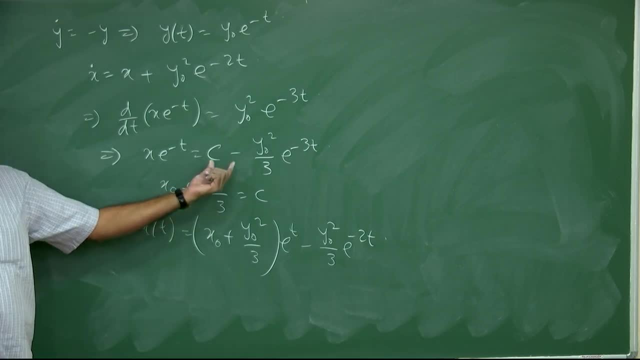 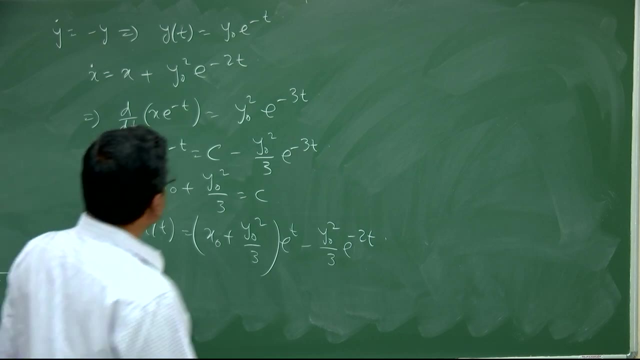 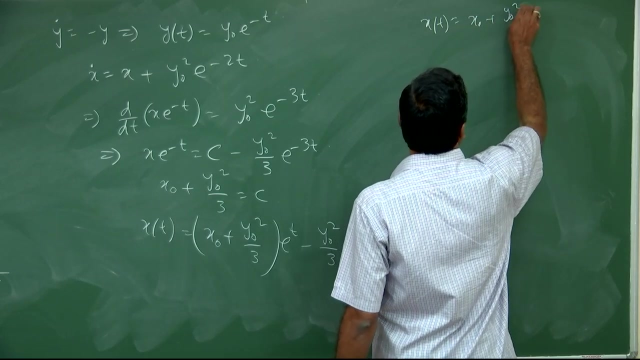 are satisfied, then we can say that particular equilibrium point is globally asymptotically stable for the given system. So for this problem I can construct this V as x minus 1 minus ln x. So what is the general format for this kind of linear? 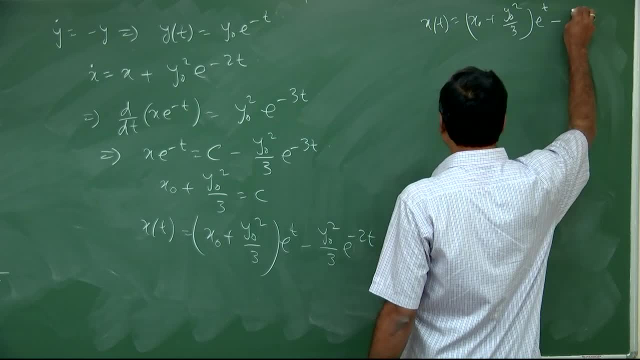 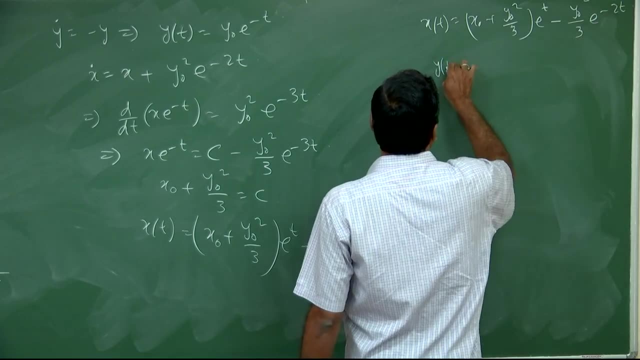 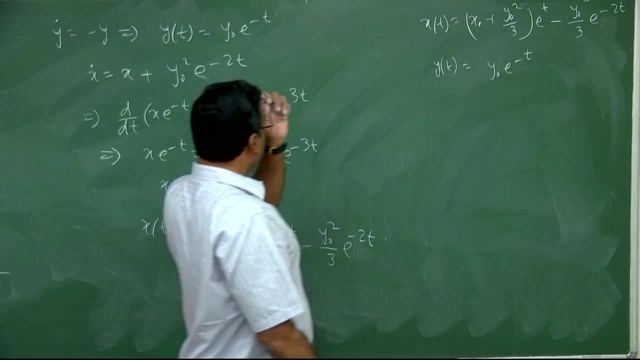 Lyapunov function. general format for this type of linear Lyapunov function is x minus x star minus x star, ln x by x star. but you should keep in mind there is no unified way by which you can construct a Lyapunov function for the given system. It is rather a some 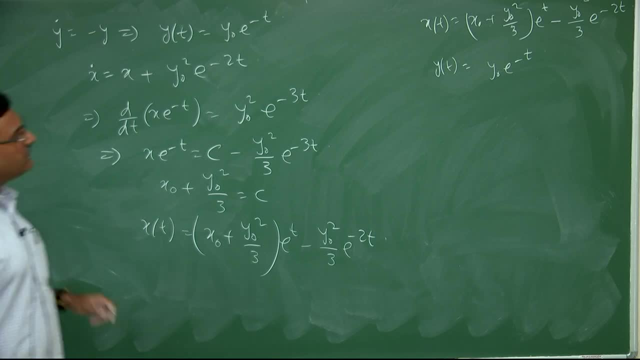 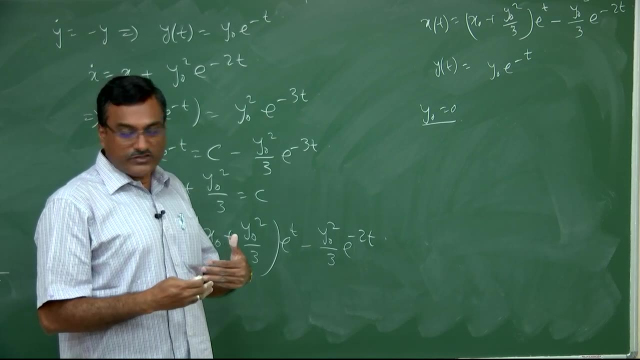 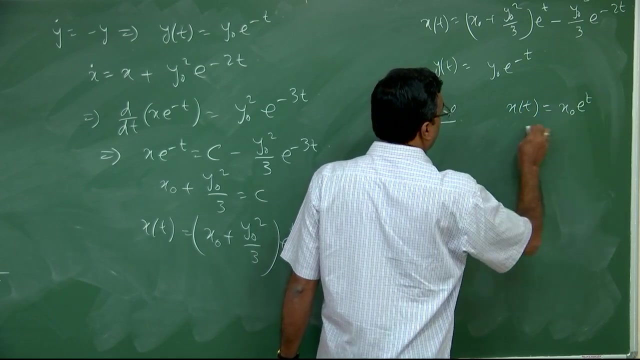 sort of trial and error method, but for this problem you can construct a Lyapunov function like this, and this is obtained from this structure by considering x star equal to 1.. So first of all you can verify number 1, that is, V 1. this is equal to 0 and V x is greater. 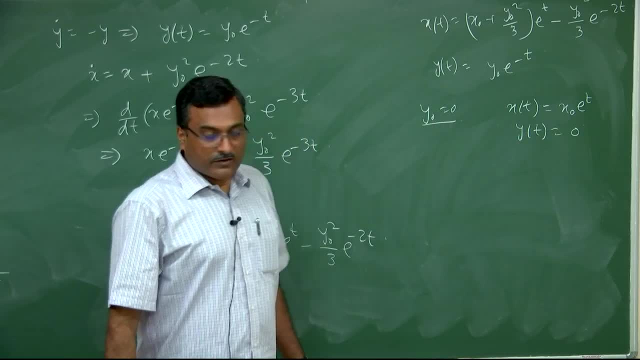 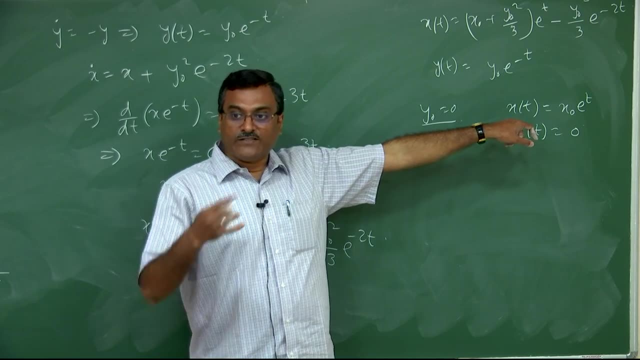 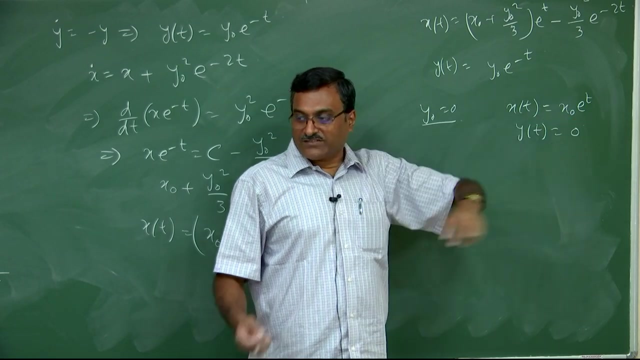 than 0, if x not equal to 1 and of course the condition x greater than 0 is satisfied. So that means within its domain. Similarly number 2: if you calculate d V d t, So d V d t, this is equal to d V d x times d x d t. So this is equal to 1 minus 1 minus 1 minus. 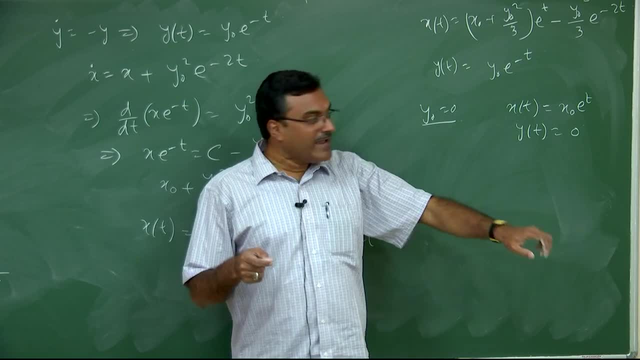 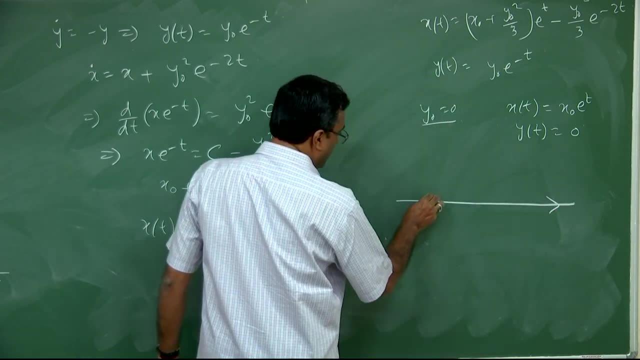 1 by x, d, x, d, t. So this is equal to x minus 1 by x into x into 1 minus x. So this is equal to minus 1 minus x, whole square, correct? Already I have mentioned x is greater than. 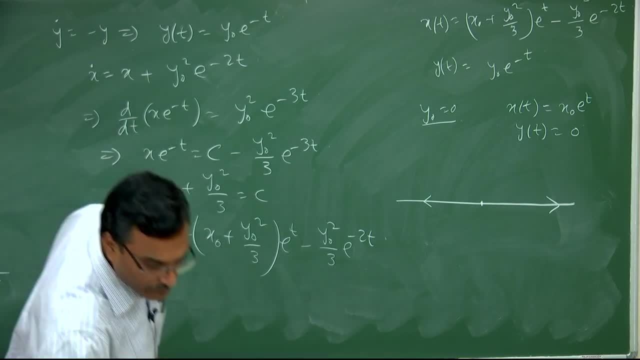 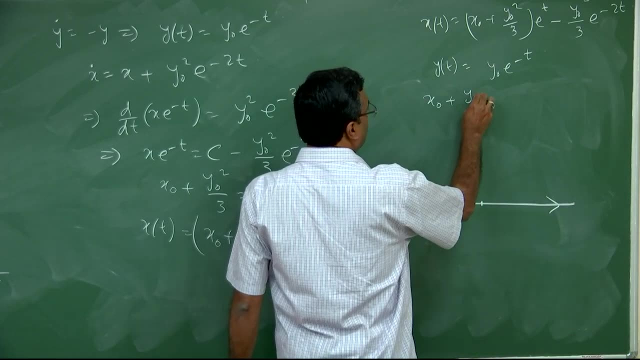 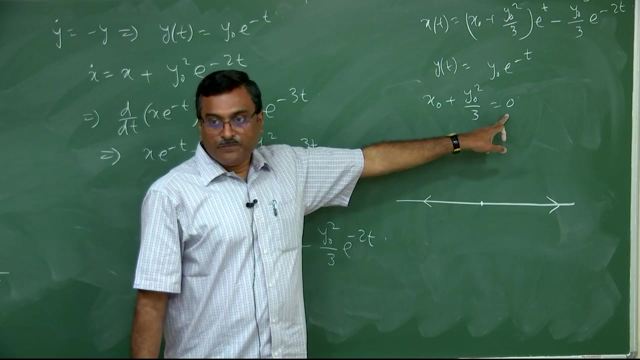 0 and then again you can verify that these two conditions are satisfied. that is, V dashed 1, this is equal to 0 and V dashed 1. this is negative definite for 1 minus 1 minus x, for x not equal to 1 and, of course, for x greater than 0, because this function does. 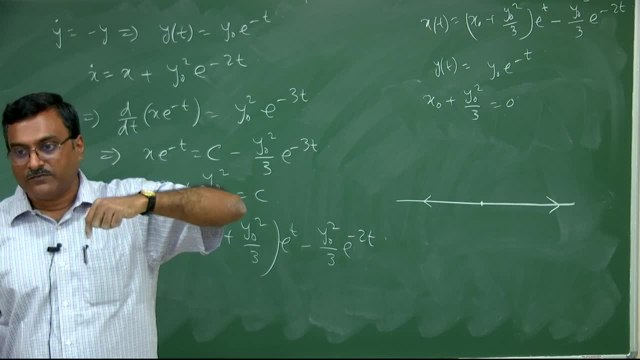 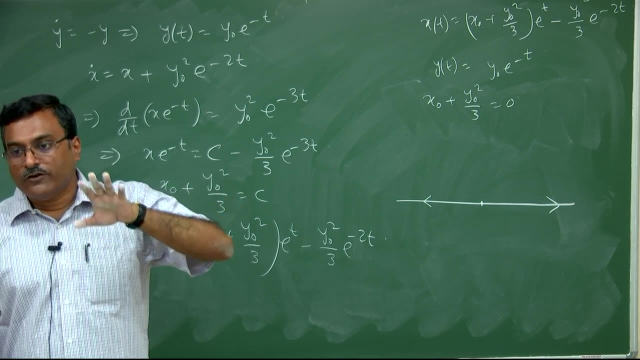 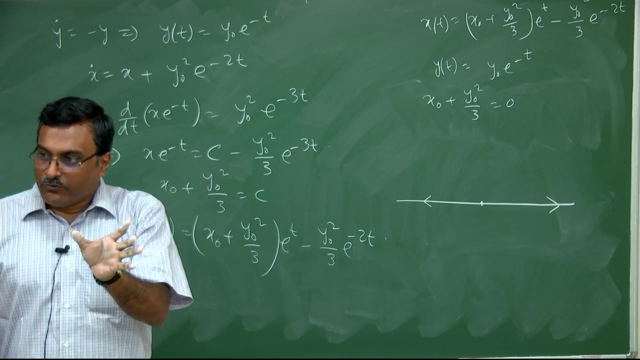 not makes any sense in terms of real variable if x less than 0, because ln is present here. So therefore both the conditions, that means, except the equilibrium point, V is a positive definite function and except at the equilibrium point the time derivative, that is, V dot x. 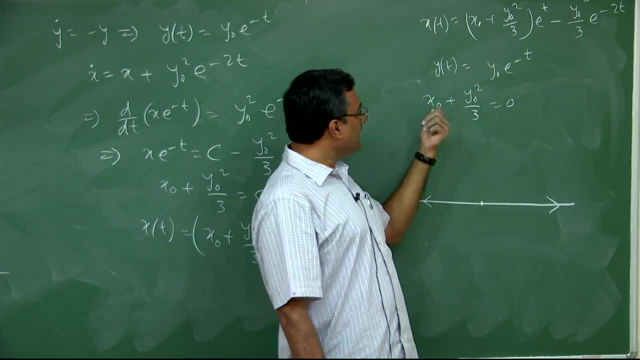 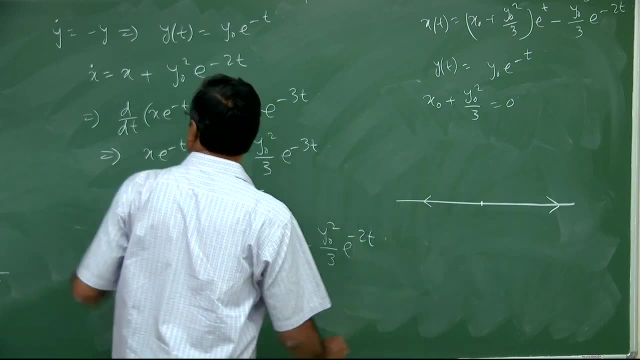 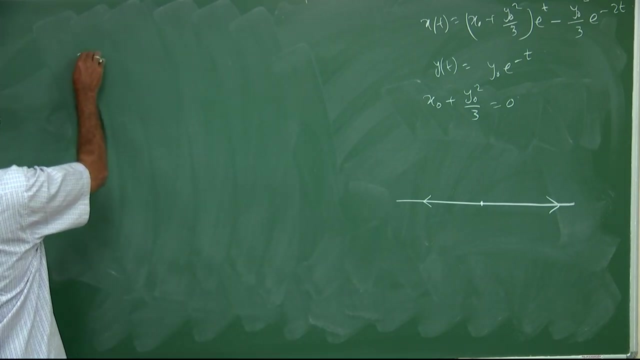 should not be 1.. V dot x is less than 0 for x not equal to 1.. So therefore it is a negative definite except at the equilibrium point. So therefore this x equal to 1 is globally asymptotically stable for this system. right, But keep in mind that there is no unified 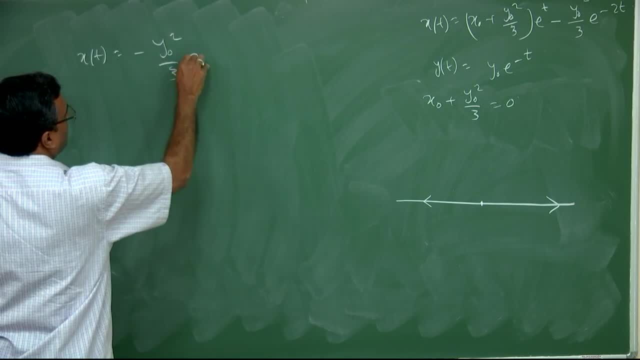 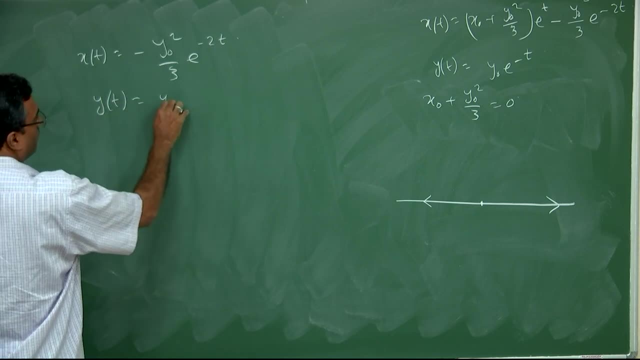 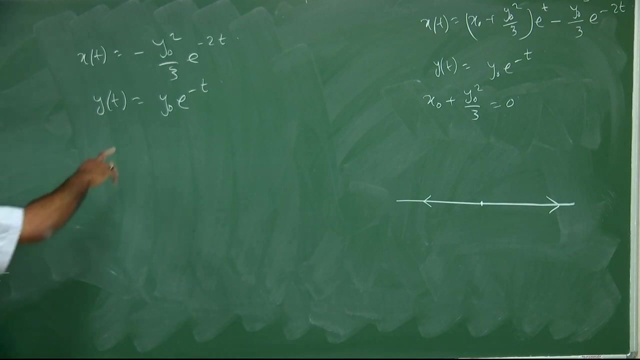 way by which you can construct either this function or some other equivalent format or applicable format for a particular problem under consideration. But there are some trial and error method and there are some different new papers or some earlier works by various people and various group of people for population dynamics model. they have come up with different. 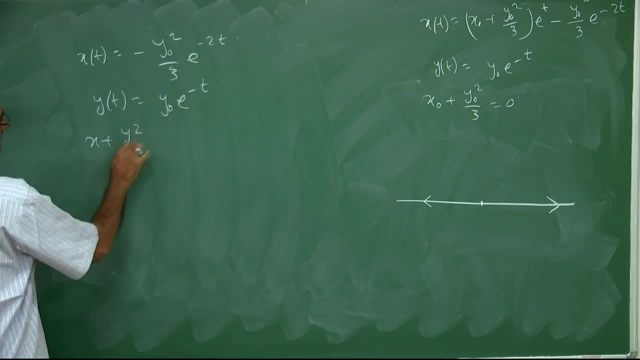 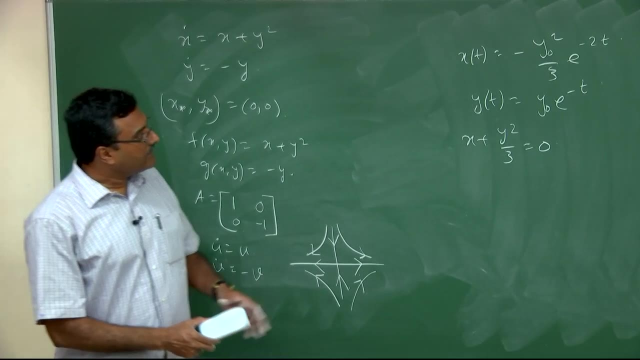 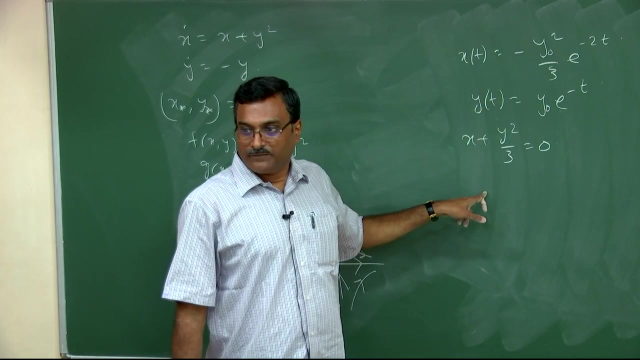 types of Lyapunov functions to prove the global stability. But the most challenging part is the construction of this kind of function. and when I will be considering the Lotka-Volterra model in two variable model, I will show you the extension of these version in order to prove that coexisting equilibrium point is globally asymptotically. 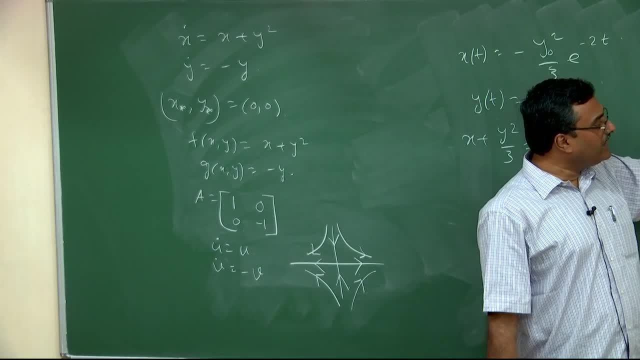 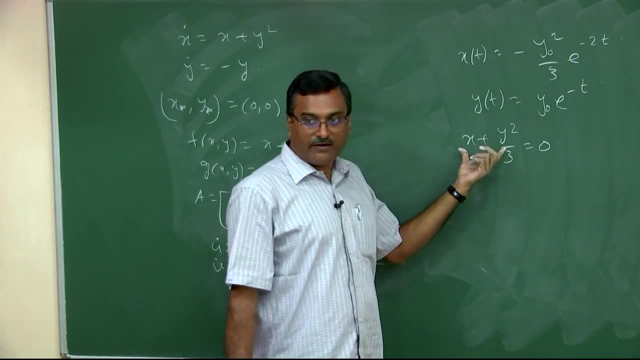 stable under certain parametric restriction, right? So for example: So for this lecture I can stop at here and just one quick question: if you have, F of x is equal to 1 minus x square and there are two local points. 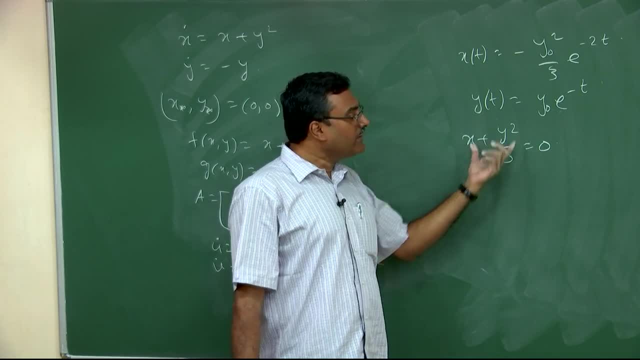 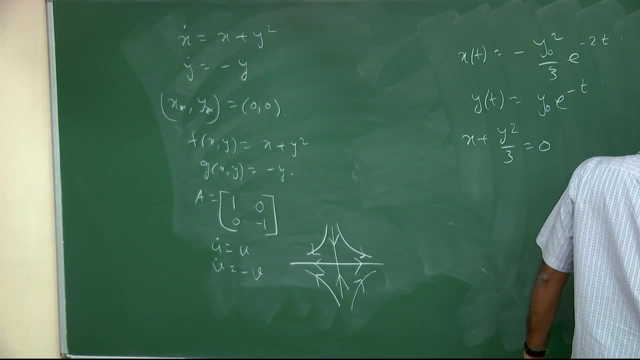 Yes, And one is comes towards the other one. is there is any bound, So in which point it will comes and which point it goes, And you are doing some small perturbation? No, in that case, actually, that is some sort of nature that, in that case, actually that. 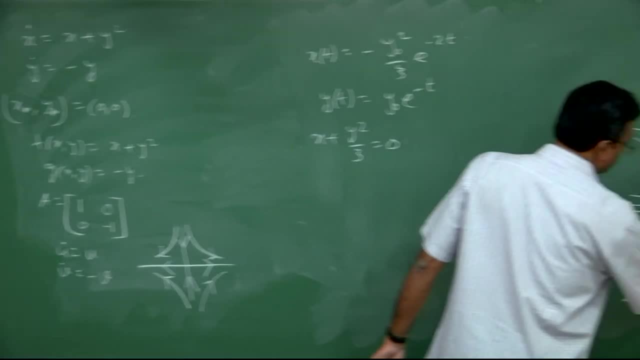 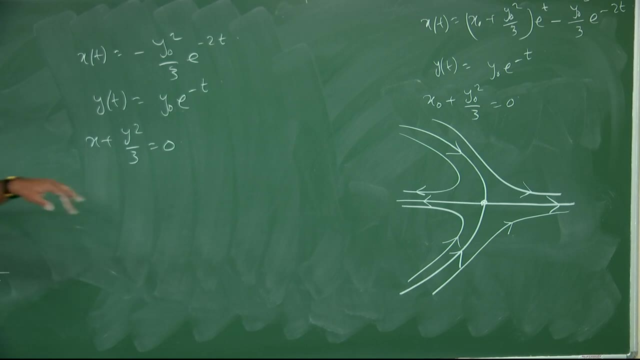 is some sort of nature- No, in that case, actually, that is some sort of nature, that, in that case, actually, that you are talking about this problem, that is, x dot equal to x square minus 1, right x dot equal to x square minus 1.. Actually, what will happen in this line, if you consider this? 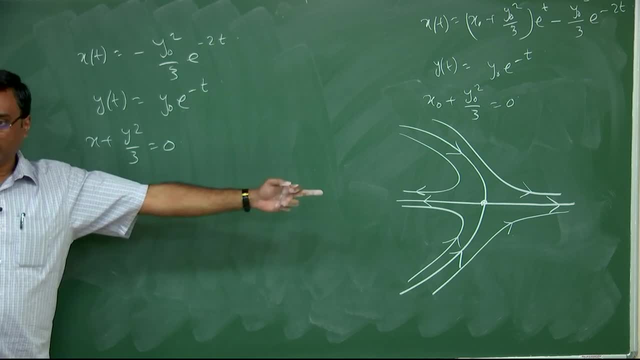 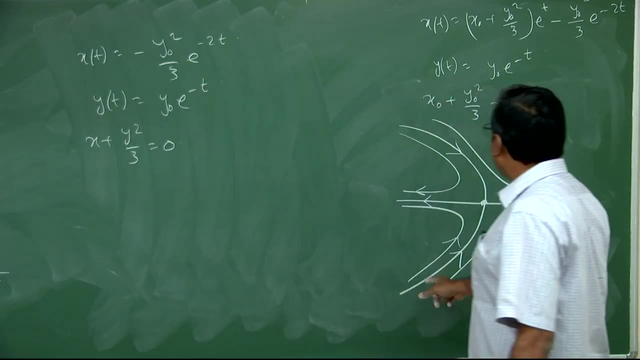 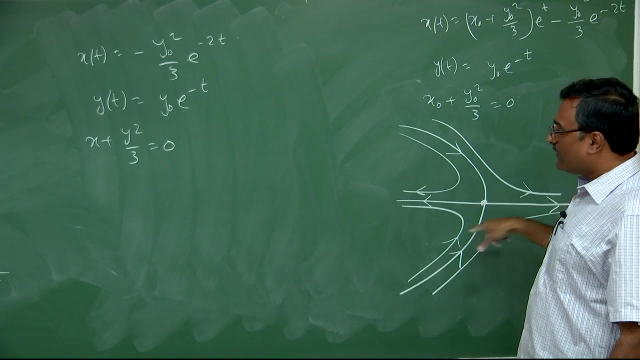 is your x 1 star equal to 1 and this is x 2 star, this is equal to minus 1.. So nature is this one for entire domain. that means minus infinity to plus infinity, because there is no other bound, But there might be some more bound if you. 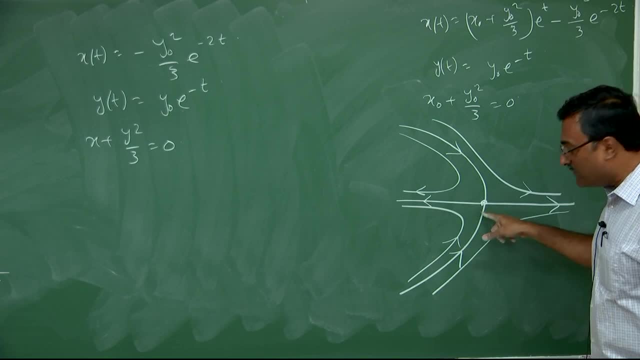 change this functional format, because in this case what you are having, you are having two equilibrium. I can give you a very simple clue by which you can construct that: one system having three equilibrium, one system having four equilibrium, and then you can change their stability property as per your own choice. How to construct that That? first of all, if 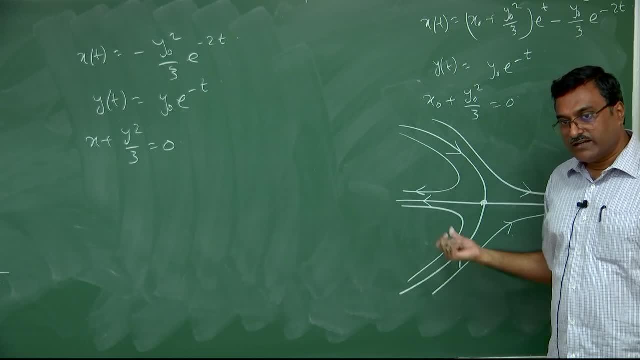 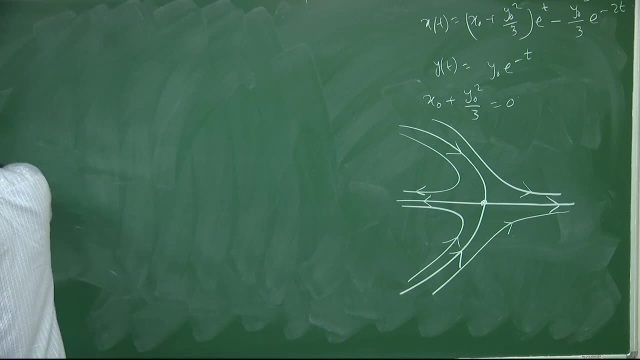 you just consider this: one x into 1 minus x, you have two equilibrium right? So you can consider x dot is equal to x into 1 minus x. either you can write x minus 2 or 2 minus x, right? So, depending upon whether x minus 2 or 2 minus x, stability property of 0 and 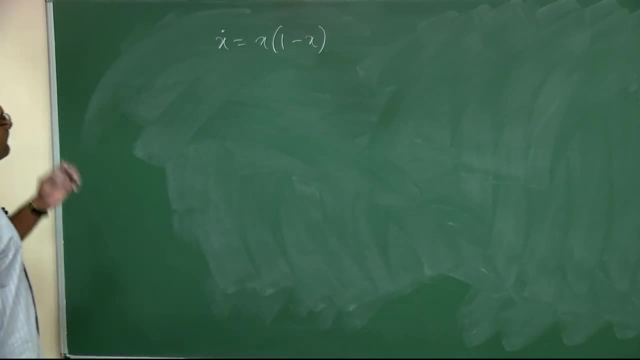 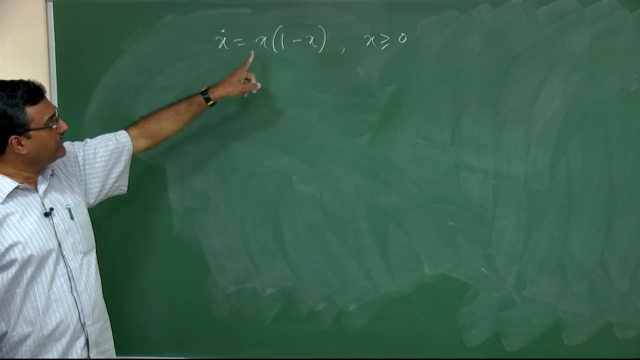 1 will be changed, but you will be having one more equilibrium point, x equal to 2, compared to this system, right? Similarly, this is nothing but your x plus 1 into x minus 1, and this stability property will be completely changed if you just introduce. 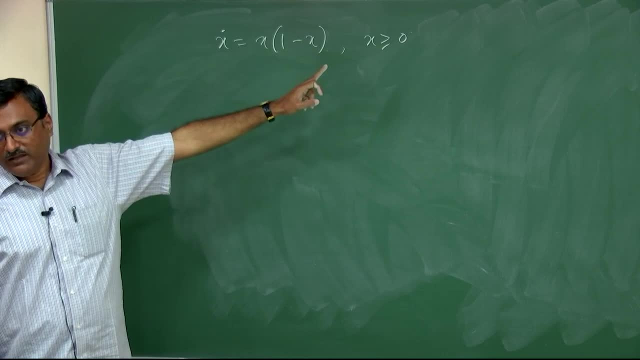 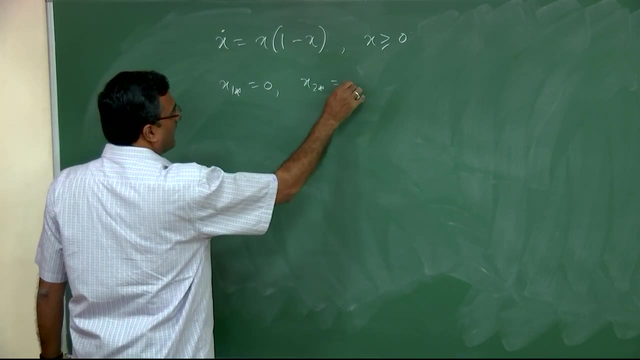 one x here. So that is x into x, square minus 1.. So if you consider x into x, square minus 1, so you have three equilibrium point, that is 1, 0 minus 1, and if you keep on doing this, 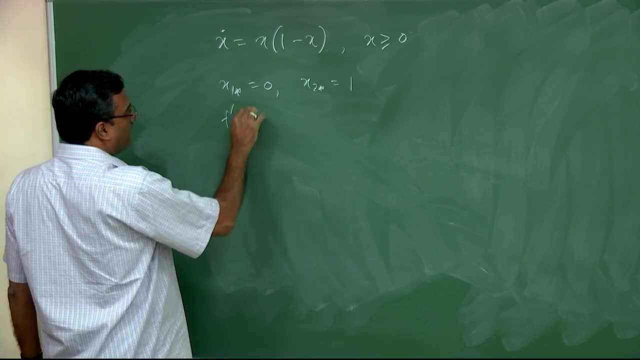 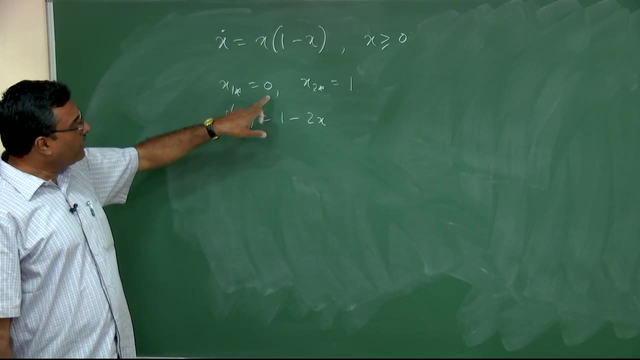 that is, 1 minus x, x minus 2, 3 minus x, x minus 4,, x minus 5, and so on. So you will be having 0, 1, 2, 3, 4, 5 as the equilibrium point and the way you are introducing either it. 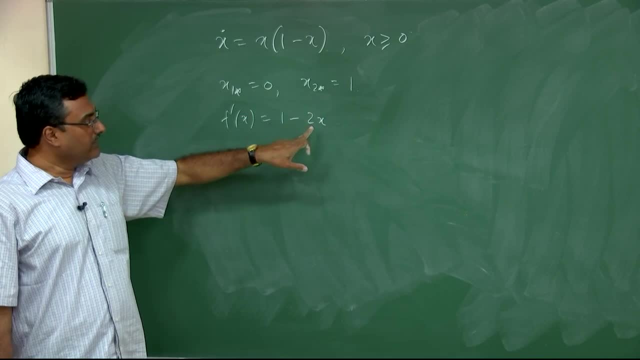 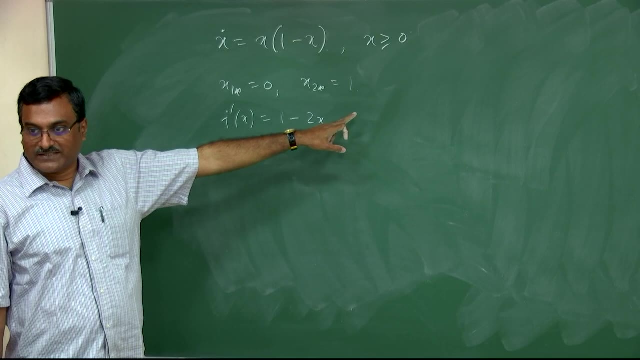 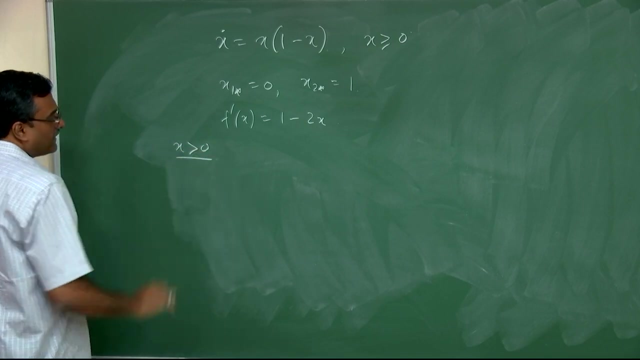 is x minus 2 or 2 minus x. So accordingly, the sign of derivative evaluated at the respective equilibrium point will be changed due to the presence of additional term which have contribution from this kind of multiplicative factor and accordingly the behavior may be changing. 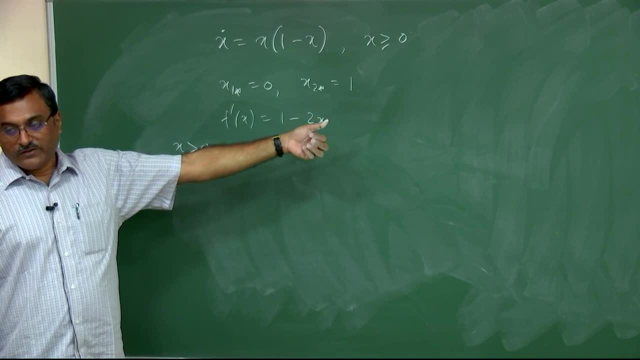 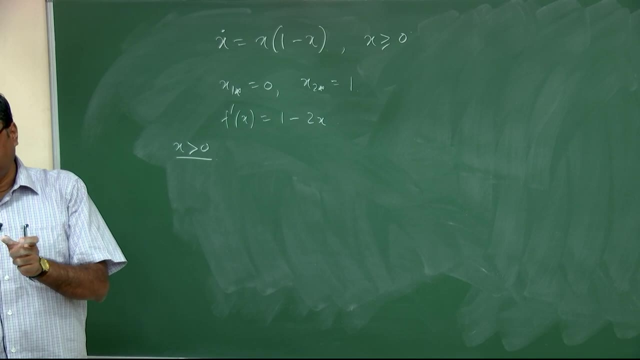 may not be changing, depending upon that how you are introducing this kind of new factor into the system. So in this case, of course, this trajectory is approaching to plus infinity. but this will not be the case. this will not be the case if you introduce one more equilibrium point here, Just for example, x square minus. 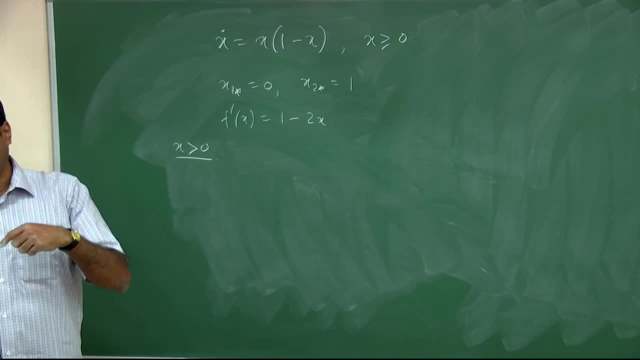 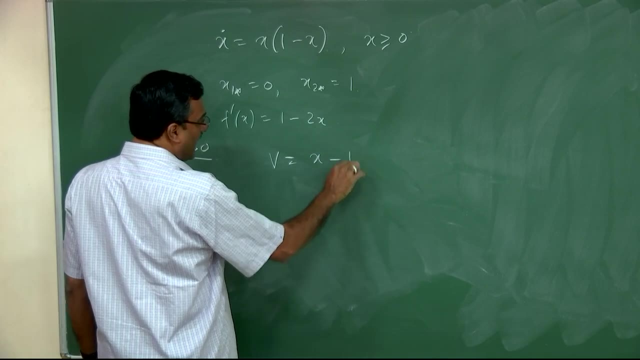 1 into you can introduce either 2 plus x or 2 minus x or x minus 2.. So there is one more equilibrium. So if your this equilibrium point is unstable still, it cannot cross x equal to 2, because x equal to 2 is a rest point. 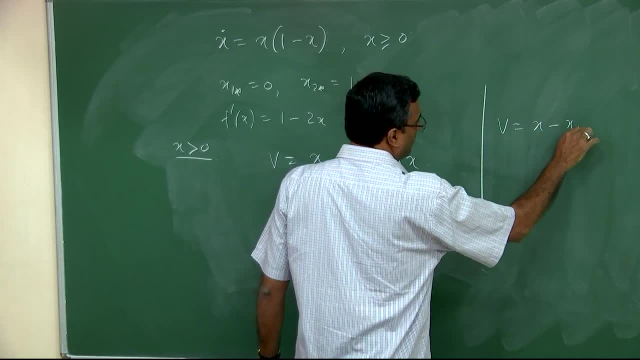 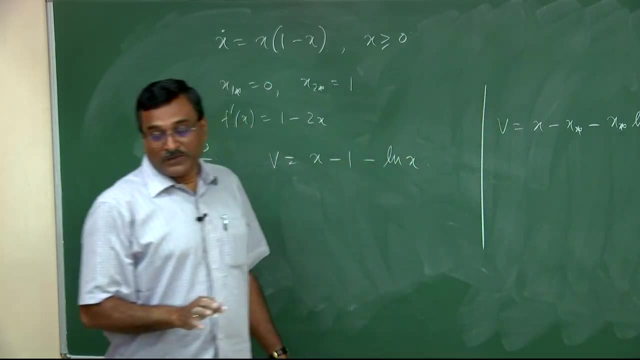 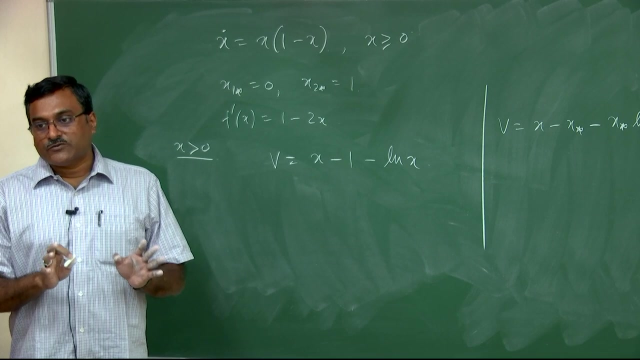 So for any system, instead of going for Eigen values, we can. the Eigen values also gives some some more and some relationship also. Yes, yes, because that I have explained in the previous example that that was the geometry, and then you can just evaluate all those derivative.